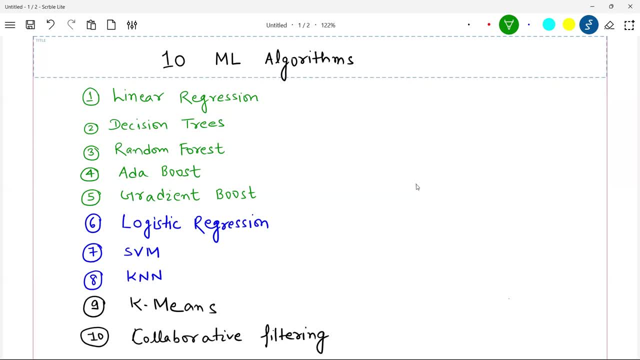 you how they work and what are their pros and cons. Okay, And as you can see, first five algorithms is in one color, Next three is in a different color and last two is in a different color. There is a reason for that, guys. I will tell you in a moment, But before that, let's try to answer. 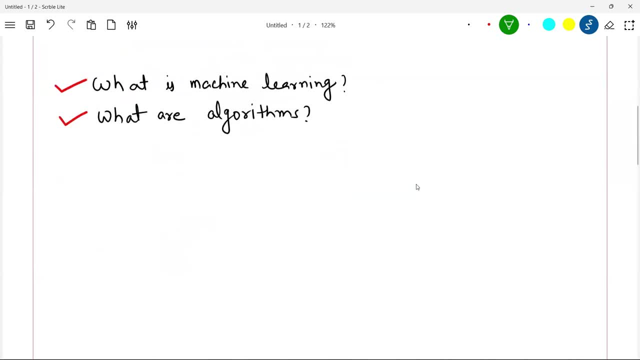 two basic questions. Okay, Let's try to answer. what is machine learning and what are algorithms? Okay, So I'll start with a non bookish definition and I will give you one simple example. Suppose you want to travel from Bangalore to Hyderabad. Okay, 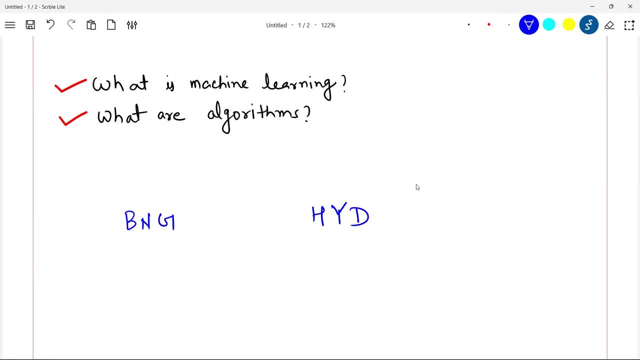 Where do you want to go? You want to go from Bangalore to Hyderabad. For this, you can either take a train, or you can either take a flight, or you can take a bus as well, or maybe you can drive your own car as well. Okay, So two things we have to understand here, guys. 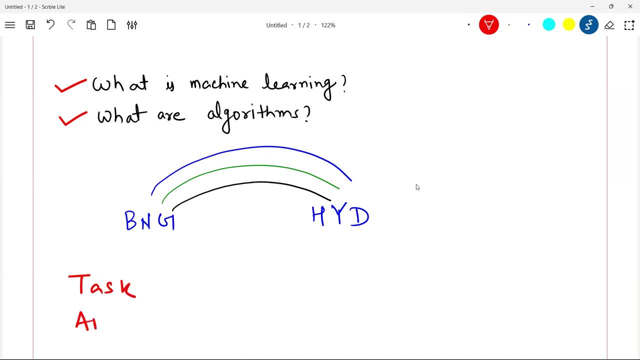 What is the task? Okay, And what is the approach? Fine, So the task in hand is: we have to go from Bangalore to Hyderabad, Okay, And the approach is all these three options that I told you just now. Now, related to the world of machine learning, in machine learning, the task: 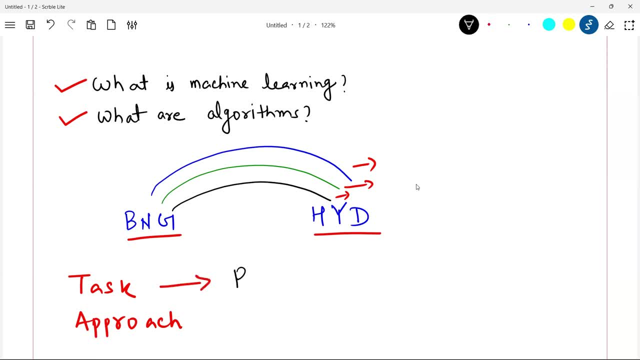 can be different kinds of tasks- Okay. For example, it can be a regression task- Okay, Or it can be a classification task- Okay, Or it can be a unsupervised learning problem. I will just write unsupervised, Okay. So in approach section we can have different approaches based. 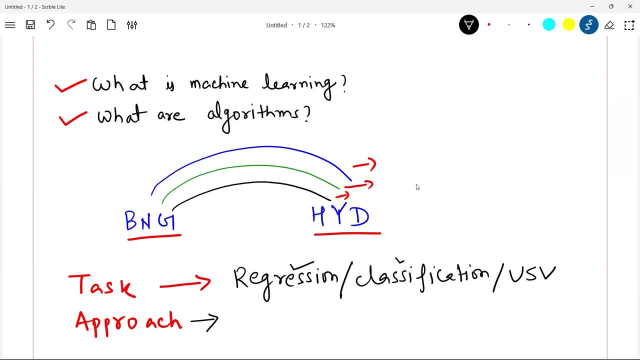 on if we are solving a regression problem or we are solving a classification or we are solving a particular case of unsupervised learning. Okay, In regression also we can take many approaches. For example, in regression there is not only one approach. In regression I can take approach one. 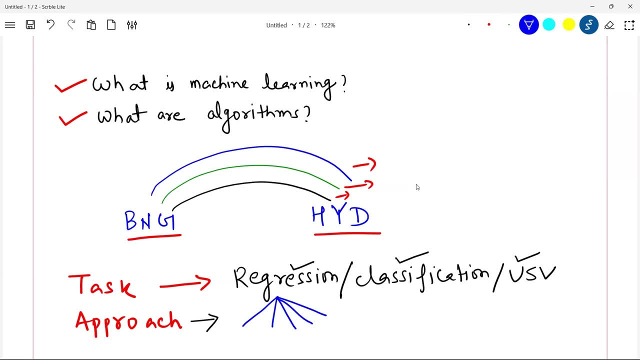 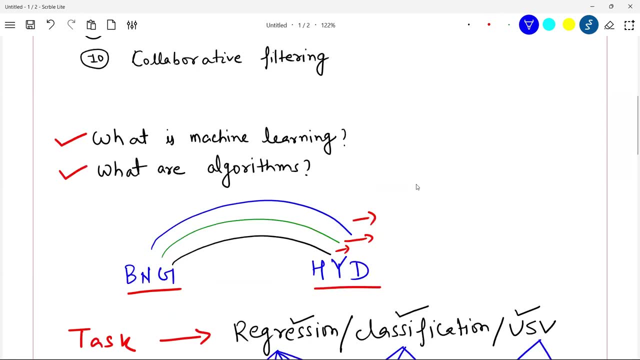 approach two: approach three: approach four: approach five: In classification I can take this approach, this approach, this approach In unsupervised. also, I can take multiple approaches, So that is why this color coding is there, The first five. 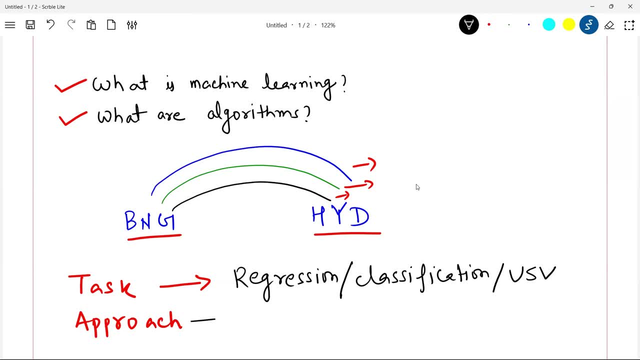 supervised. okay. so in approach section we can have different. different approaches based on if we are solving a regression problem, or we are solving a classification, or we are solving a particular case of unsupervised learning. okay, in regression also we can take many approaches. for example, in regression there is not only one approach. in regression i can take approach one. 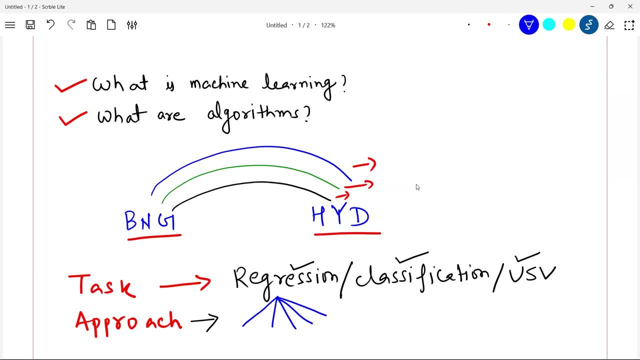 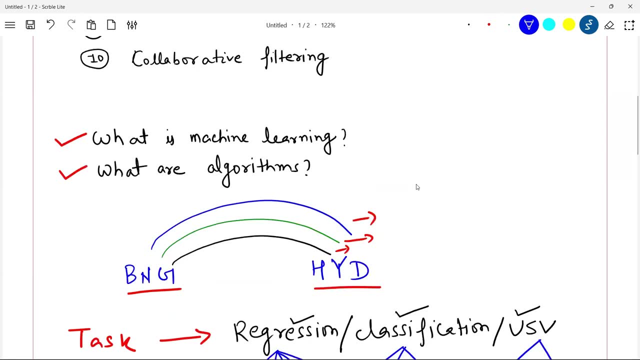 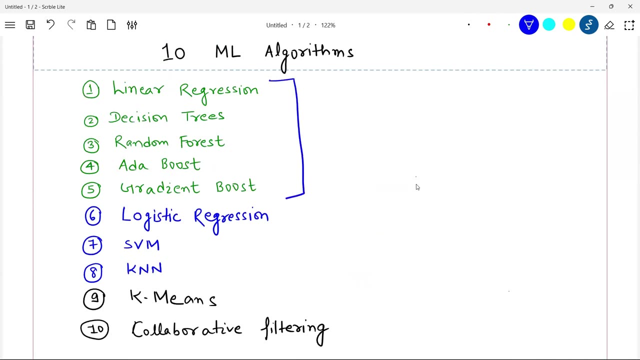 approach two. approach three, approach four, approach five: in classification, i can take this approach, this approach, this approach in unsupervised. also, i can take multiple approaches, so that is why this color coding is there. the first five algorithms that you see here will solve. i will explain you for regression use case. okay, so there we will take a regression use. 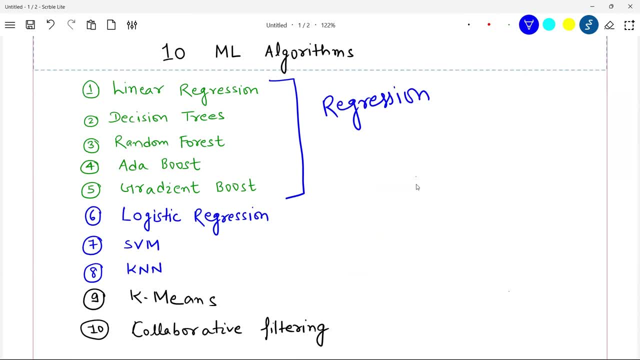 case and try to understand how to solve that using these five algorithms. okay, the next three that you see i am going to explain you with a classification use case. so these approaches are for classification problem, okay. and last two, i am going to explain you for a unsupervised learning problem: how that. 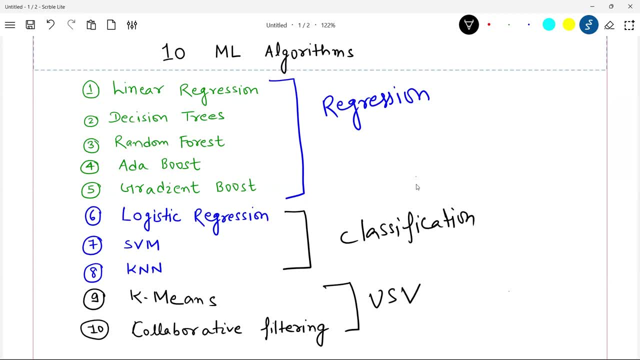 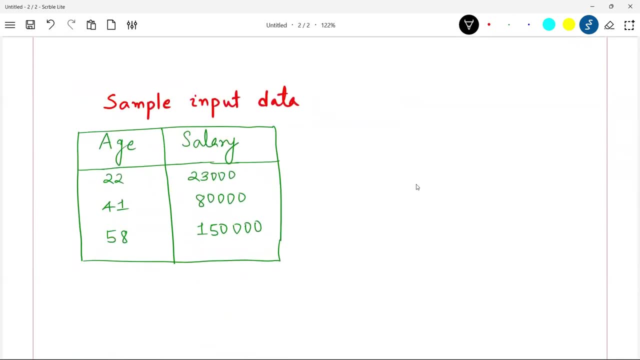 will be this: these algorithms will be used to solve a unsupervised learning problem. okay, so let's go ahead, guys, and try to understand with a simple input data. i have taken a sample input data here and let's, without any delay, start on the first algorithm, known as linear regression. 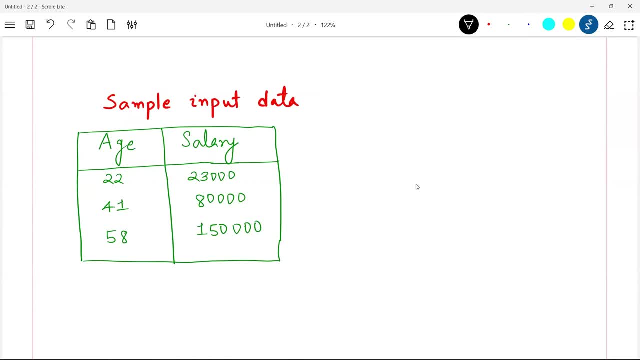 so machine learning is all about learning pattern from the data using algorithms. okay, so if we are using a algorithm known as linear regression, then what will happen? let's try to understand that. so, first algorithm of our list: linear regression. okay, now suppose this is the employee data of an. 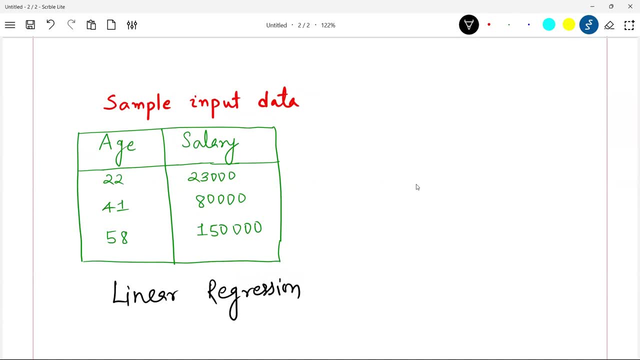 organization. you have a age column, you have a salary column- fine, so 22 years person earns 23 000, and so on and so forth. suppose we using the linear regression algorithm to solve this regression problem now, as i told you first, five problems will be regression problems. 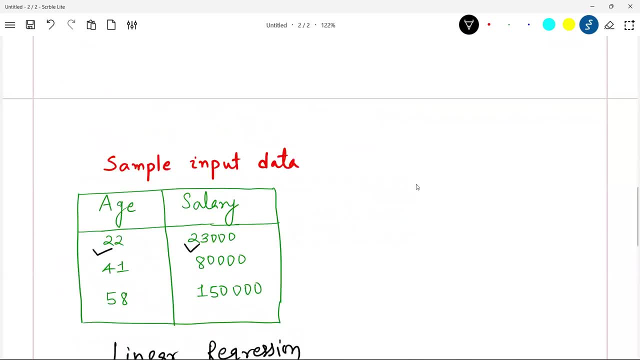 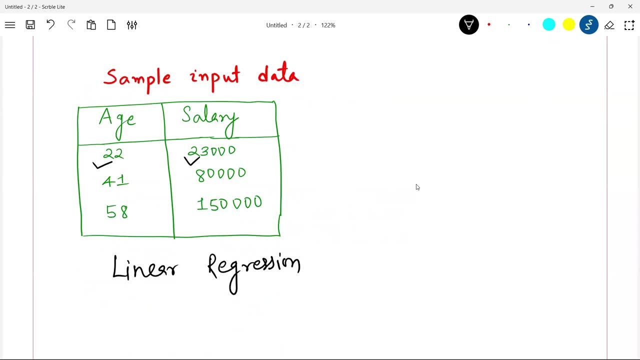 first five algorithms we will understand using regression problem. okay, come here. this is your data. so what linear regression will do is it will just take this data and it will see how the data is plotted on a xy plane like this, for example, on one axis we can take salary- okay, on y-axis and on x-axis 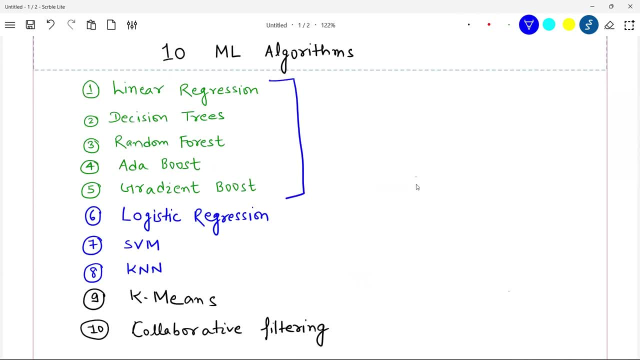 algorithms that you see here will solve, I will explain you for regression use case. Okay, So then we will take a regression use case and try to understand how to solve that using these five algorithms. Okay, The next three that you see I am going to explain you with a classification use. 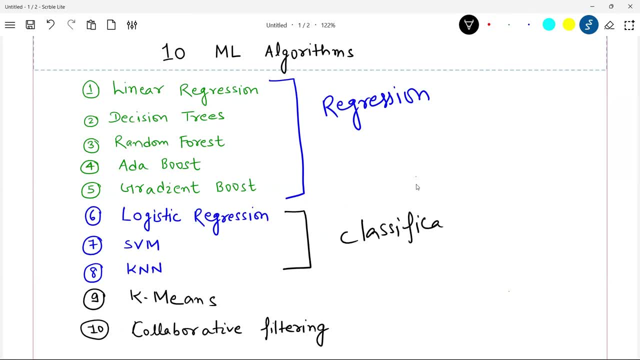 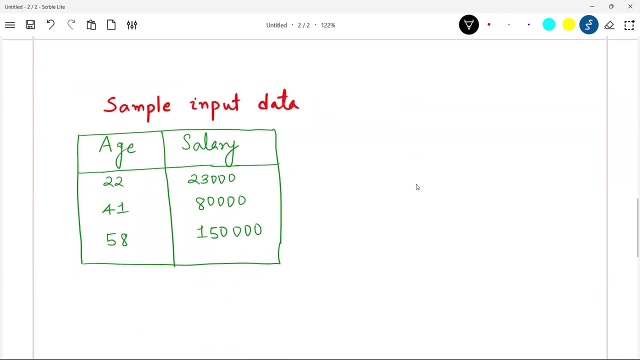 case. So these approaches are for classification problem, Okay. And last two, I am going to explain you, for an unsupervised learning problem, how that will be. These algorithms will be used to solve an unsupervised learning problem, Okay. So let's go ahead, guys, and try to understand with a simple 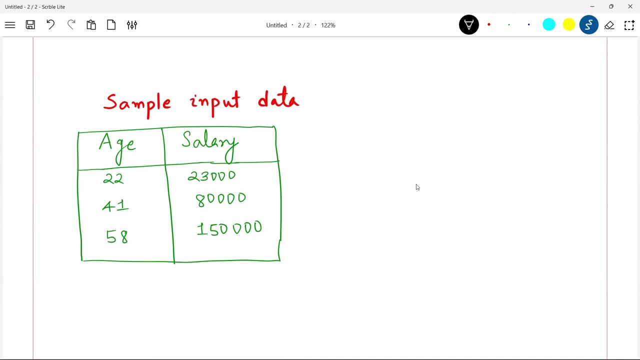 input data. I have taken a sample input data here and let's, without any delay, start on the first algorithm, known as linear regression. So machine learning is all about learning pattern from the data using algorithms. Okay, So if we are using an algorithm known as linear regression, then what? 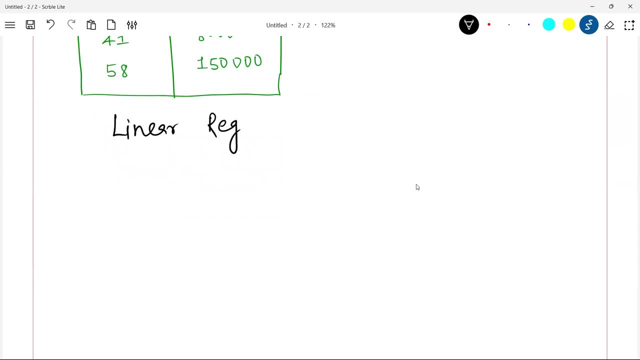 will happen. Let's try to understand that. So first algorithm of our list: linear regression. Okay, Now suppose this is the employee data of an organization. You have an age column, you have a salary column, Fine, So 22 years person earns 23,000, and so on and so forth. 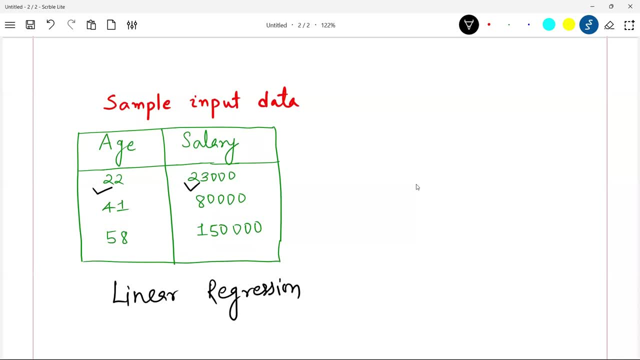 Suppose we using the linear regression approach to solve this regression problem. Now, as you can see, we are using the linear regression approach to solve this regression problem. Now, as I told you, first five problems will be regression problems. First five algorithms. we will understand. 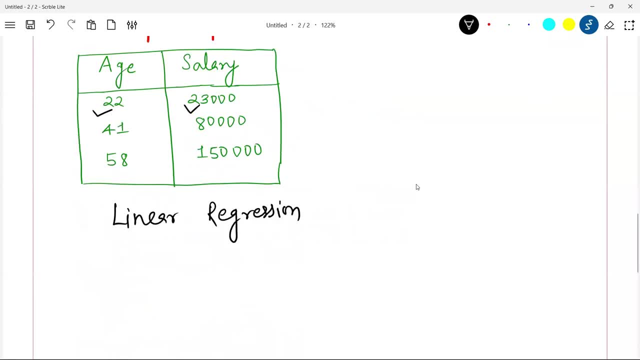 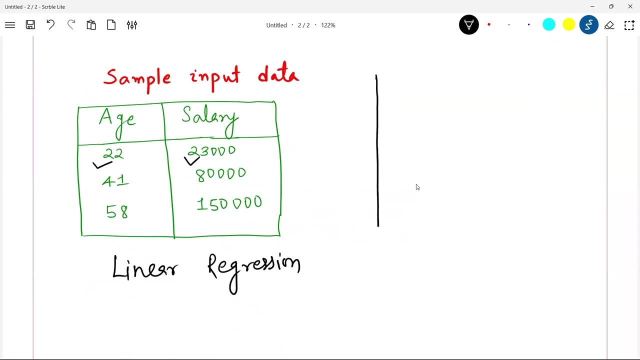 using regression problem. Okay, Come here, This is your data. So what linear regression will do is it will just take this data and it will see how the data is plotted on an X- Y plane like this, For example: on one axis we can take salary- Okay, On Y axis, and on X axis we can take age. 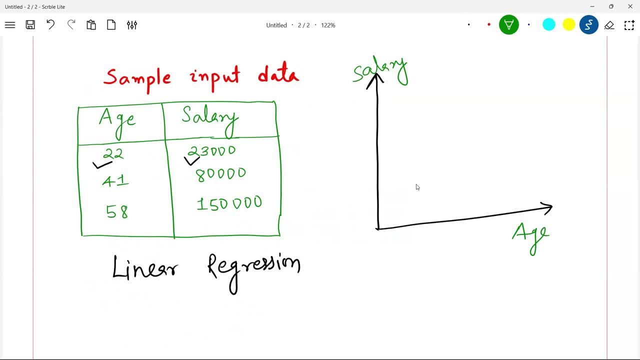 Okay, And I'm just roughly pointing these points. Okay, First point: 22 and 23,000.. Maybe it can come somewhere here on X axis If you put age on Y axis, salary I'm just putting here. Second data point can come somewhere here. 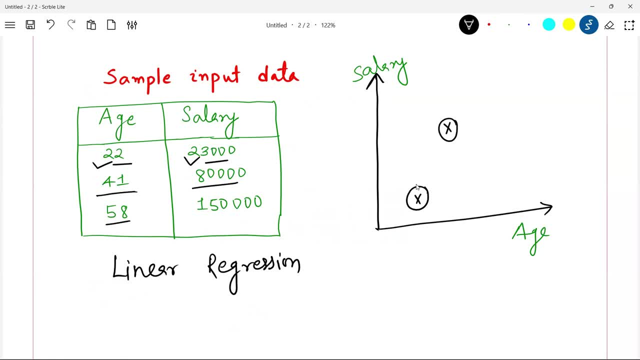 Let's say 41 and 80,000 data points and third data point 58 and 150 K. This data point can come maybe somewhere here I can say: Okay, So what linear regression will do is it will try to plot a line. 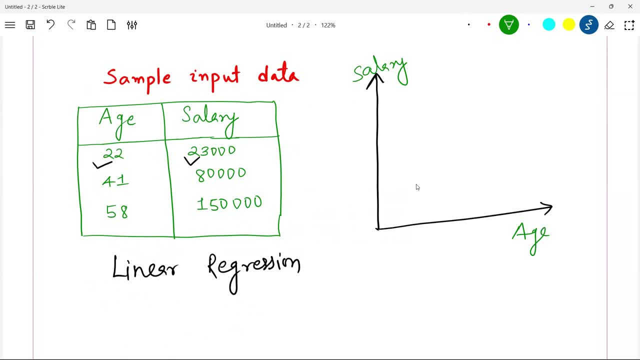 we can take age okay, and i'm just roughly pointing these points okay. first point: 22 and 23 000. maybe it can come somewhere here on x-axis if you put age on y-axis salary. i'm just putting here. second data point can come somewhere here, let's say 41 and 80 000 data points. and third data point 58 and 150k. this data 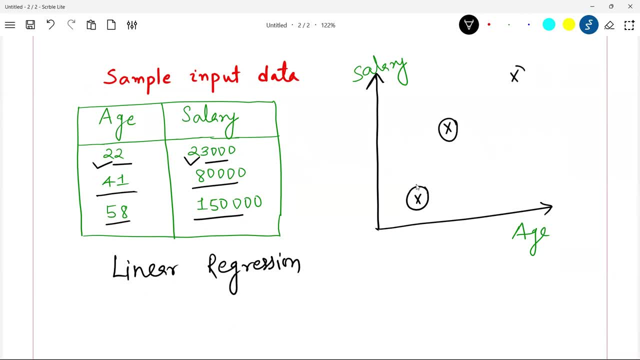 point can come maybe somewhere. here i can say: okay, so what linear regression will do is it will try to plot a line. okay, ideally, what the assumption is: all these points should fall on same line. a line like this can be plotted, or a line like this can be plotted, but the assumption here is: 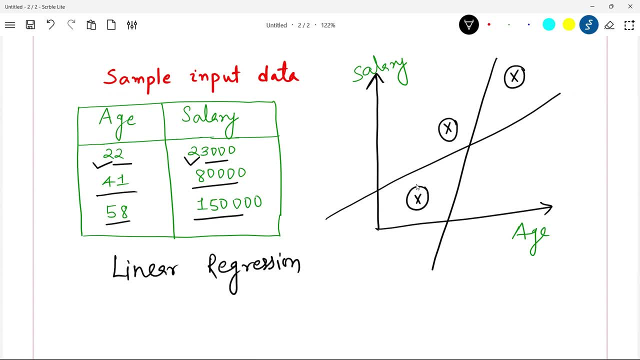 ideally, in an ideal world, all these points will fall in the same line, but it will never happen in the real world. so what logistic linear regression will do is it will try to fit something known as a best fit line. okay, so this is a best fit line, let's assume. 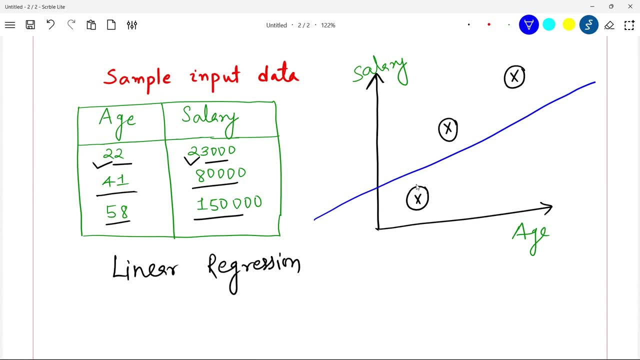 that how this best fit line is computed. it will try to minimize the distance from all these points together. so, distance from this point is this? distance from this point is this parallel to y-axis. distance from this point is this? okay, so you can call this e1. you can call this e2, you can call. 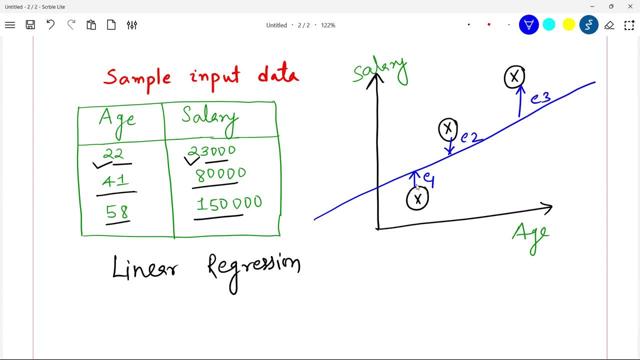 this e3. okay. so what linear regression will do is it will try to minimize e1 square plus e2 square plus e3 square. for whichever line it finds the minimum- e1 square, e2 square, e3 square- it will call that line as the model. 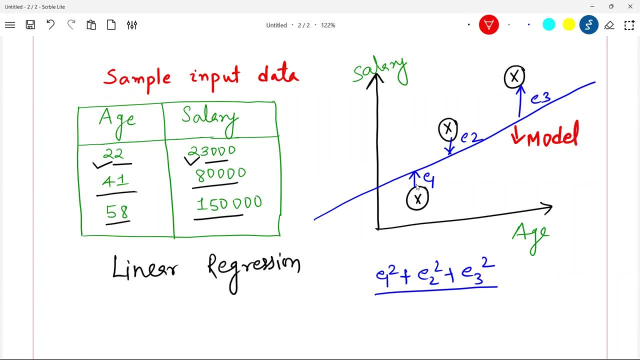 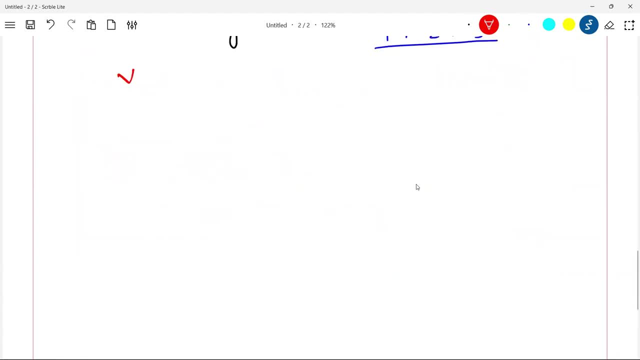 okay, it will call that line as the model. now, as you know from your normal understanding of mathematics, this straight line will have a equation in the form of mostly simplest we can write: y is equal to mx plus c. right, in our case, i can say: salary is equal to m times age, m times. 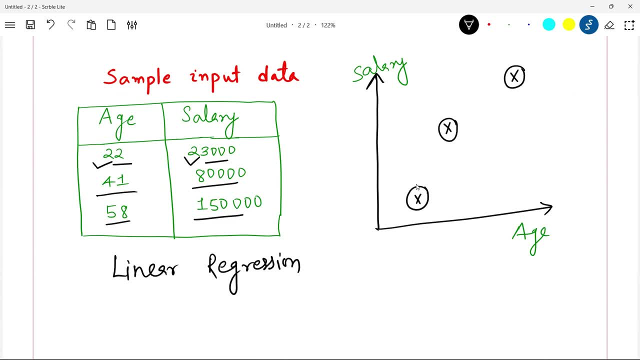 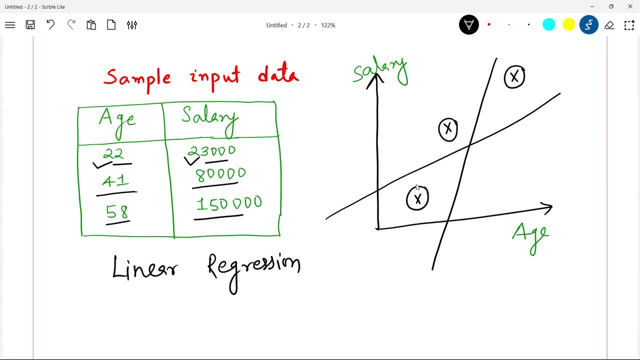 ideally, in an ideal world, all these points will fall in the same line, but it will never happen in the real world. So what logistically linear regression will do is it will try to fit something known as a best fit line. Okay, So this is a best fit line. Let's assume that. how this best fit line? 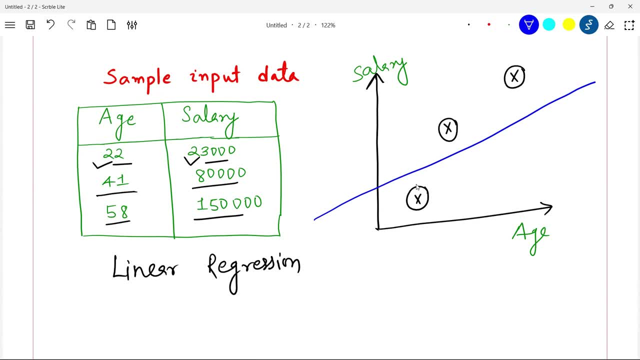 is computed. Okay, So this is a best fit line. Let's assume that. how this best fit line is computed, It will try to minimize the distance from all these points together. So distance from this point is this: Distance from this point is this parallel to y axis. 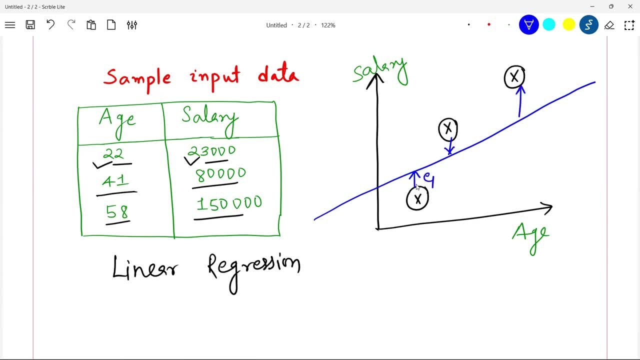 Distance from this point is this: Okay, So you can call this E1, you can call this E2, you can call this E3.. Okay, So what linear regression will do is it will try to minimize E1 square plus E2 square plus E3 square for whichever line it finds the minimum, even squared. 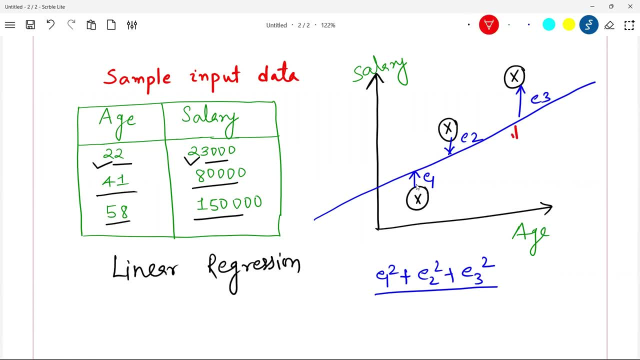 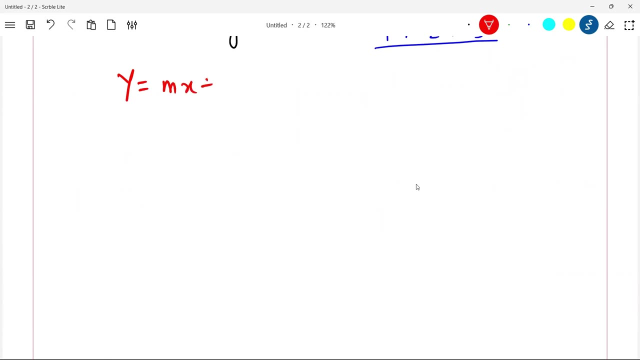 square, e2 square, e3 square. it will call that line as the model. okay, it will call that line as the model. now, as you know from your normal understanding of mathematics, this straight line will have a equation in the form of, mostly simplest we can write: y is equal to mx plus c, right in our case. 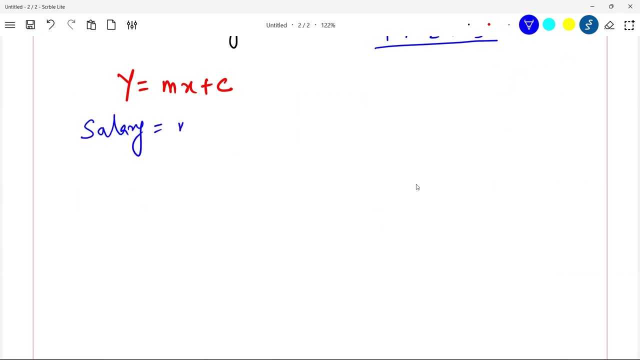 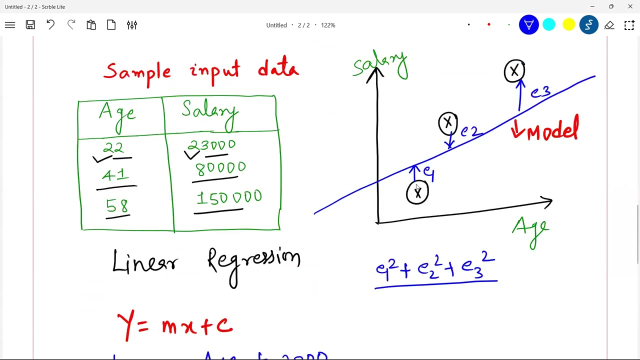 i can say: salary is equal to m times h, m times of h. this is multiplication plus c. c can be an intercept. let's give some number here, some random number. i will give, let's say, 2000. okay. so imagine this line, which is the model for linear regression, has this formula. okay. now the next question comes. 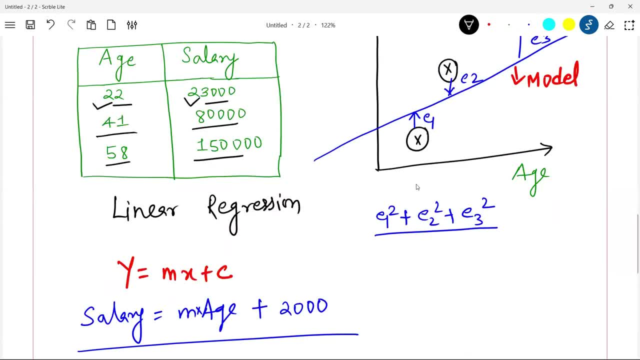 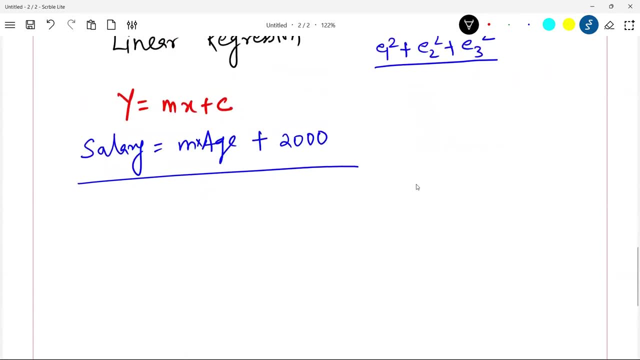 tomorrow, when the pattern has been learned and a new age comes. let's say, age is 50, so what will be the salary for that person? so very simple. the model will come here and put the numbers here. for example, if for m we can put any number, let's say 0.2, then age will be 50 and then 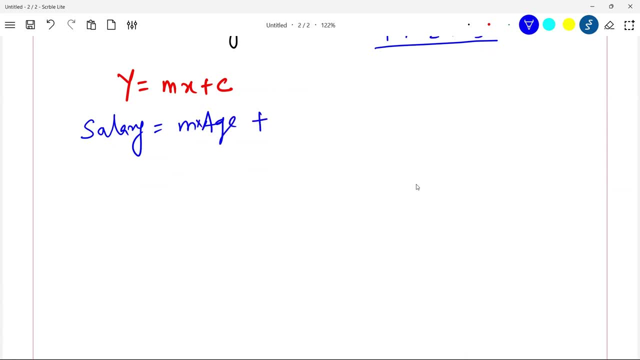 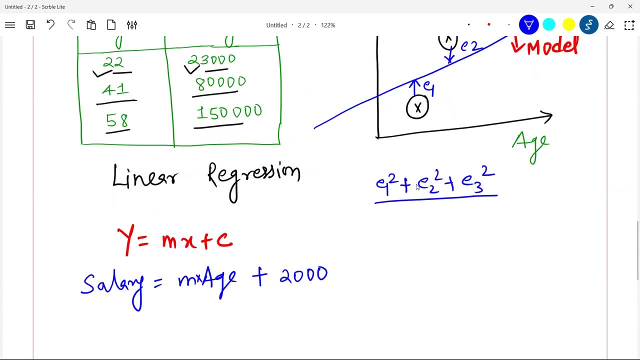 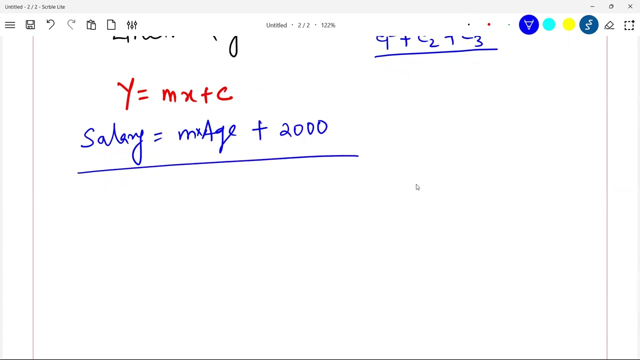 of age. this is multiplication plus c. c can be an intercept. let's give some number here, some random number. i will give, let's say, 2000. okay, so imagine this line, which is the model for linear regression, has this formula. okay, now the next question comes tomorrow, when the pattern has: 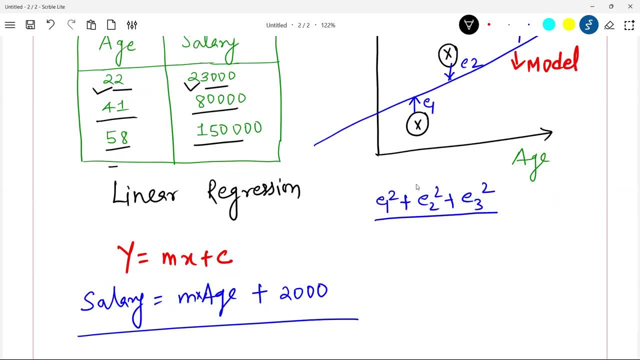 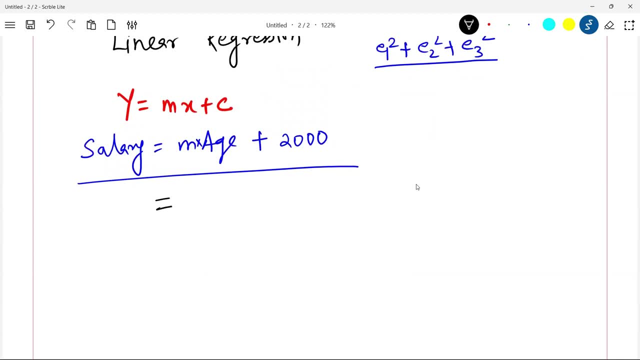 been learned and a new age comes. let's say age is 50, so what will be the salary for that person? so very simple. the model will come here and put the numbers here. for example, if for m we can put any number, let's say 0.2, then age will be 50 and then salary will be intercept will be 2000. whatever this calculation, 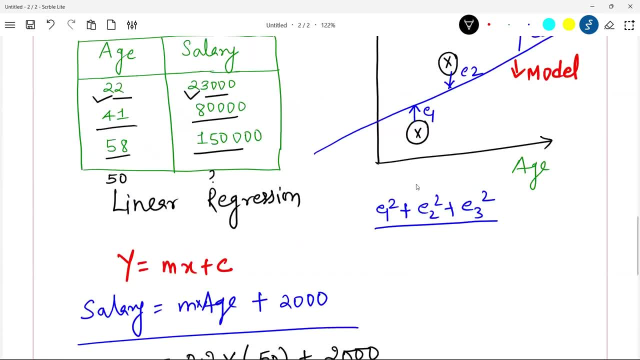 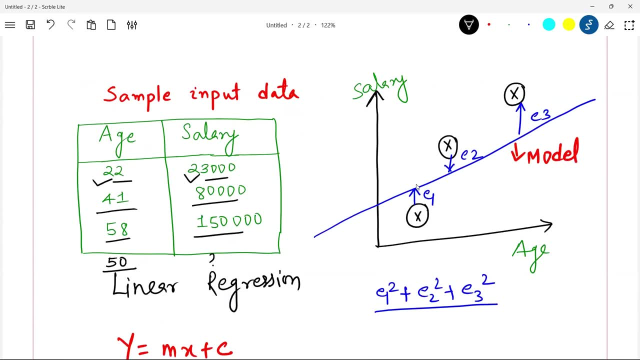 comes, that will be the prediction of the salary for this 50. okay, very simple, very simple mathematical model. the assumption is there is a linear relation between independent variable and target variable. okay, that's the assumption. so what it will do? it will try to plot a line, what it will call as a best fit line. 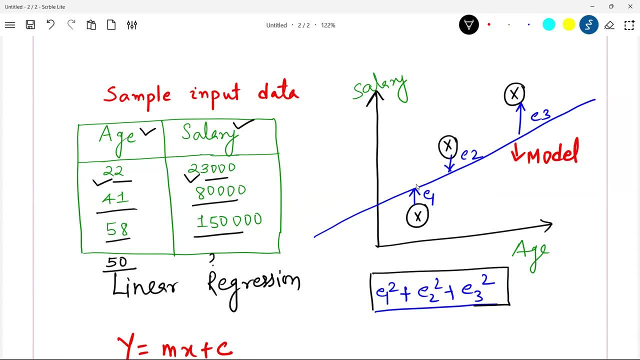 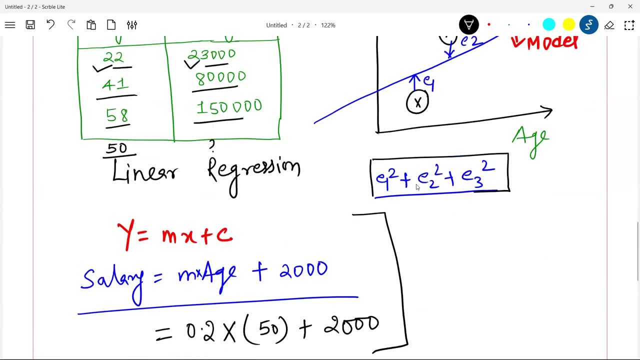 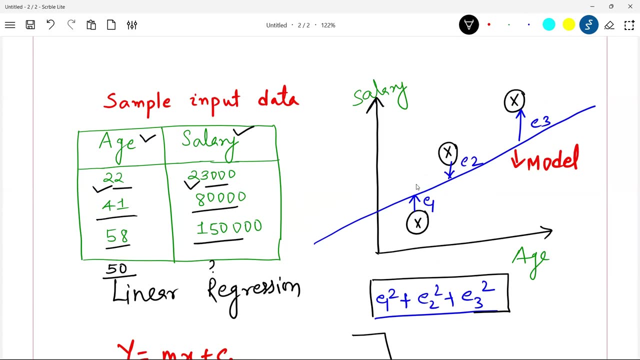 wherever it finds this value as minimum, once the best fit line comes. then how the prediction happens like this: okay, obviously there will be pros and cons of all the algorithms, all the models. so what is the pros and cons of linear regression? the? the pluses or pros for this model will be it's. 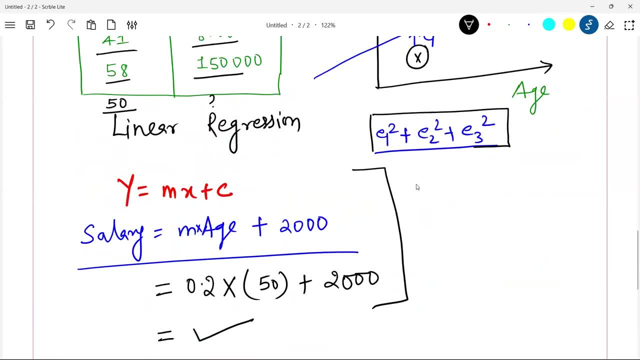 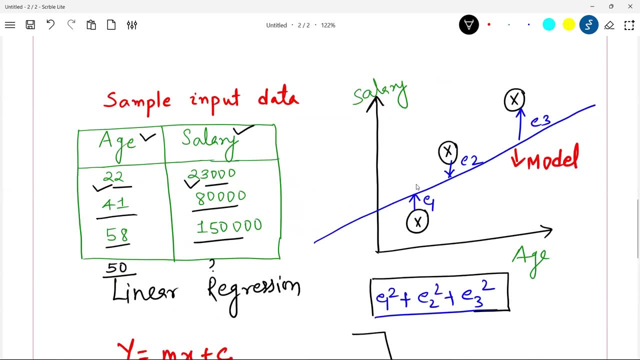 a simple to understand model. it's a mathematical model. you can explain to someone, but the cons will be. it's not a mathematical model. it's a mathematical model. it's a mathematical model, not necessary that your data will always be this simple. that can be fit in a line right or close to. 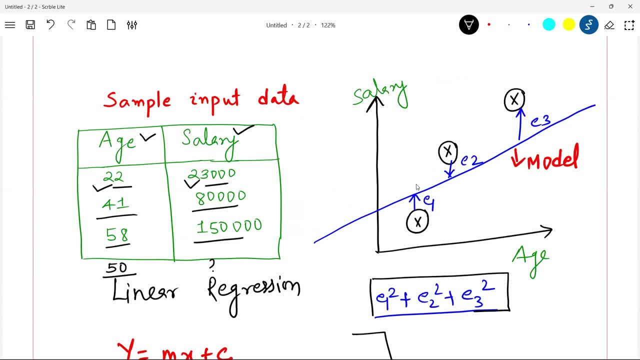 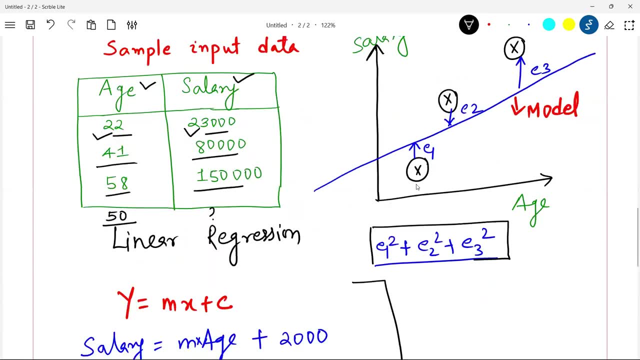 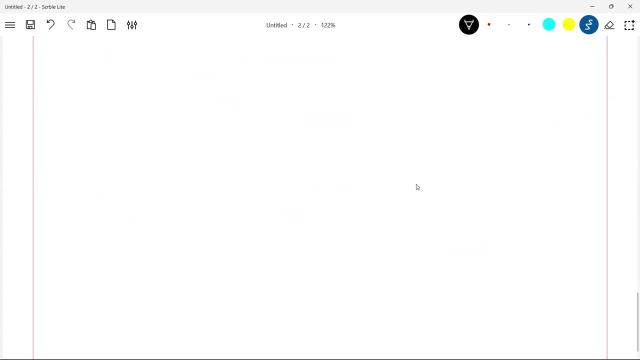 a line, so it's a simple model, hence lot of real world problems it may be difficult to solve with simple linear regression. there can be a varieties in linear regression that i have created videos. you can watch those videos, but simply linear regression works like this. okay, this is one. 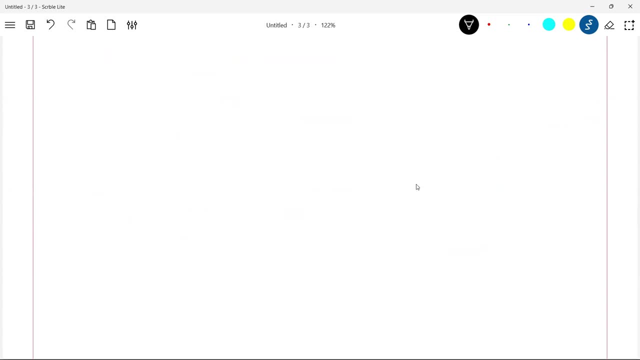 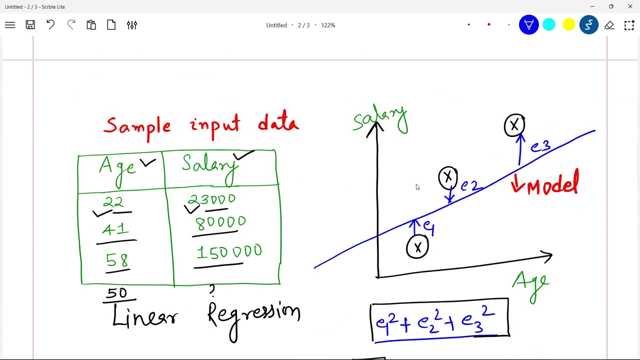 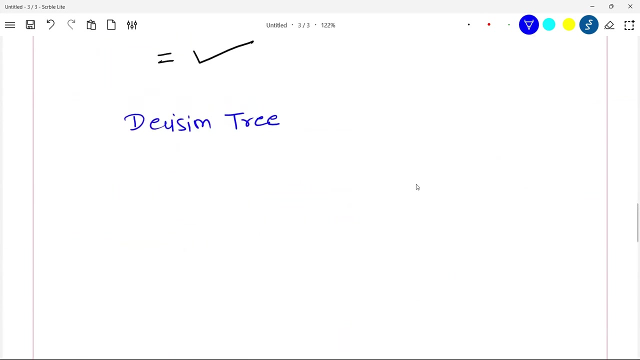 first approach. first approach means first algorithm. now let's go ahead and try to see how decision tree will approach the same problem. okay, how decision tree will approach the same problem. so if you give this same data, okay, if you give the same data to decision tree and you ask, hey, learn pattern from this data, what decision tree will do is it will just try to break. 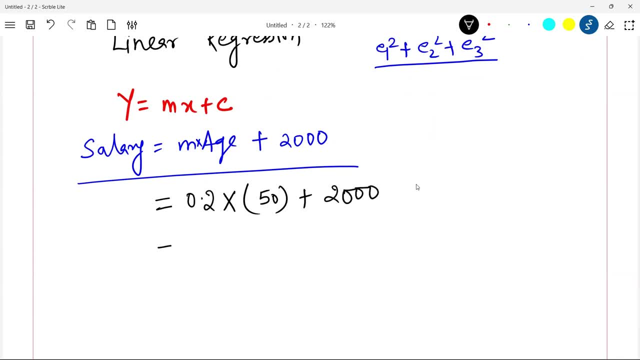 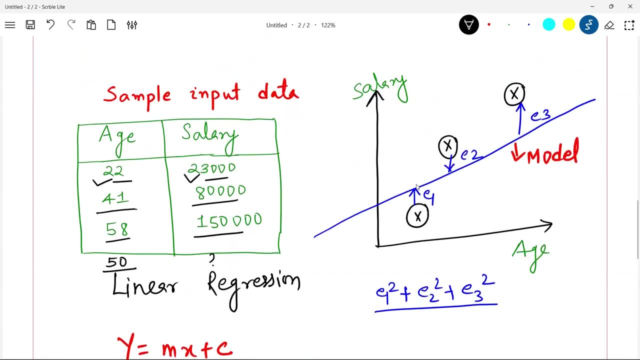 salary will be intercept will be 2000. whatever this calculation comes, that will be the prediction of the salary for this 50. okay, very simple, very simple mathematical model. the assumption is there is a linear relation between independent variable and target variable. okay, that's the assumption. so what it will do? it will try to plot a line, what it will call as a best fit line. 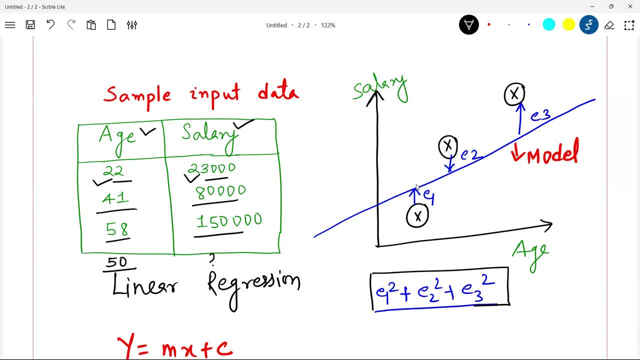 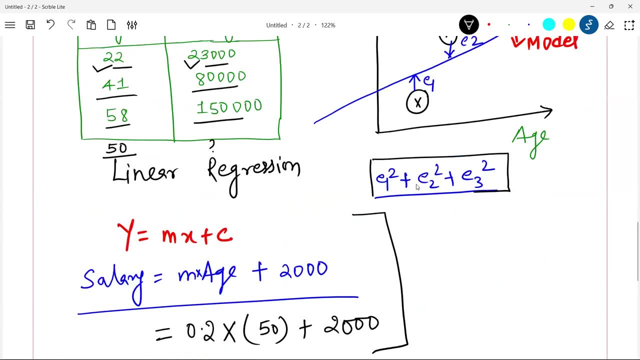 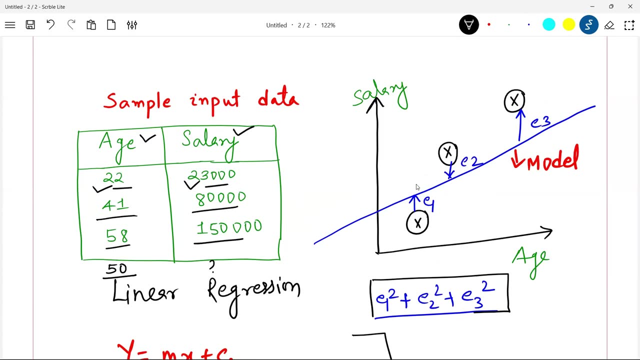 wherever it finds this value as minimum, once the best fit line comes. then how the prediction happens like this: okay, obviously there will be pros and cons of all the algorithms, all the models. so what is the pros and cons of linear regression? the, the pluses or pros for this model will be. it's a simple. 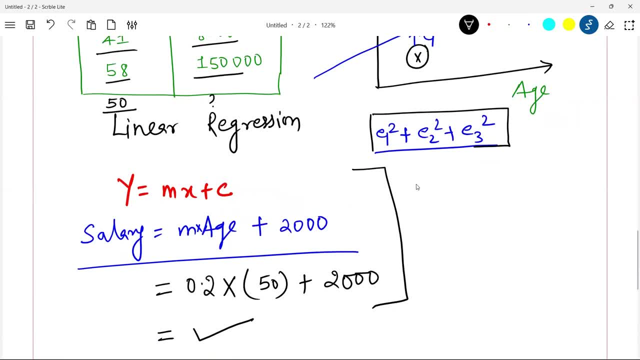 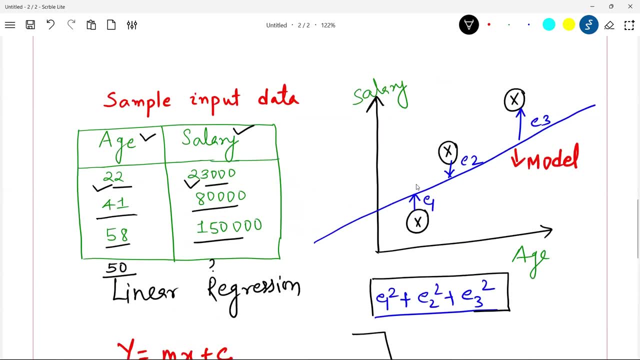 to understand model. it's a mathematical model. you can explain to someone, but the cons will be. it's not necessary that your data will always be this simple. that can be fit in a line right or close to a line. so it's a simple model, hence lot of real world problems. it may be difficult. 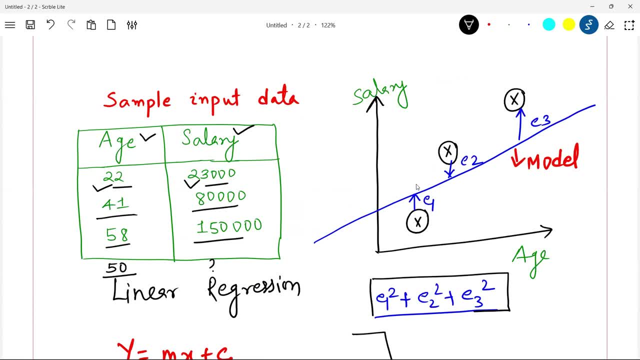 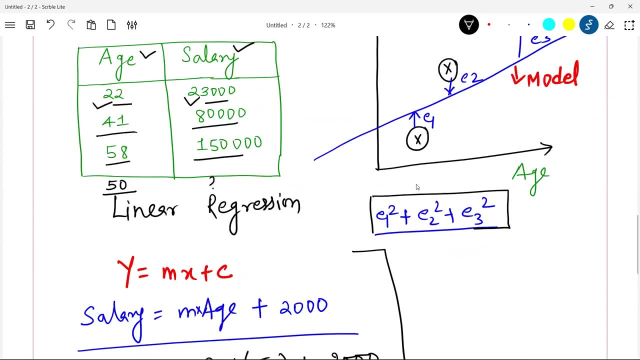 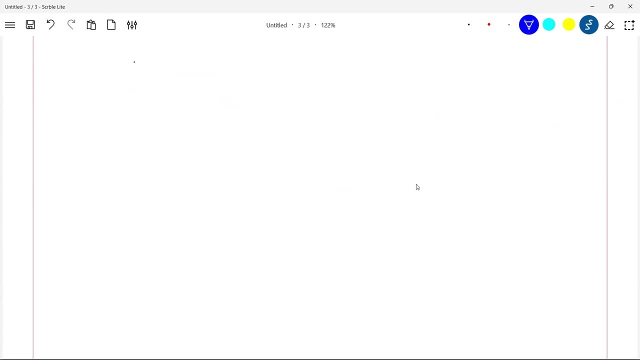 to solve with simple linear regression. there can be a varieties in linear regression that i have created videos. you can watch those videos, but simply linear regression works like this. okay, so first approach. first approach means first algorithm. now let's go ahead and try to see how decision tree will approach the same problem. okay, how decision tree will approach the same problem. 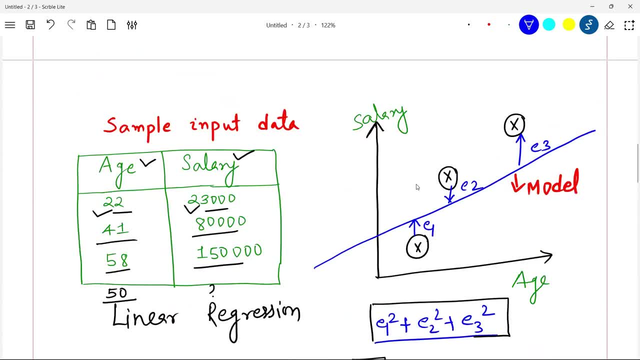 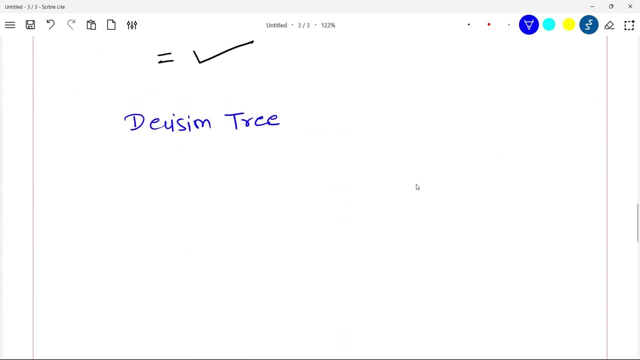 so if you give this same data, okay, if you give the same data to decision tree and you ask, hey, learn pattern from this data- what decision tree will do is it will just try to break the data. how it will break the data is it will create a rule like this: okay, so 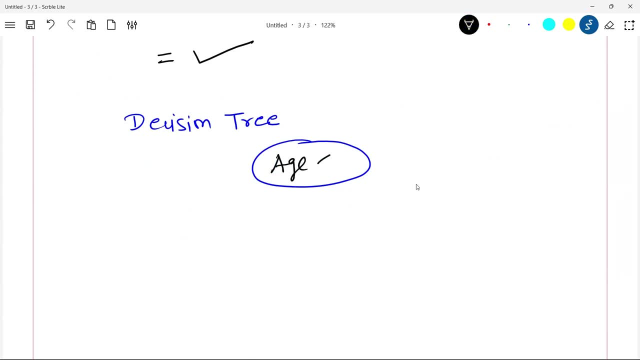 I can write a rule here. for example, I can say: age less than equals to 30. this is a rule, okay, so some records will satisfy this rule. okay, some records will satisfy and some records will not satisfy. this way, data will break. okay, if you come here. age less than 30, how many records? only one. 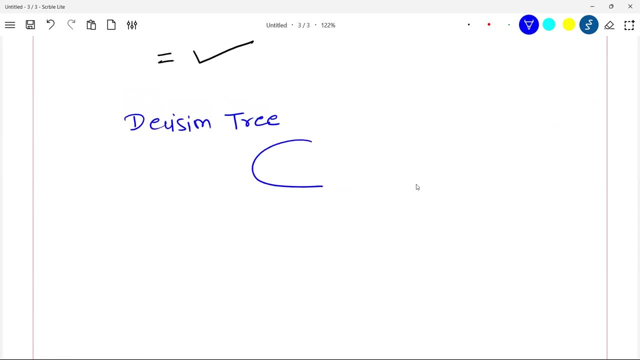 the data. how it will break the data is it will create a rule like this. okay, so i can write a rule here. for example, i can say: is less than equals to 30. this is a rule that i can write a rule. okay, so some records will satisfy this rule. okay, some records will satisfy and some. 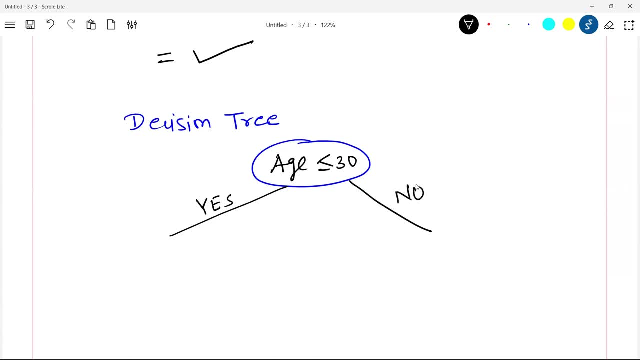 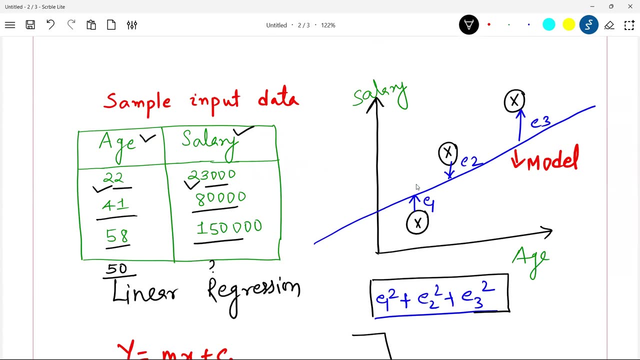 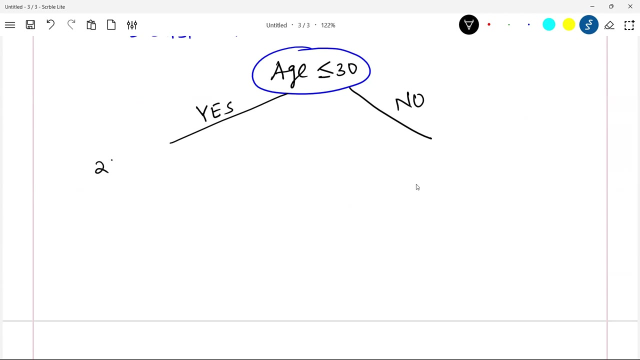 records will not satisfy. this way, data will break. okay, if you come here is less than 30, how many records? only one record is more than 30. two records. so how many records will come this side? only one record will come. okay, so let's say that record is- i should not write the wrong numbers- 22. 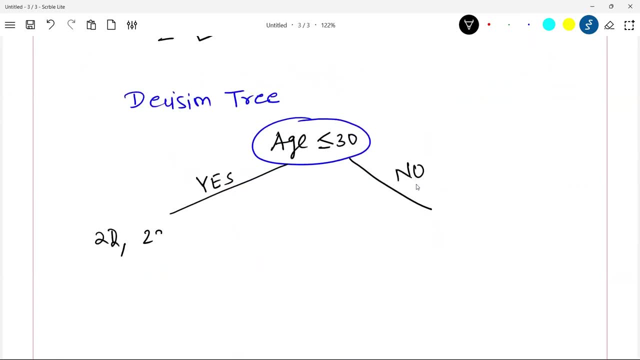 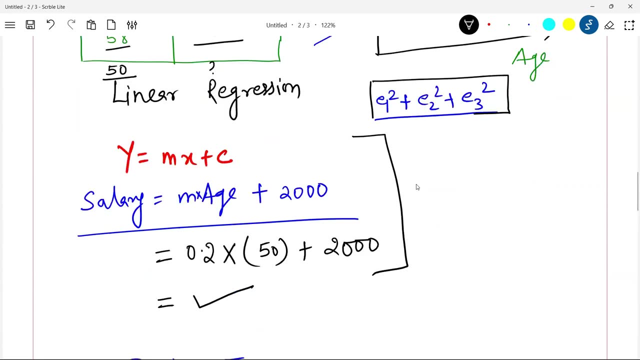 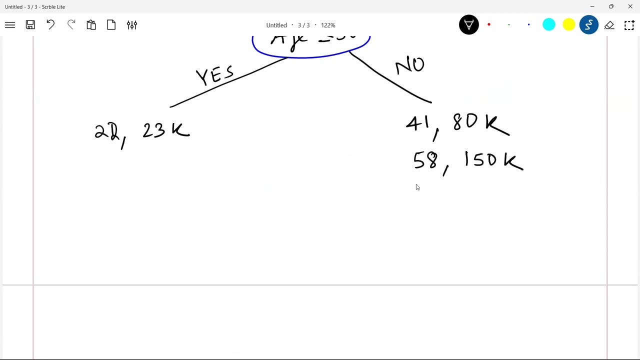 so i will write here 22 and 23 k and here i will write 41 and 80 k. okay, and there is one more record. let me take the numbers 58 and 150 k. 58 and 150 k. understand this carefully, guys, because for next. 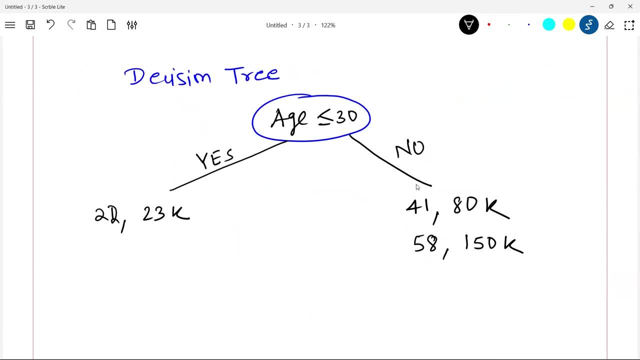 next algorithms. this is the base. okay, so decision tree will split your data like this. so you had total: how many records in the beginning? three records here. how many records you are having one record here. how many records you are having one record here. how many records you are having one. 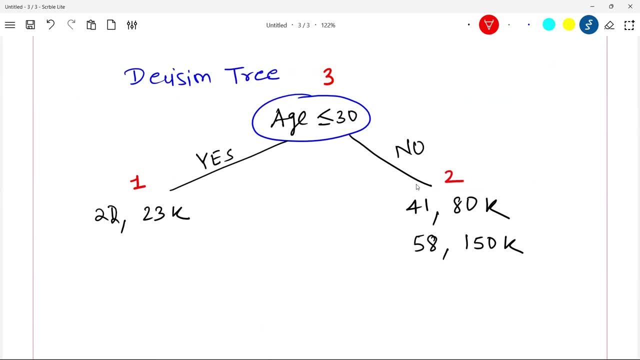 two records. okay, so this is first level of split. now decision: tree can split it one more time. okay, so tree can make here there are limited number of records, but imagine if there are more records there can be one more split here saying: you know, another filter is is maybe less than 40. 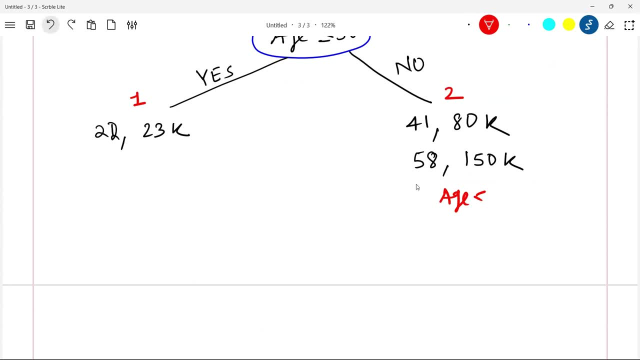 or something like this. okay, but i will not take that now. that will make the tree complex. okay, so this is your model. breaking your data based on some conditions is nothing but your model. so somebody asks you: what is your model in decision tree? this is your model. 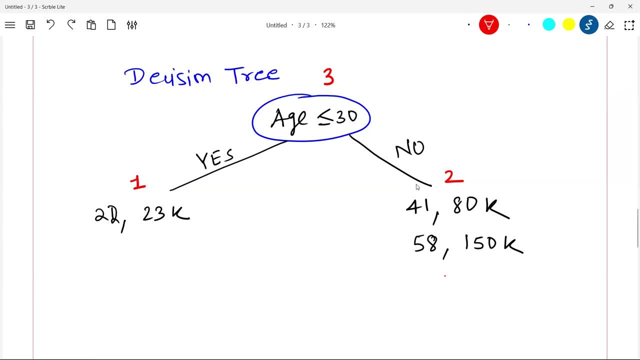 now the important question is: suppose tomorrow somebody comes and asks for a person with age 50, what is your prediction for a person with age 50? what is your prediction? very, very important concept to understand: guys decision tree will come and check: what is this for age 50? okay, so age 50 will come in. which category will come in this line? okay, in this. 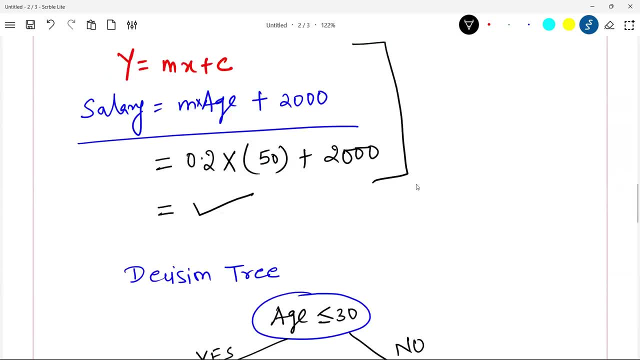 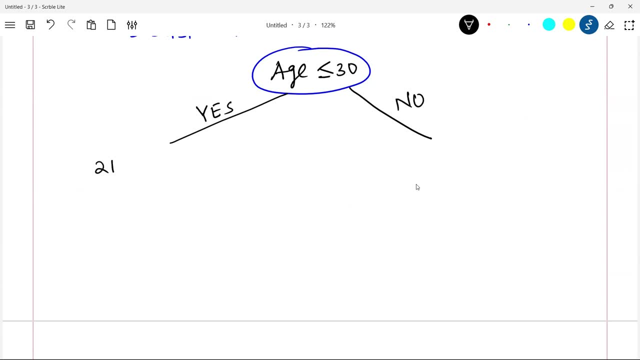 record age: more than 30, two records. so how many records will come this side? only one record will come, okay, so let's say that record is- I should not write the wrong numbers- 22, 23 k, 41, 80 k. so I will write here 22 and 23 k and here I will write 41 and 80 k. okay, and there is one more record. let 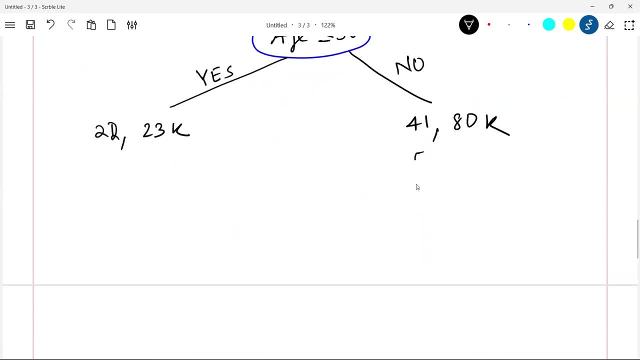 me take the numbers 58 and 150 k. 58 and 150 k. understand this carefully, guys, because for next next algorithms, this is the base. okay, so decision two tree will split your data like this. so you had total, how many records in the beginning three. 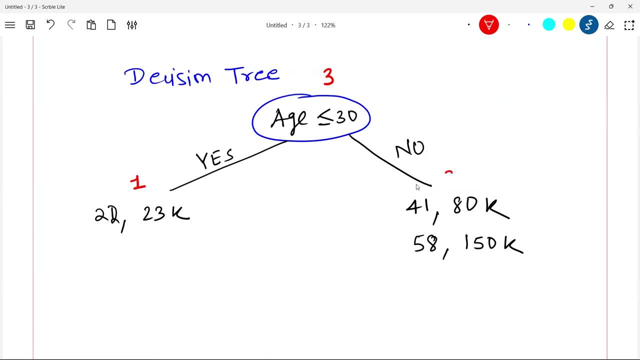 records here. how many records you are having one record here. how many records you are having two records? okay, so this is first level of split. now decision tree can split it one more time. okay, so tree can make here. there are limited number of records, but imagine if there are more records. 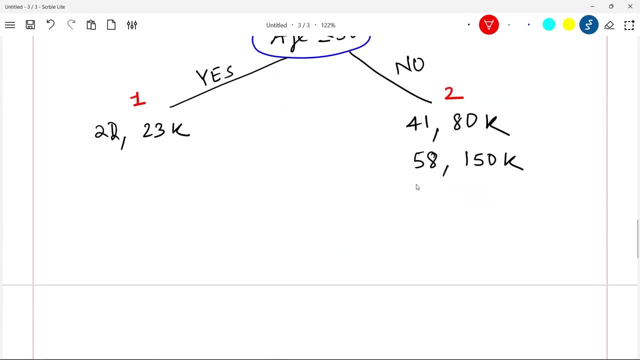 there can be one more split here saying: you know, another filter is is maybe less than 40 or something like this: okay, but I will not take that that now, that will make that tree complex. okay, so this is your model. breaking your data based on some conditions is nothing but your model. so somebody asks you: what is your model in decision tree? this: 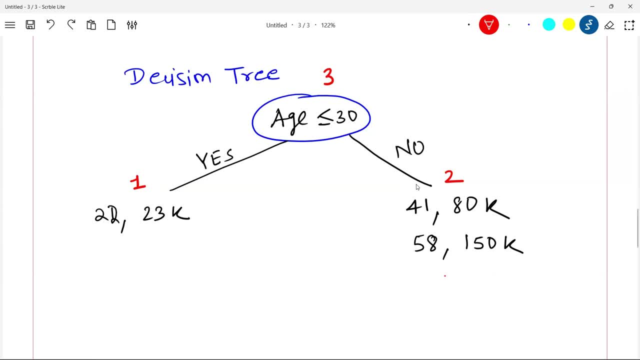 is your model? now the important question is: suppose tomorrow somebody comes and asks for a person with age 50. what is your prediction for a person with age 50? what is your prediction? very, very important concept to understand: guys decision tree will come and check your data for your data. 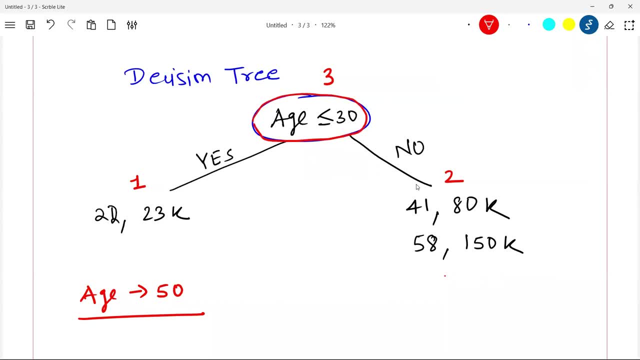 what is this for age 50? okay, so age 50 will come in. which category will come in this line? okay, in this line, how many records? are there? two records. so decision tree will go ahead and take the average of these two salaries. so, for age 50, your prediction will be: what will be the prediction, guys, for age 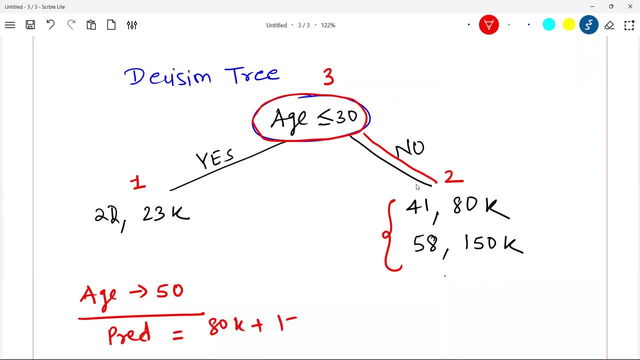 50 prediction will be 80k plus 150k divided by 2. okay, this is how decision tree will be making the prediction. suppose you ask to this entity: hey, what will be the salary of a person with age 21? so it will not go to right hand side, it will go to left hand side, because this is the tree branch in which it should. 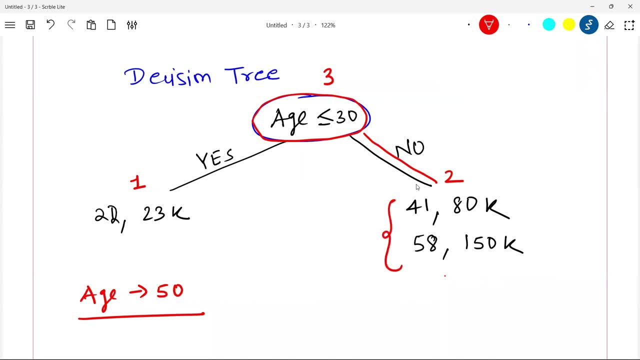 line. how many records are there? two records. so decision tree will go ahead and take the average of these two salaries. so for age 50, your prediction will be: what will be the prediction guys? for age 50, prediction will be 80k plus 150k divided by 2.. okay, this is how decision tree will be making. 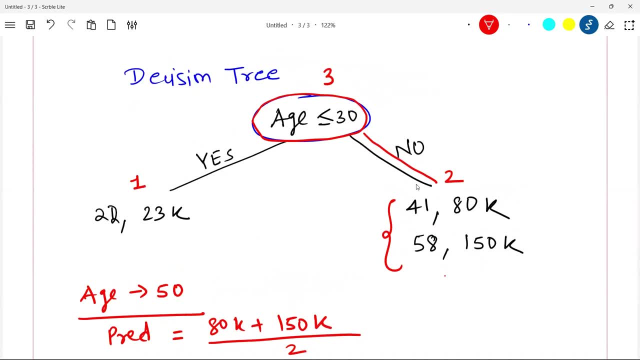 the prediction. suppose you ask to this entry: hey, what will be the salary of a person with age 21? so it will not go to right hand side, it will go to left hand side, because this is the tree branch in which it should go. it will directly say 23k in this case, because there is only one record. 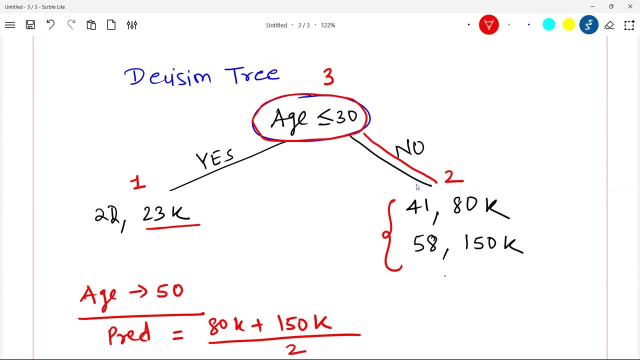 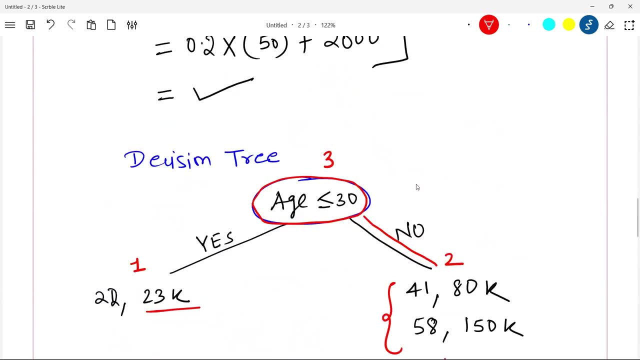 suppose there are two records, it will take the average. okay, so you see how these two approaches are different for solving same regression problem. here a mathematical line will be fit and here a decision tree. you know, data will be broken into multiple pieces and prediction will be made. 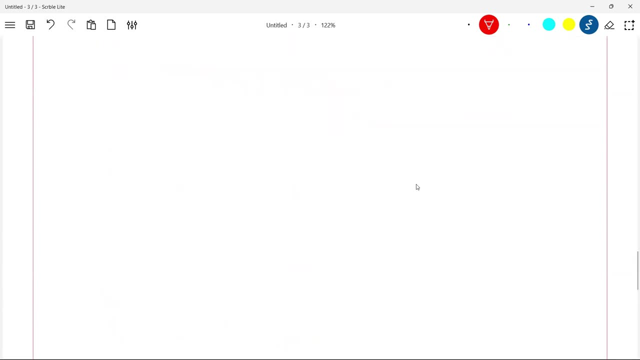 okay, remember guys, decision tree is base for many other advanced algorithms, and our third algorithm in the list is something known as a random forest. okay, a random forest. what random forest will do is? it will say: decision tree, okay, you have done a good job, but there is a chances of overfitting of the data. so we did not discuss pros and cons of this. 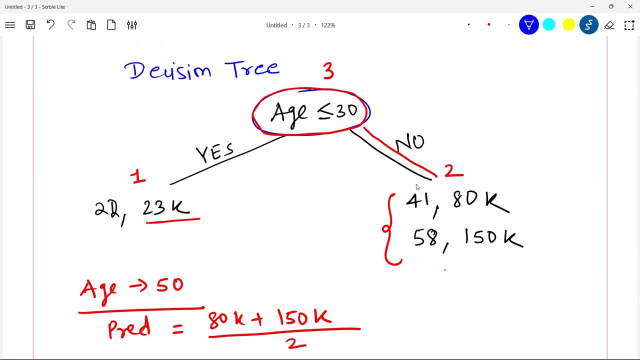 process. it's a simple model, you know you don't need to do a lot of mathematics etc. and cons is there is a chances of overfitting because you know if there is a little change in the data your model may change totally. that's the risk here in decision tree. so overfitting, so random forest will. 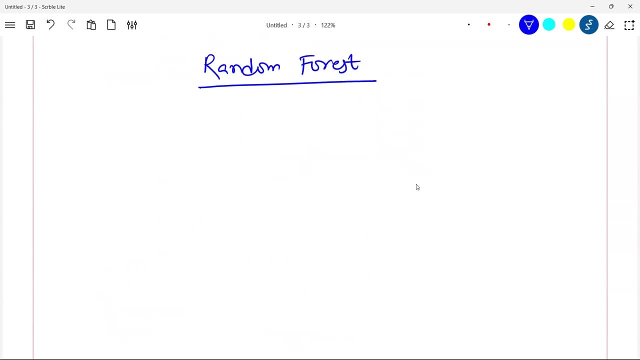 come and say, hey, you are taking a right approach, but there is a chance of overfitting, so why don't you fit multiple trees? so what random forest will do is it will come and create multiple trees. this is your tree one. okay, like the way we saw decision tree, this is your, for example, tree one. 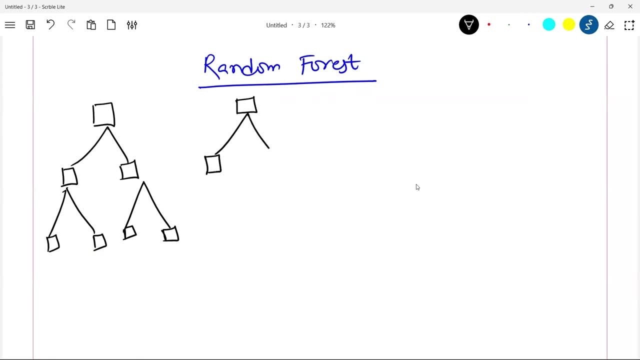 okay, this is your, for example, tree 2. okay, and similarly, there can be n number of trees. okay, similarly, there can be n number of trees. so we will call this as t1, we will call this as t2, and that there can be, you know, 500 trees, for example. so what random forest will do is it will say: 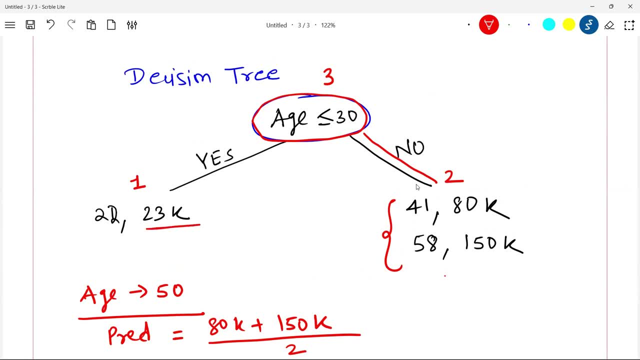 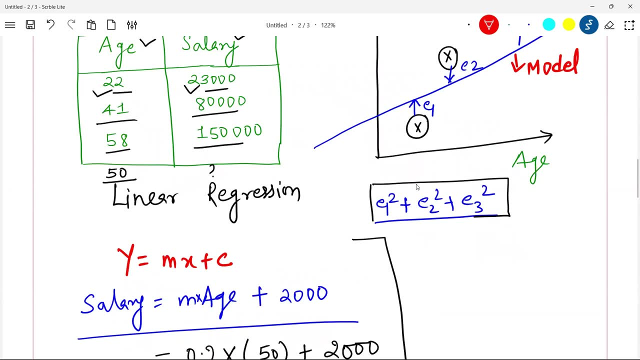 go, it will directly say 23k in this case because there is only one record. suppose there are two records, it will take the average. okay, so you see how these two approaches are different for solving same regression problem. here a mathematical line will be fit and here a decision tree. you know. 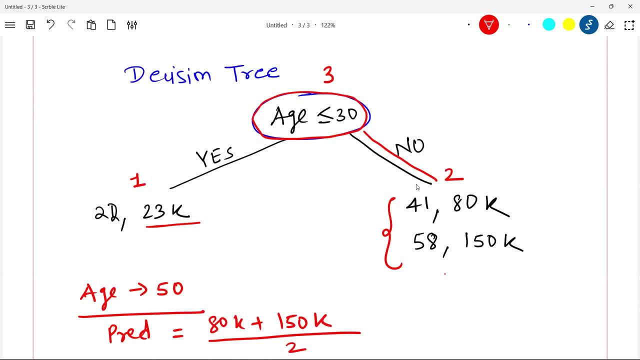 data will be broken into multiple pieces and predicts will be made. okay, remember guys. decision tree is base for many other advanced algorithms, and our third algorithm in the list is something known as a random forest. okay, a random forest. what random forest will do is it will say decision tree. 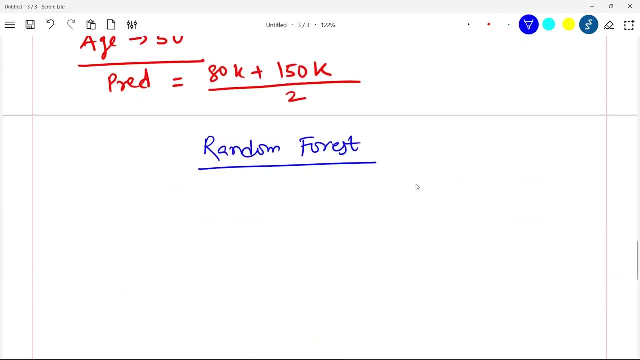 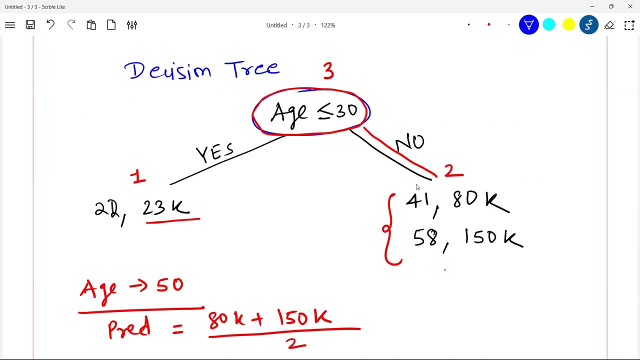 okay, you have done a good job, but, uh, there is a chances of overfitting of the data. so we did not discuss pros and cons of this process. it's a simple model, you know. you don't need to do a lot of mathematics, etc. you don't need to do a lot of mathematics, etc. you don't need to do a lot of mathematics, etc. 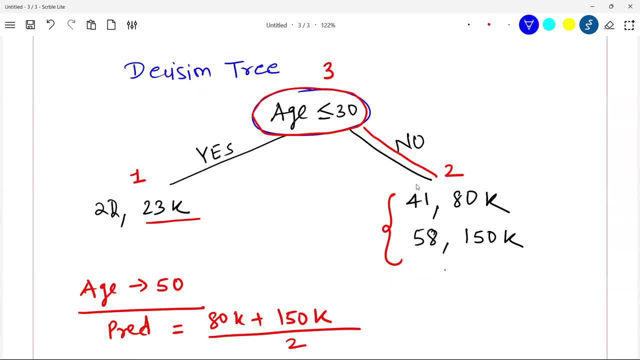 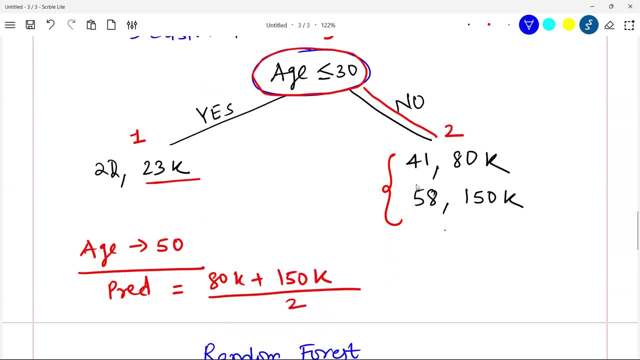 and cons is there is a chances of overfitting because you know if there is a little change in the data your model may change totally. that's a risk here in decision tree. so overfitting. so random forest will come and say: hey, you are taking a right approach, but there is a chance of 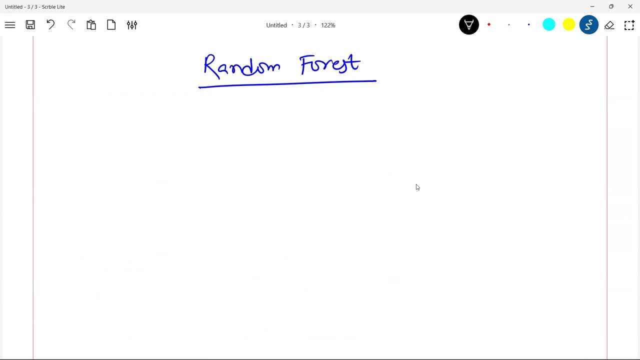 overfitting, so why don't you fit multiple trees? so what random forest will do is it will come and create multiple trees. this is your. tree one: okay, like the way we saw decision tree. this is your, for okay. this is your, for example. tree two: okay, and similarly, there can be n number of trees okay. 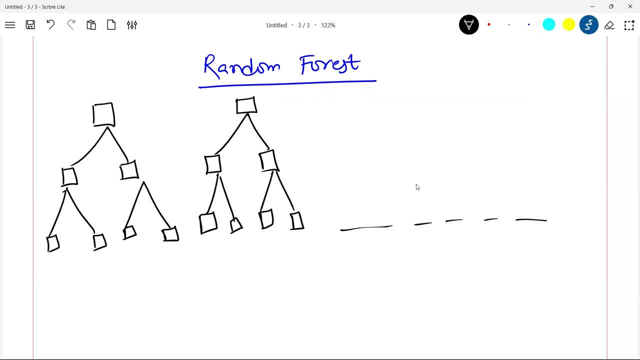 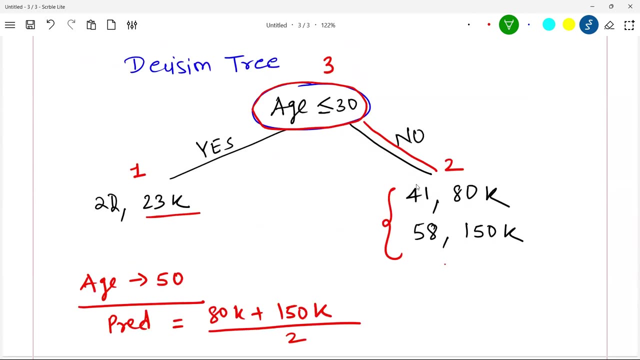 similarly, there can be n number of trees, so we will call this as t1, we will call this as t2, and that there can be, you know, 500 trees, for example. so what random forest will do is it will say to decision tree: hey, if you are fitting one tree, there is a chance of result being biased. or 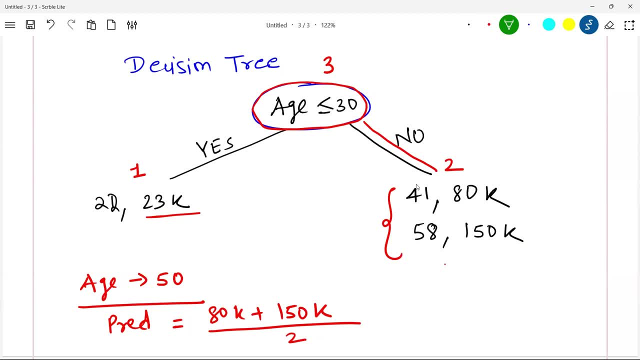 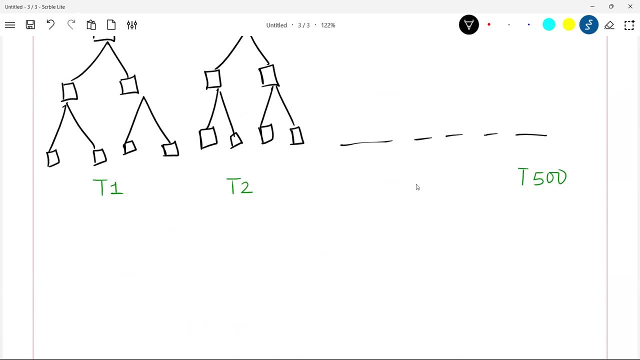 there is a chance of overfitting or there is a chance of model not being stable, but what i will do is i will fit 500 trees. okay, and how i will make the prediction is very important to understand here. guys, prediction of random forest will be average of all these prediction. for example, if 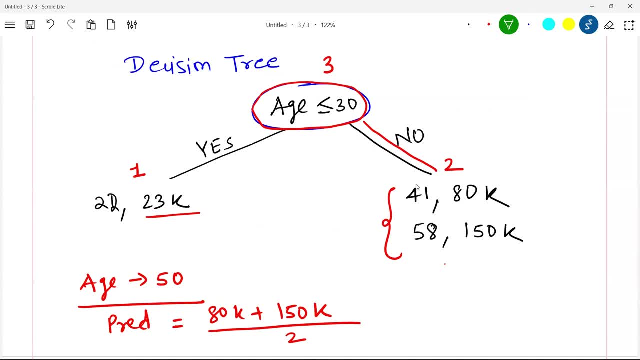 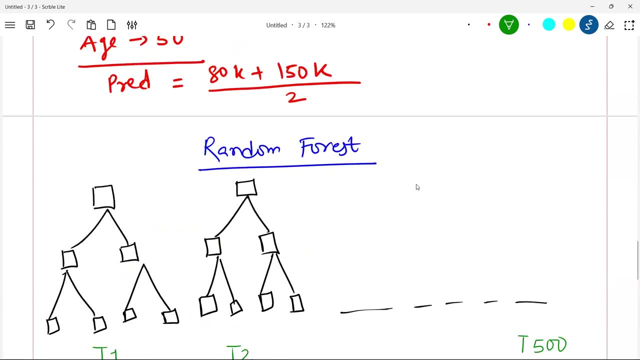 to decision tree. hey, if you are fitting one tree, there is a chance of result being biased, or there is a chance of overfitting, or there is a chance of model not being stable. but what I will do is I will fit 500 trees, okay, and how I will make the prediction is very 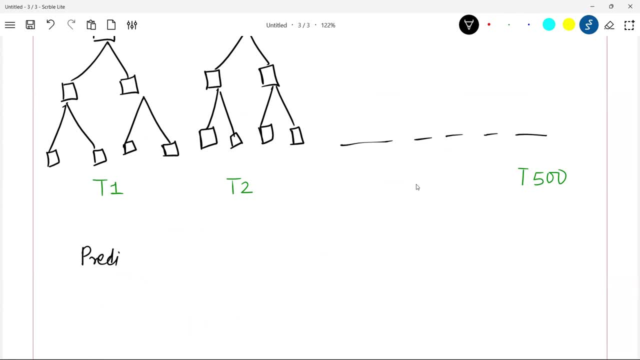 important to understand here, guys: prediction of random forest will be average of all these prediction. for example, if we are trying to predict for the age 50- right, for the age 50, what will be the salary? if we are trying to predict, okay, then in random forest it will. 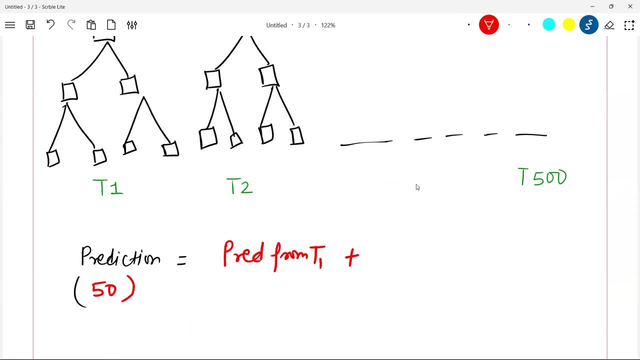 take prediction from tree 1 plus prediction from tree 2 plus prediction from tree 500. okay, it will take all the predictions and it will take a average of that. what is the? what is the thing that we are trying to achieve here? suppose in one decision tree your tree is. 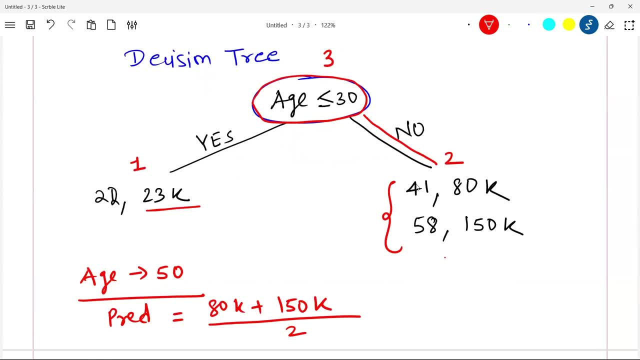 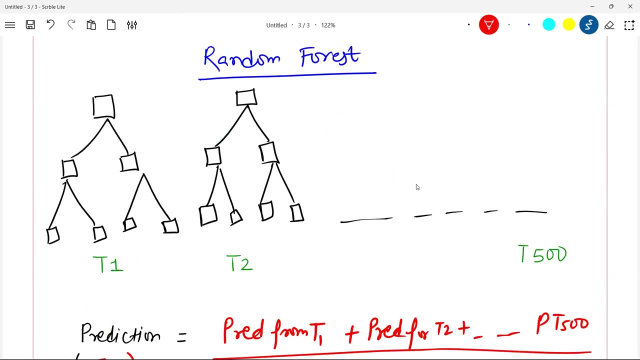 overfitting or not performing well or is biased. okay, so what may happen in decision tree, since you are taking a feedback from 500 trees- different trees- so that overfitting problem or model instability problem may not be there. okay, so this is how random forest is different from decision tree. remember all these individual. 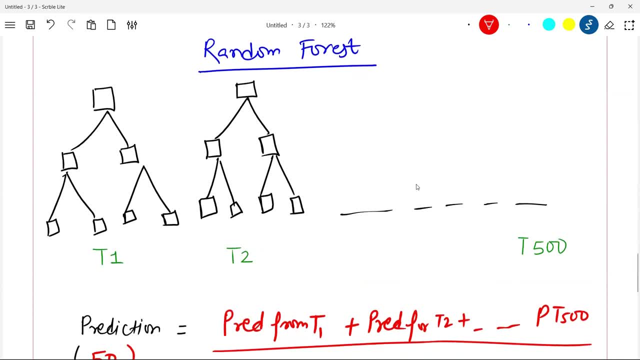 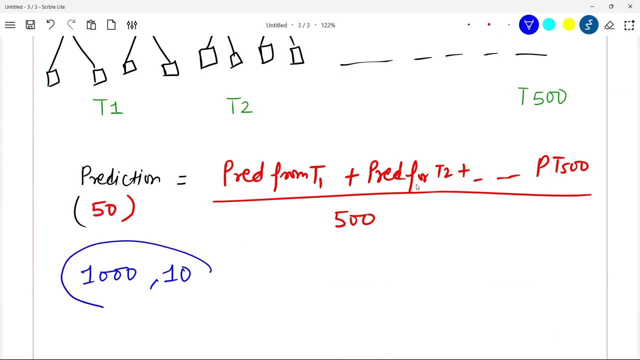 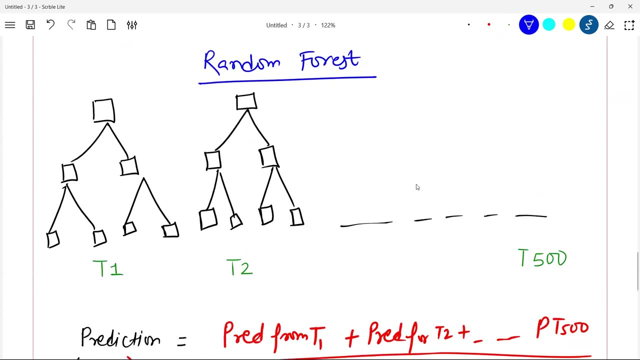 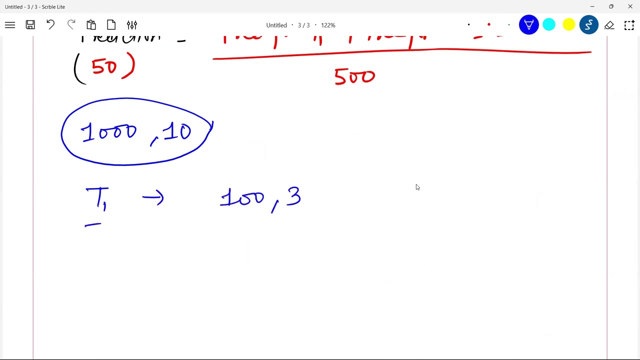 trees will not be using all the data. for example, suppose in your data there is 1000 rows and 10 columns. okay, just an example I'm giving. so all these, all these trees will not use necessarily all the records. it may be possible that tree 1 is using 100 records and 3 columns randomly selected. 3 to t2 is using 3 to 100. 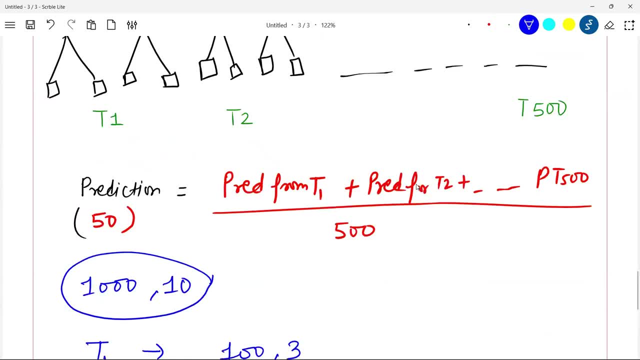 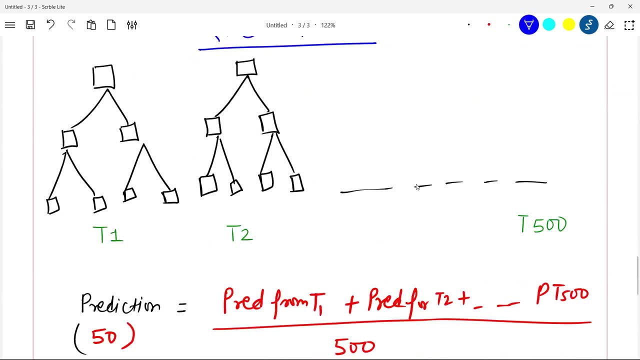 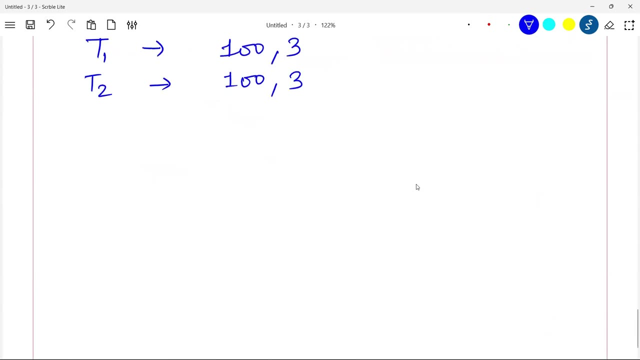 records and 3 columns randomly selected. okay, and that is the advantage of this random forest, that all these trees will may learn a different kind of pattern and when you take a aggregated result, then you will have all the flavors. okay, this kind of learning that I just explained. 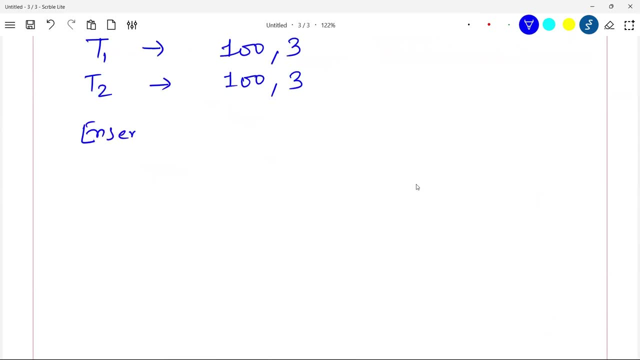 you is known as ensemble learning. okay, remember, guys, at unfold data science you will find a big playlist explaining all the algorithms of ensemble learning in detail. I will paste the link in the description. you must check if you have any confusion on how ensemble learning works. okay, but there is. 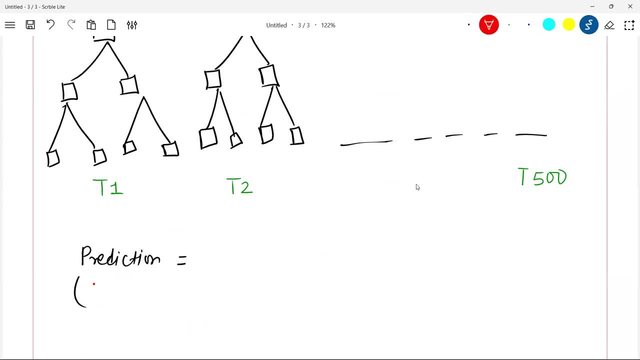 we are trying to predict for the age 50. right, for the age 50, what will be the salary? if we are trying to predict, okay, then in random forest, it will take: prediction from tree 1 plus prediction from tree 2 plus prediction from tree 500. okay, it will take. 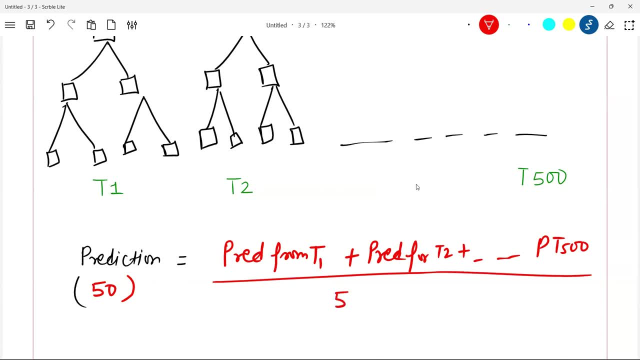 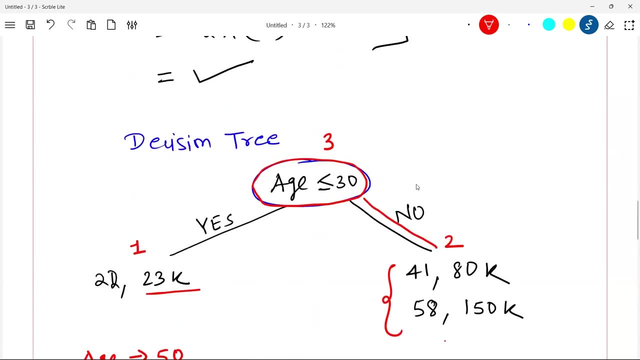 all the predictions and it will take a average of that. what is the? what is the thing that we are trying to achieve here? suppose, in one decision tree, your tree is overfitting or not performing well or is biased. okay, so what may happen in decision tree, since you are taking a feedback? 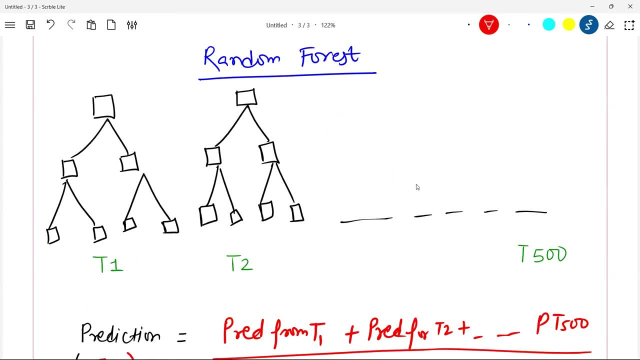 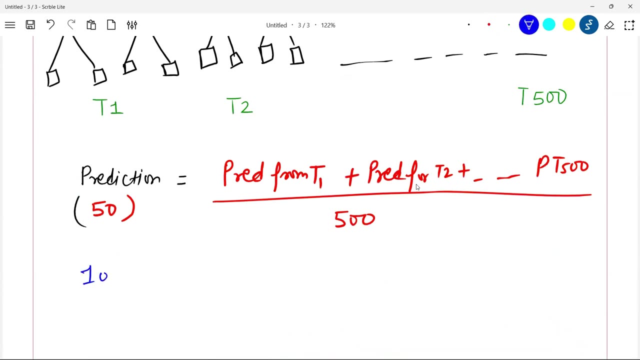 from different trees so that overfitting problem or model instability problem may not be there. okay, so this is how random forest is different from decision tree. remember all these individual trees will not be using all the data. for example, suppose in your data there is 1000 rows and 10. 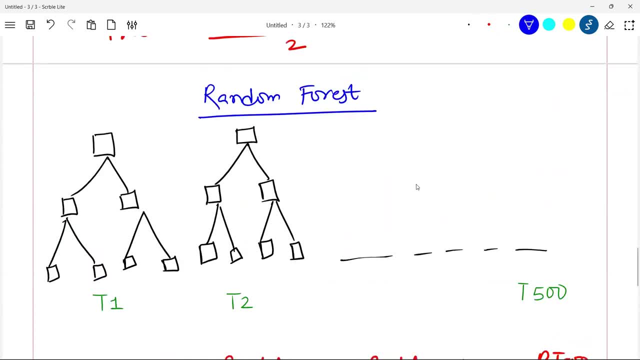 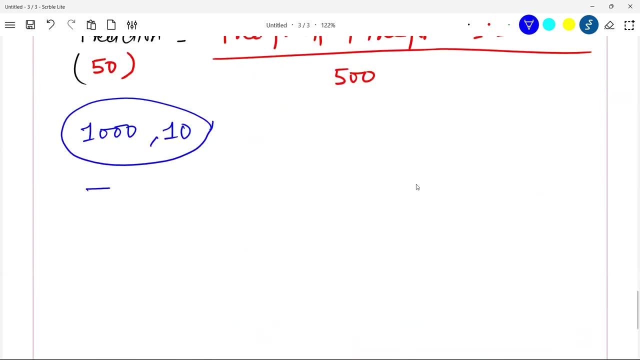 columns. okay, just an example i am giving. so all these, all these trees will not use necessarily all the records. it may be possible that tree 1 is using 100 records and 3 columns randomly selected: 3, 2. t. 2 is using 3, 2- 100. 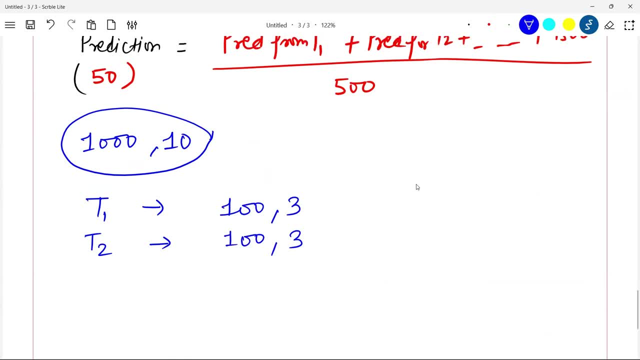 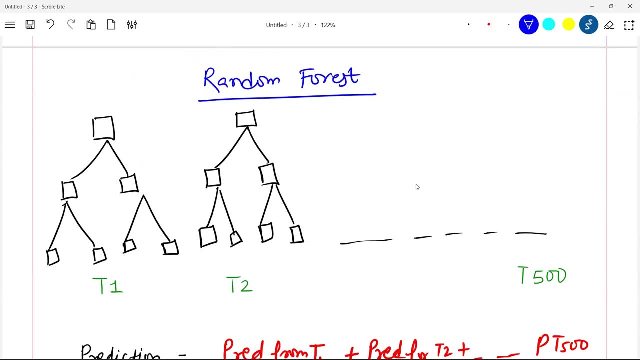 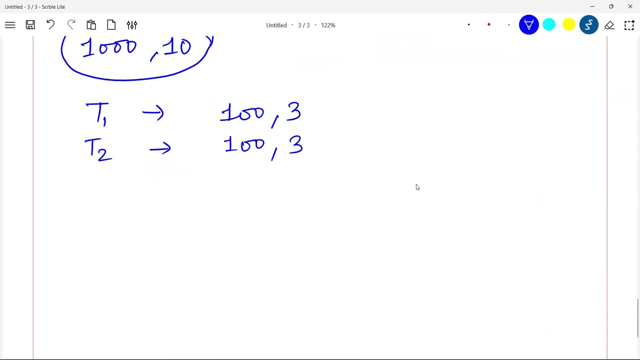 records and 3 columns randomly selected. okay, and that is the advantage of this random forest, that all these trees will may learn a different kind of pattern and when you take a aggregated result, then you will have all the flavors. okay, this kind of learning that i just explained you is known as 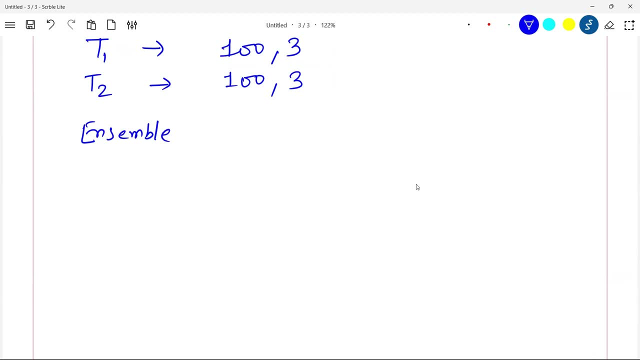 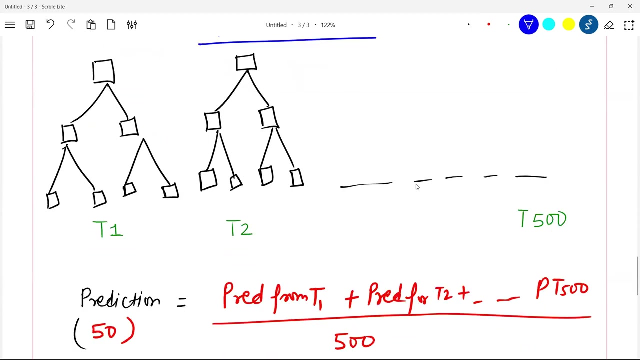 ensemble learning. okay, remember, guys, at unfold data science, you will find a big playlist explaining all the algorithms of ensemble learning in detail. i will paste the link in the description. you must check if you have any confusion on how ensemble learning works. okay, but there is more to ensemble learning. 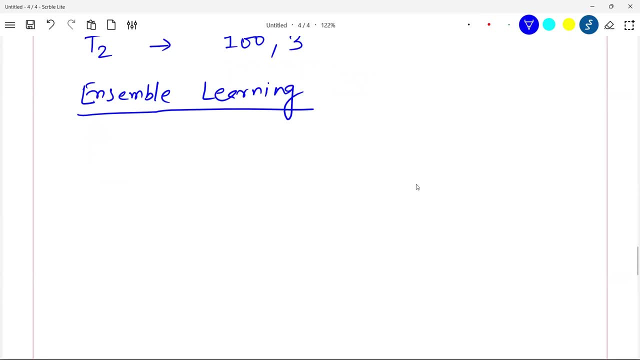 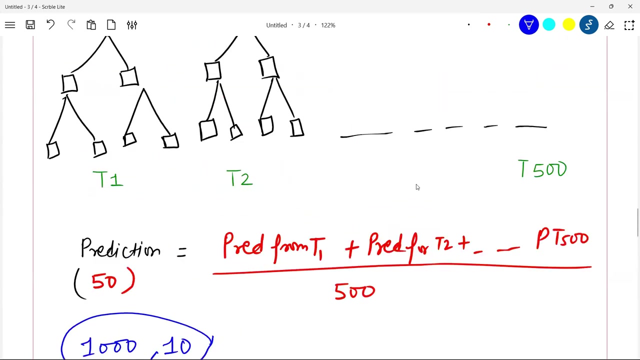 what happened just now in random forest is known as parallel way of learning. okay, parallel way of learning. parallel way of learning. why parallel way of learning, guys? because here tree 1 and tree 2 and tree 3 are independent of each other. when you call a random forest model, tree 1 can start. 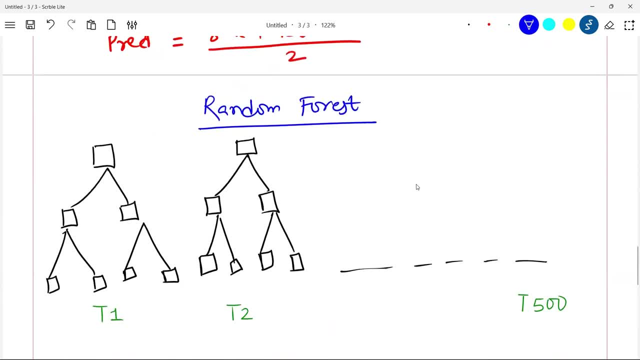 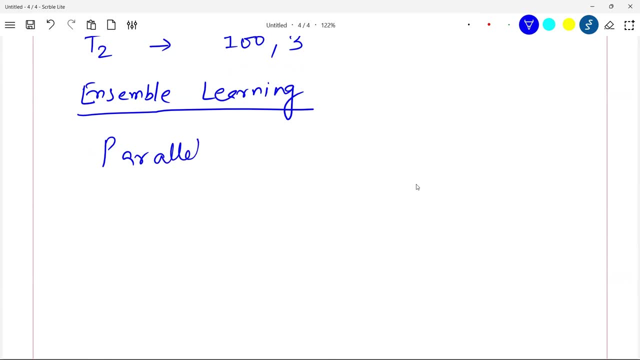 more to ensemble learning. what happened just now in random forest is known as parallel way of learning. okay, parallel way of learning. parallel way of learning. why parallel way of learning, guys? because here tree 1 and tree 2 and tree 3 are independent of each other when you call. 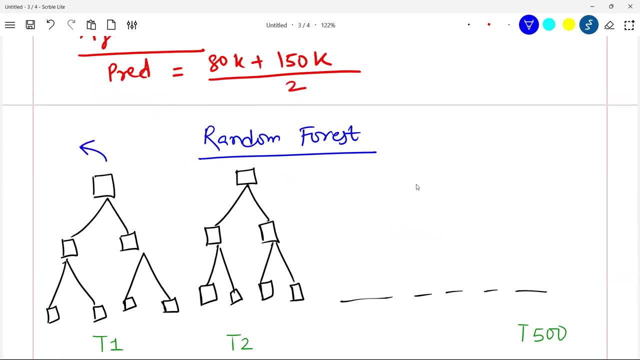 a random forest model. tree 1 can start building by taking a sub sample of the data. tree 2 can start building by taking a sub sample of the data. they are not dependent on each other, okay, so all these things can happen parallelly, hence we call it a parallel learning. 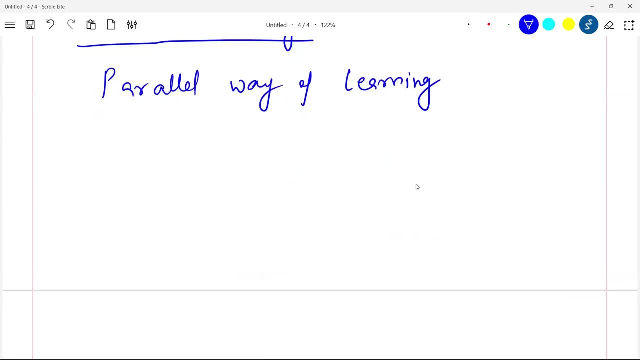 now the question is: is there another way of learning in ensemble? yes, there comes our next algorithm, known as add a boost. okay, add a boost standing for adaptive boosting. so what add a boost will do is: let me write the data here. let me write the data one more time and I may be writing some different numbers. 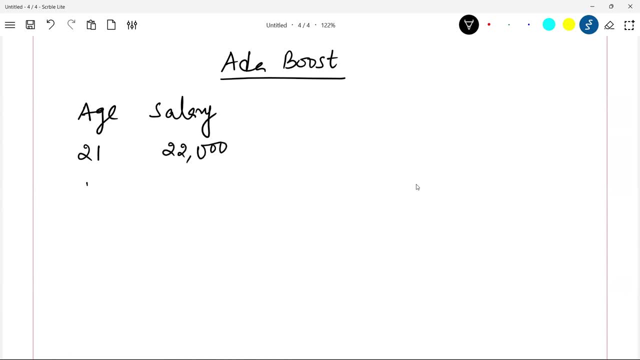 so that's not important. just understanding the concept is important. okay, so 42, I will write 50,000, and let's say 58, I will write 150,000, just as an example. this is your input data. so Boosting, Boosting is another technique. boosting is another technique of ensemble category. okay, 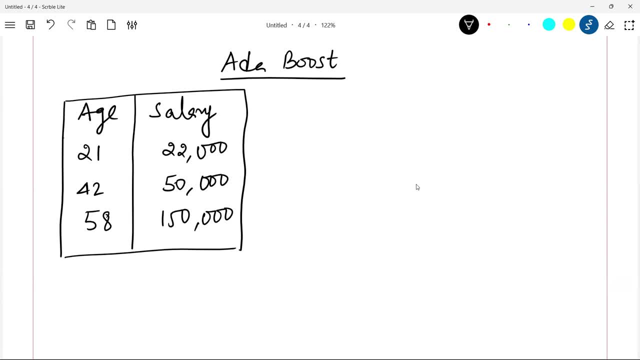 in boosting, especially add a boost. what will happen is it will assign a weight to all your observations. okay, suppose this is your original data for training, salary being your target column. so initial weights, initial weights, okay, and what the initial weights will be, it will be the same weight. 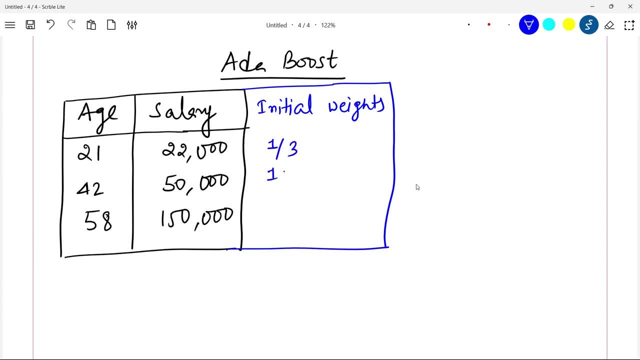 so Do all your records. for example, there are three records, so one by three. I'm saying one by three. I'm saying one by three, I'm saying so. all the rows are equally important. okay, try to understand the concept, guys in. add a boost in the beginning. first iteration, all. 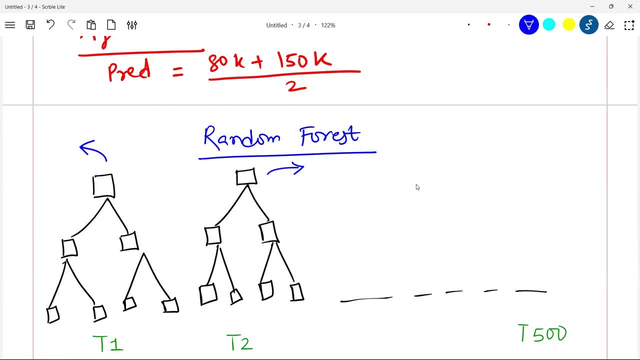 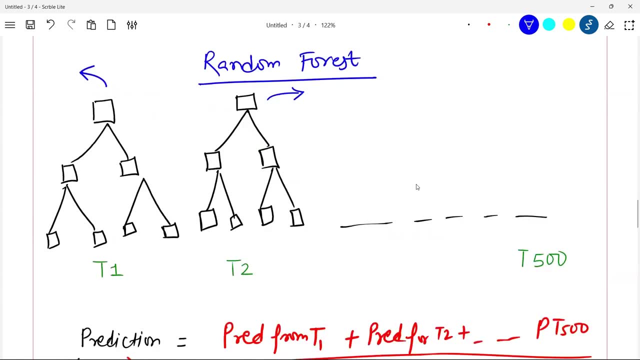 building by taking a sub sample of the data. tree 2 can start building by taking a sub sample of the data. they are not dependent on each other, okay, so all these things can happen parallelly. hence we call it a parallel learning. now the question is: is there another way of learning in ensemble? yes, 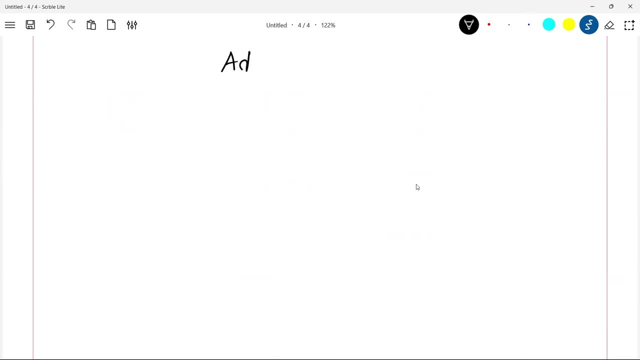 there comes our next algorithm, known as ada boost. okay, ada boost standing for adaptive boosting. so what ada boost will do is: let me write the data here. let me write the data one more time, and i may be writing some different numbers, so that's not important. just understanding the concept is. 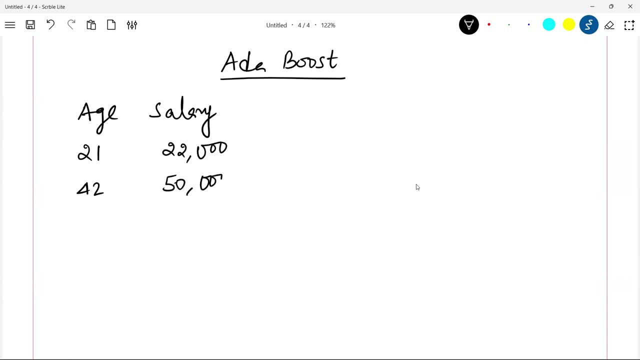 important. okay, so 42, i will write 50 000, and let's say 58, i will write 150 000, just as an example. this is your input data. so boosting is another technique. boosting is another technique of ensemble category. okay, in boosting, especially ada boost, what will happen is: 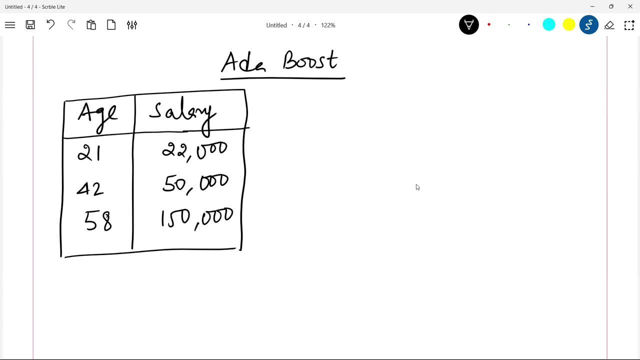 it will assign a weight to all your observations. okay, suppose this is your original data for training, salary being your target column. so initial weights, initial weights, okay, and what the initial weights will be, it will be the same weight for all your records. for example, there are three records, so one by three, i am saying one by three, i am saying one by three, i am saying so. 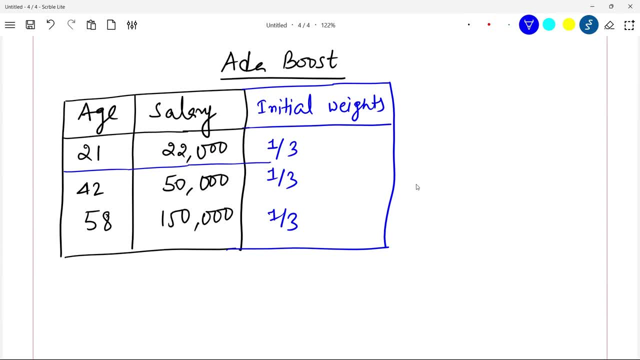 all the rows are equally important. okay, try to understand the concept, guys. in ada boost in the beginning, first iteration, all the rows are equally important. okay, but how ada boost works is in the name only there is adaptive. it adapts to the mistakes of the previous model. 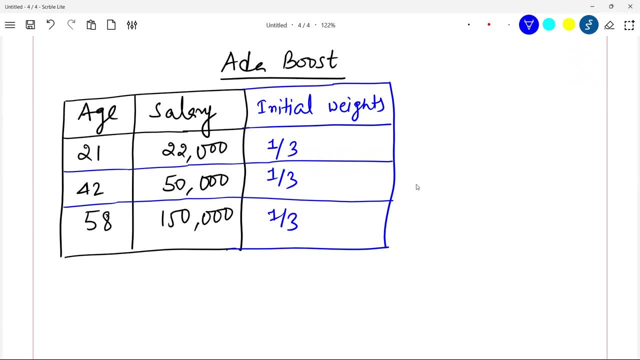 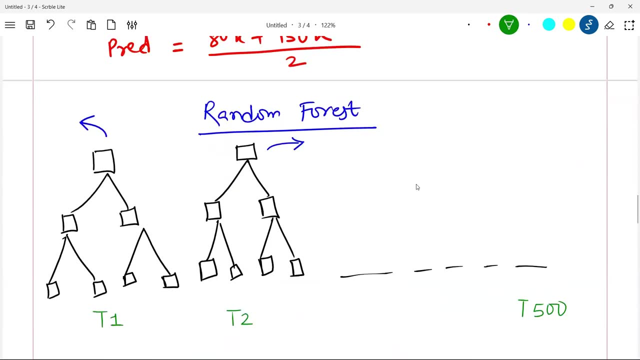 why i am saying a previous model and next model is one thing you have to always remember: ada boost is a sequential learning process. you, you remember how i just now told. random forest is a parallel learning process. so in random forest, tree one and tree two are independent of each other. okay it. 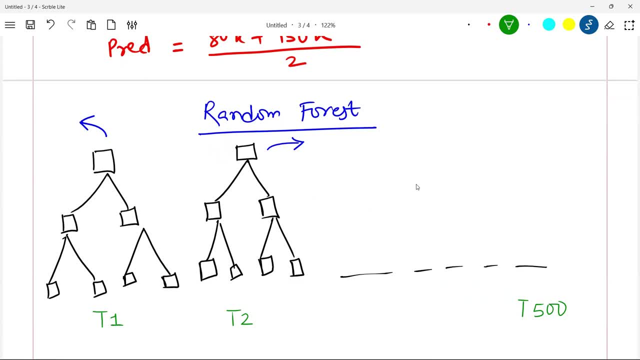 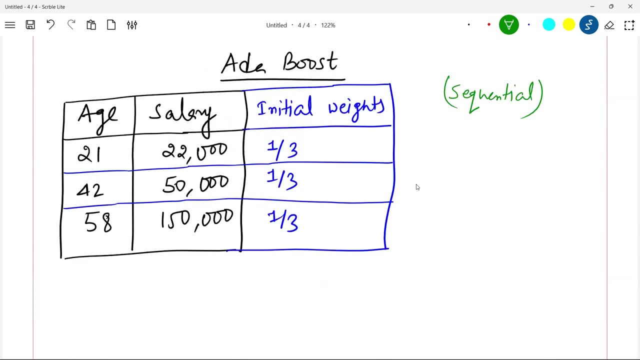 will take a sub sample and create. it will take a sub sample and create. nothing to do with each other. but in ada, boost or other boosting techniques, it's a sequential model, so there will be a multiple models in this. so there will be multiple models fitted to the data i will tell you in a moment. 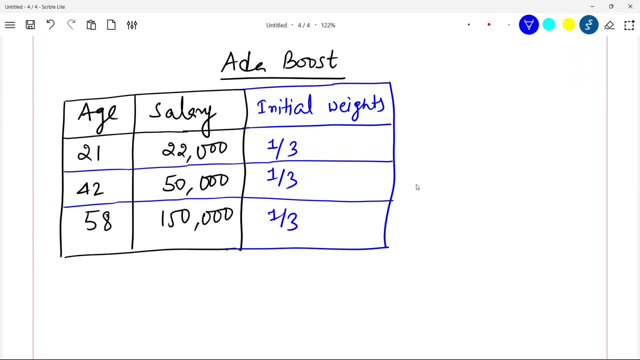 the rows are equally important. okay, but how other boost works is in the name only there is adaptive. it adapts to the mistakes of the previous model. now why I am saying a previous model and next model is Boost Boost. to always remember ada, boost is a sequential learning process. you, you remember how i just 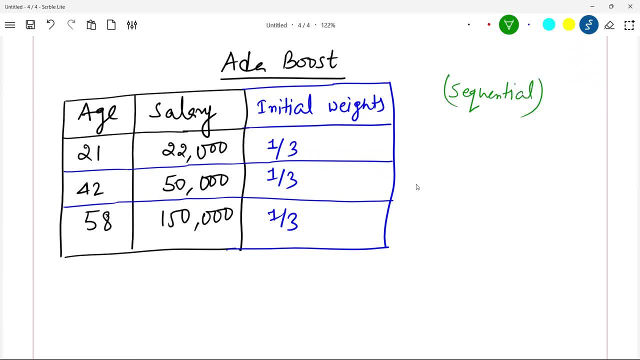 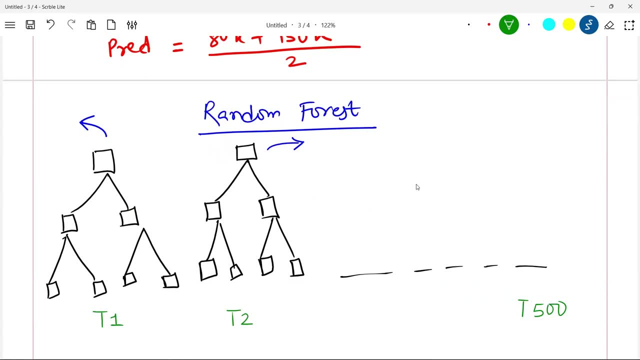 now told. random forest is a parallel learning process, so in random forest, tree one and tree two are independent of each other. okay, it will take a sub sample and create. it will take a sub sample and create. nothing to do with each other. but in ada, boost or other boosting techniques. 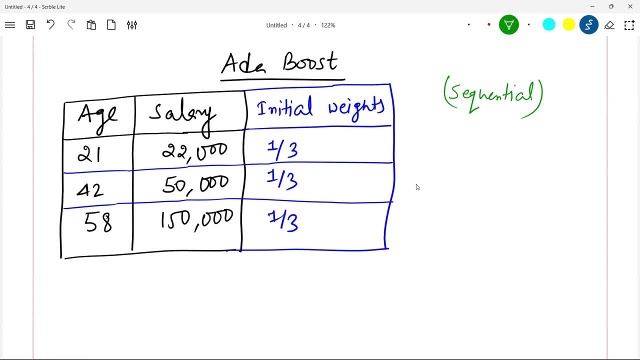 it's a sequential model, so there will be a multiple models in this. so there will be multiple models fitted to the data. i will tell you in a moment what these models will be: model 1, model 2, model 3, model 4 and so on and so forth, how many ever model comes, but it will not happen parallely. 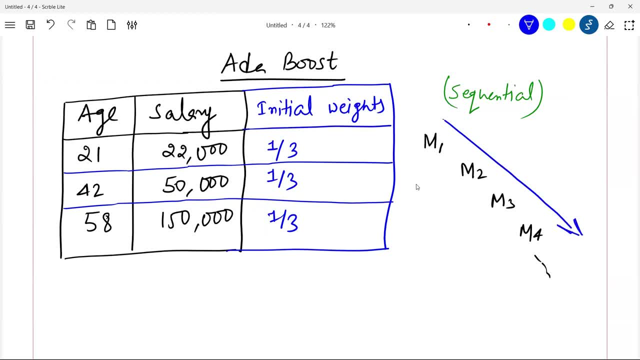 okay, it will happen in sequence. now the important thing to understand is how this sequence will be generated. okay, so what will happen? is this model one you can think of as a base model, this model one you can think of as a base model and remember, in ada boost? 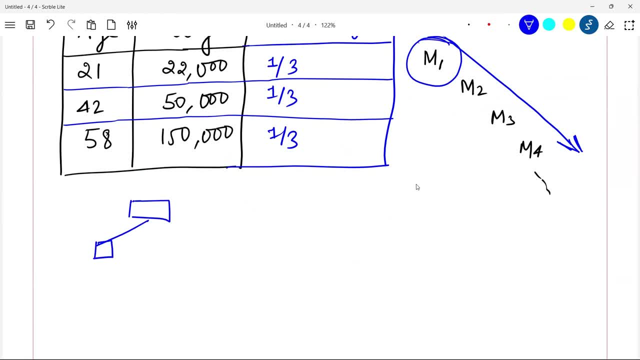 your decision, trees will look like stumps. stumps means there will be a tree like this and there will be another tree like this. so it will. the depth of the tree will not be beyond one level. okay, so this is called stumps in the language of machine learning, so multiple stumps will. 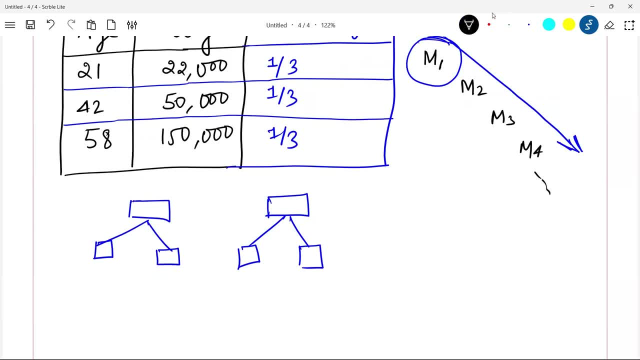 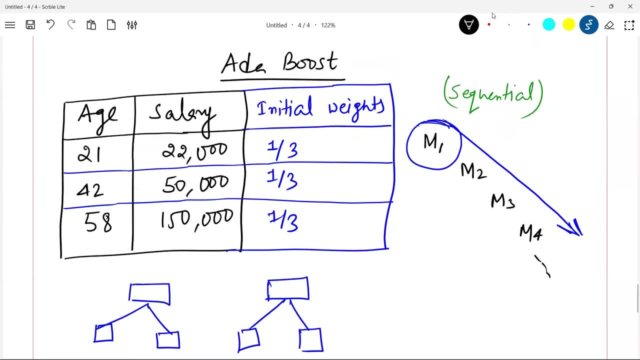 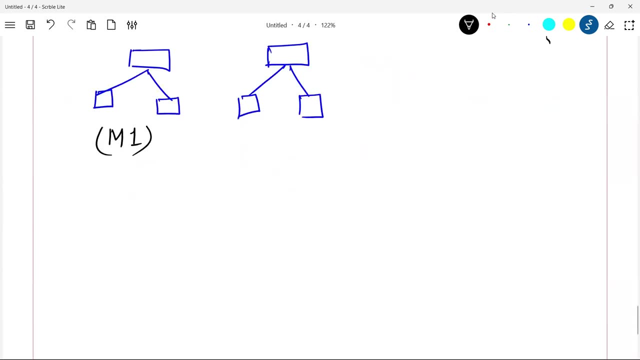 be created. now suppose your model one is this: first stump. what is your model one, guys? this first stump. okay. model one comes and make some prediction about the salary. model one comes and make some predictions about this salary. okay, so what we will have is another column called as. 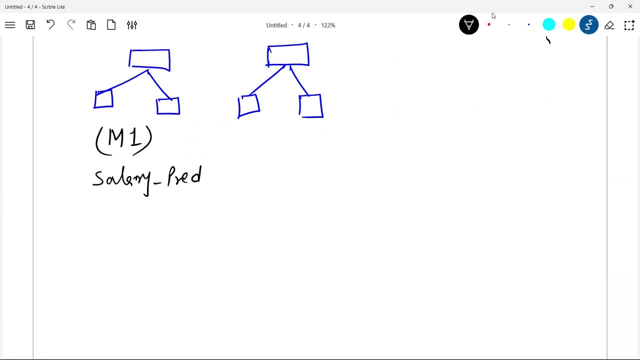 salary underscore prediction and where from this prediction comes. this prediction comes from model one, the first model, okay, so obviously there will be some mistakes. so 22 000 may be said as 21 900 and 50 and 150 can be said as. 50 can be said as, let's say, 52 000, okay, and 150 can be said as, let's. 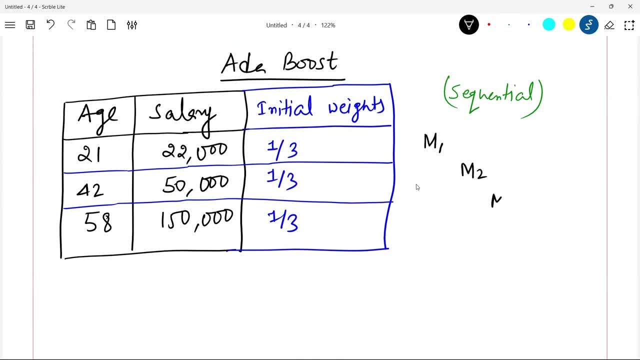 what these models will be: model 1, model 2, model 3, model 4, and so on and so forth, how many ever model comes, but it will not happen parallelly. okay, it will happen in sequence. now the important thing to understand is how this sequence will be generated. okay, so what will happen is this: 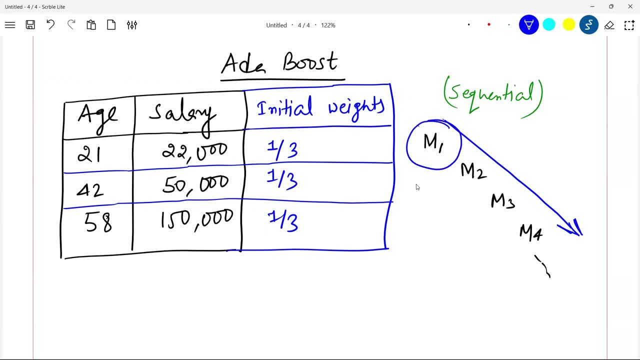 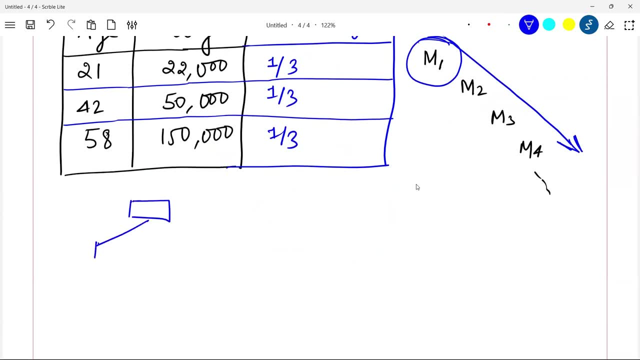 model, one you can think of as a base model. this model one you can think of as a base model, and remember, in ada, boost your decision. trees will look like stumps. stumps means there will be a tree like this and there will be another tree like this, so it will. 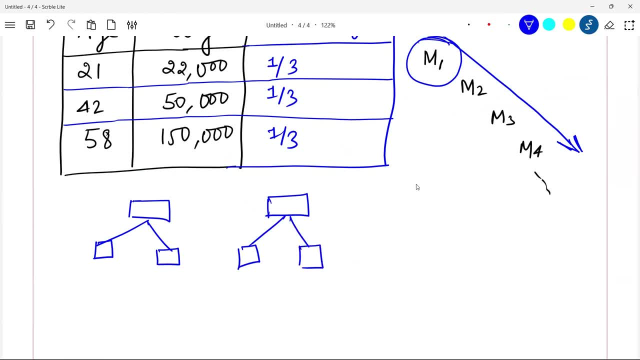 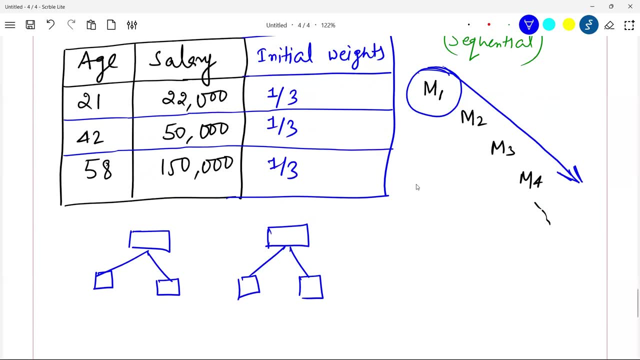 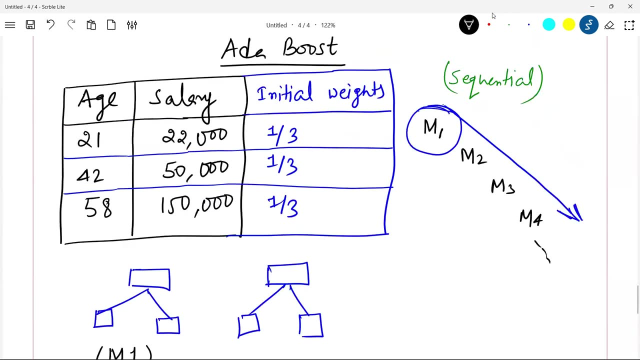 the depth of the tree will not be beyond one level. okay, so this is called stumps in the language of machine learning. so multiple stumps will be created. now suppose your model 1 is this first stump. what is your model 1, guys? this first stump. okay, model one comes and make some prediction. 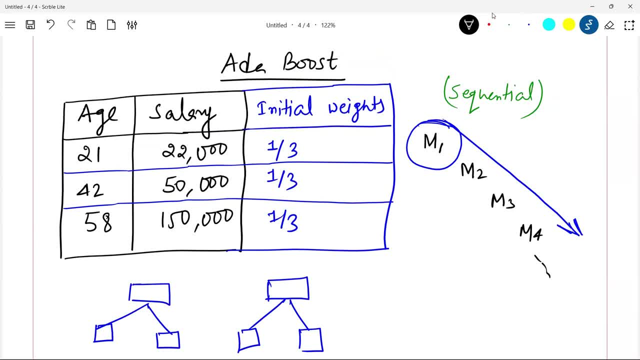 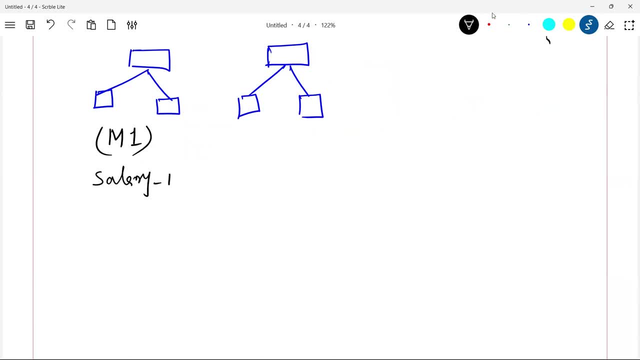 about the salary. model one comes and make some predictions about this salary. okay, so what we will have is another column called as salary underscore prediction and where from this prediction comes. this prediction comes from model one, the first model. okay, so obviously there will be some mistakes. so 22 000 may be said as 21 900 and 50 and 150 can be said as 50 can be said as. 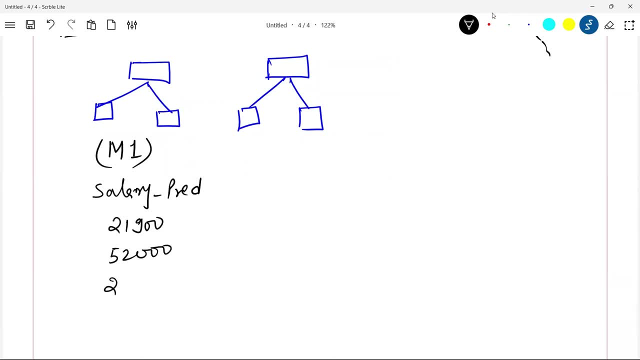 let's say 52 000, okay, and 150 can be said as, let's say, 200 000, based on this first model, first decision tree that it is creating, which i am calling a system. so there will be some differences between actual and predicted, and from this there will be a residual coming. residual means errors. 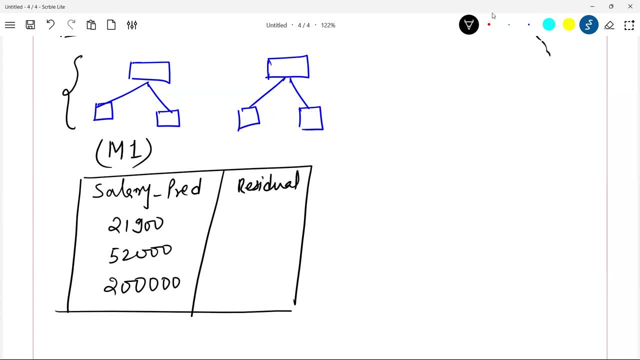 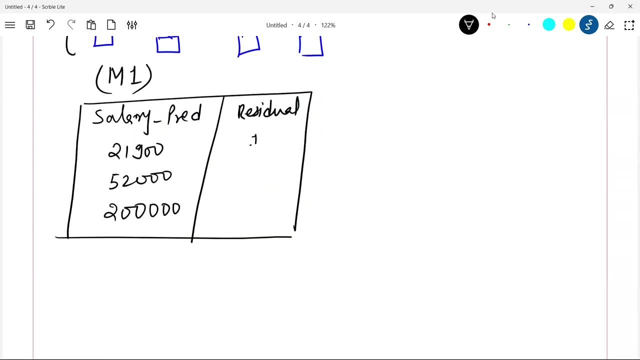 right, residual means errors. okay, so what will be the errors? 21 900 minus 22 000, right, so it will be. for example, i can say 100 actual minus predicted, it is minus 2000 and it is minus minus 50 000 because we have 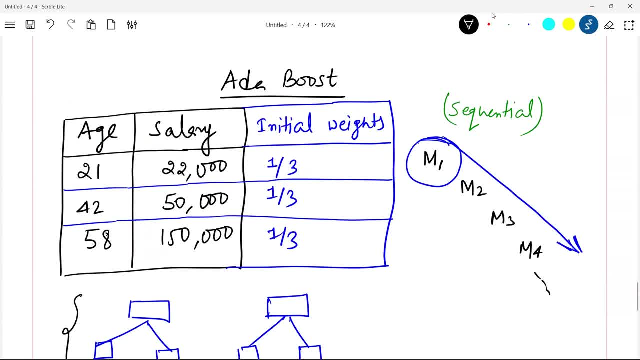 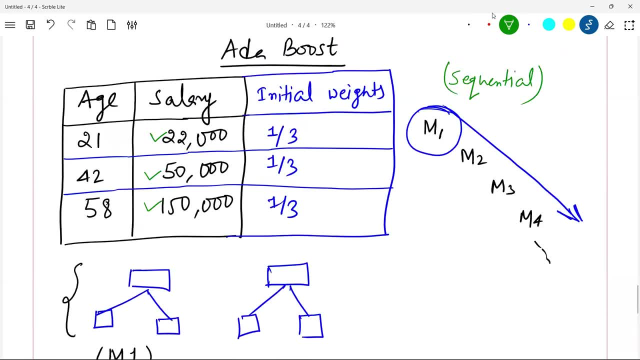 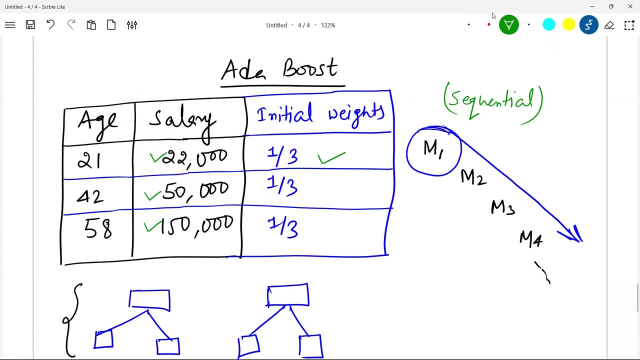 put. okay, so this is the errors. these are the actual values and the first model, what it predicts. right? those are the errors from the first model. okay, 22 000 minus 21 900 is 100, and so on and so forth. now these are the initial weights. okay, so what will happen in the next model? 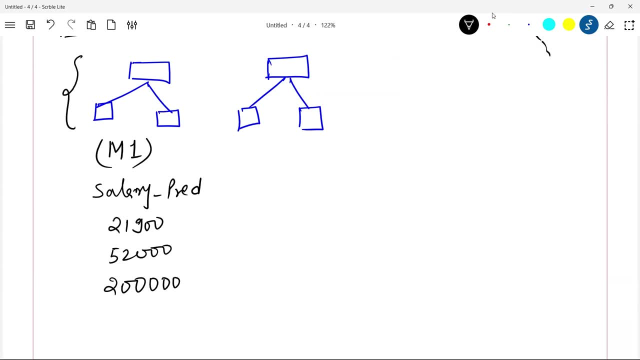 do based on this first model, first decision tree that it is creating, which i am calling a stump. so there will be some differences between actual and predicted and from this there will be a residual coming. residual means errors, right, residual means errors, okay. so what will be the errors? 21 900 minus 22 000 right. so it will be, for example, i can say, 100 actual minus predicted. 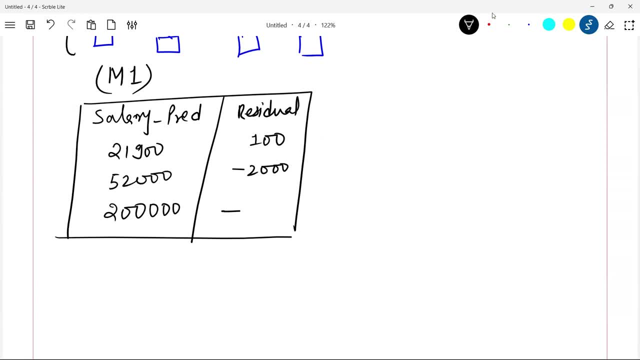 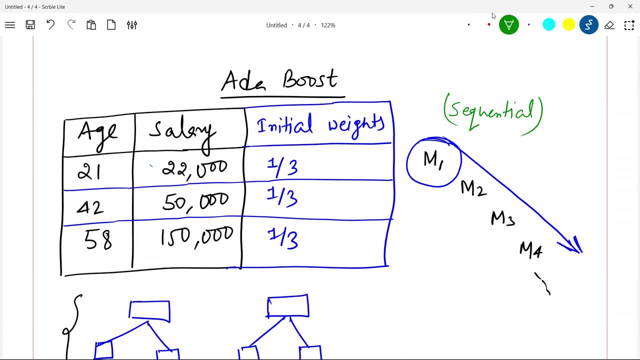 it is minus two thousand- and it will be the first decision tree that i am creating, which i am calling a stumps- is minus minus 50 000 because we have put okay. so this is the errors. these are the actual values and the first model, what it predicts. right, those are the errors from the first model. okay, 22 000. 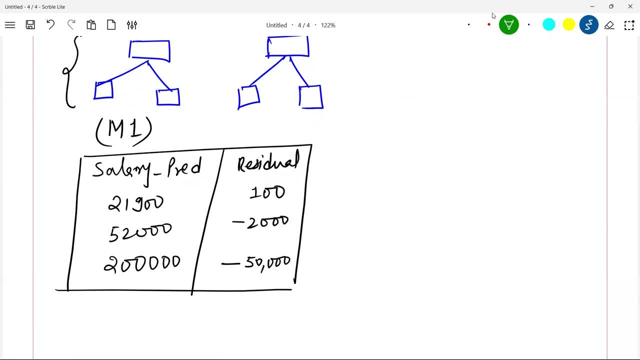 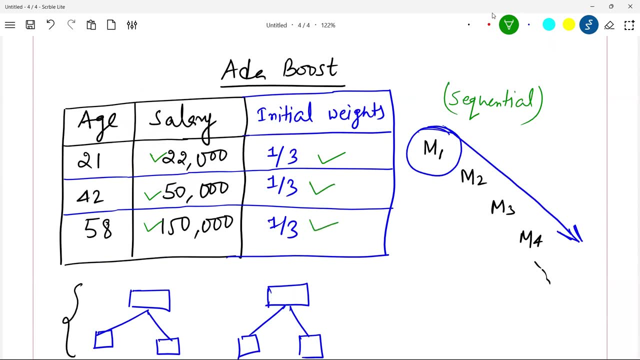 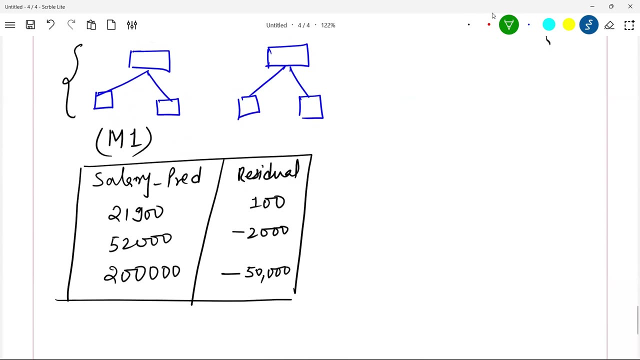 minus 21, 900 is 100, and so on and so forth. now these are the initial weights. okay, so what will happen in the next model when the m2 is fitted right? these initial weights will be changed and more preference will be given to the observations where these residuals are more okay. i am repeating: 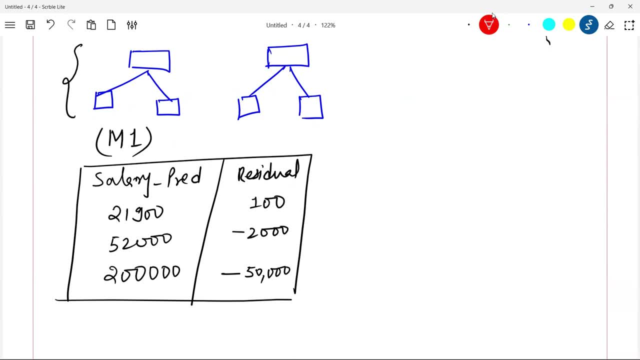 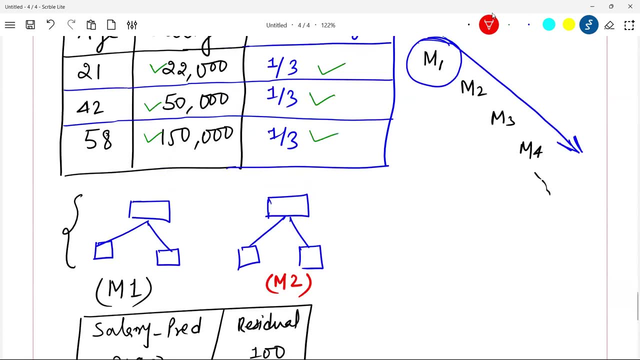 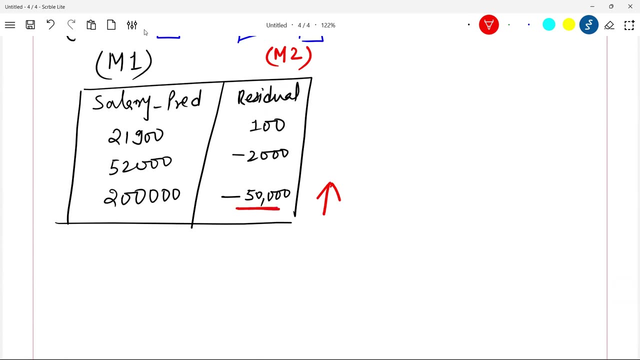 one more time, guys. m1 will predict this and then residuals or errors will come. when the m2 is trained right, then the weights will not be same for all these three records. rather, weight will be increased for this because you are getting more errors here, and weight will be decreased for this because you are getting less error here. okay. 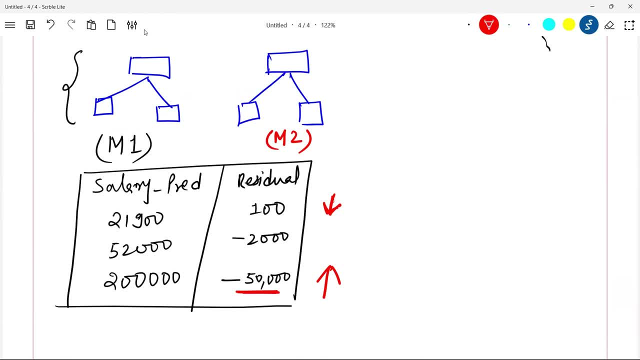 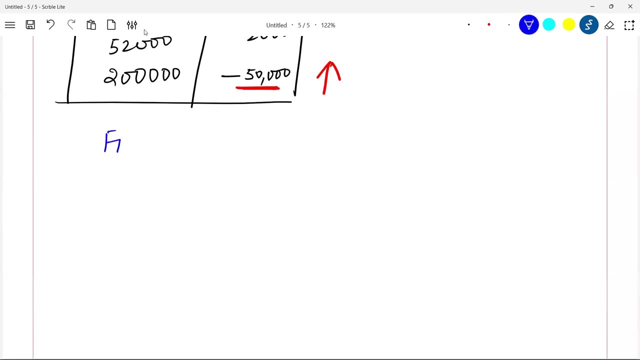 and so on and so forth. m2 will come compute, create the residual. then again, weights will be adjusted. m3 will come predict, residual will be calculated, weights will be adjusted and, finally, what you will get is a combination of what will be your final model. your final model will be: 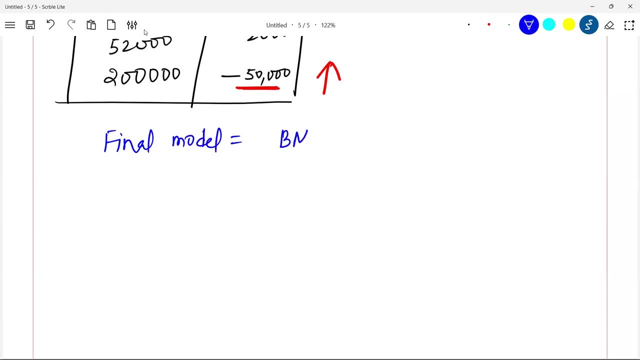 a combination of base model- i'm calling it the first model, okay, plus m1 plus m2, plus m3, plus so on and so forth. remember this: this is not a mathematical equation. this is just an indicative equation i'm giving you okay if you want to understand more mathematics behind it. 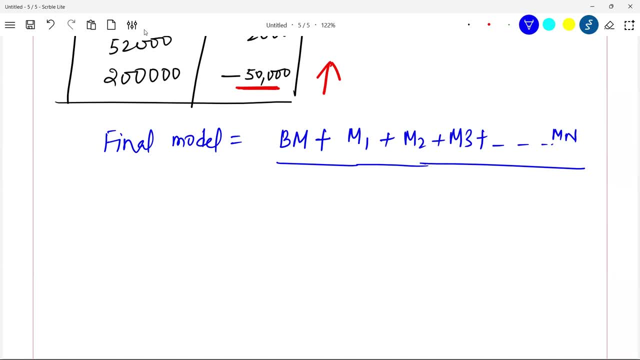 please go ahead and click on the link i'm giving you in the description. okay, and all these things will not have equal say in the final output. their say also will be different in the final output. for example, in random forest you saw all the models have equal say in the final. 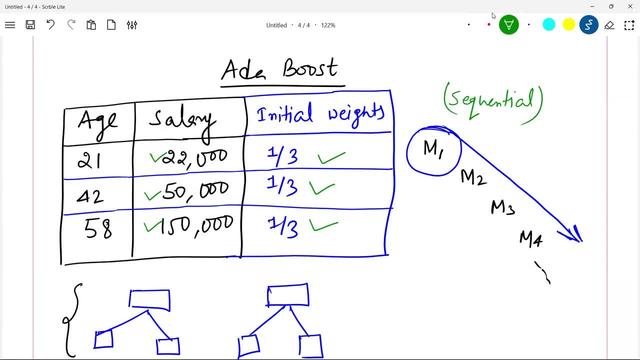 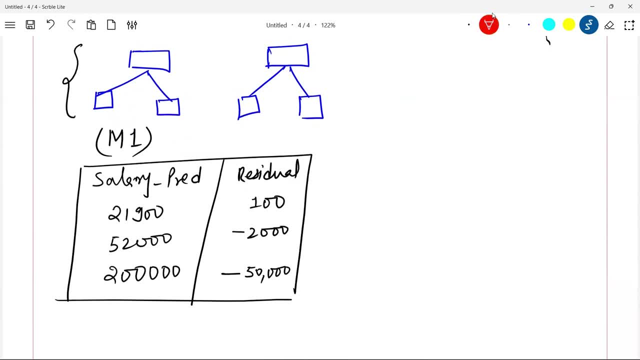 when the m2 is fitted right, these initial weights will be changed and more preference will be given to the observations where these residuals are more okay. i am repeating one more time, guys: m1 will predict this and then residuals or errors will come when the m2 is trained right. then the weights. 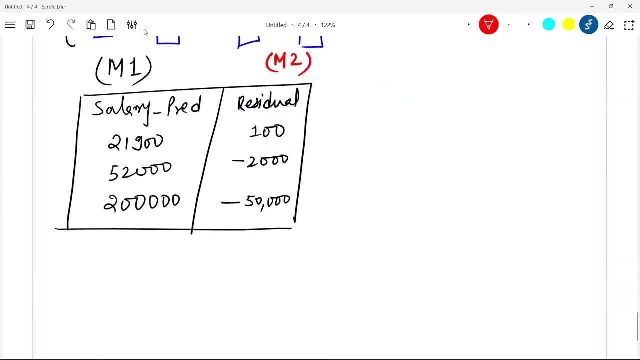 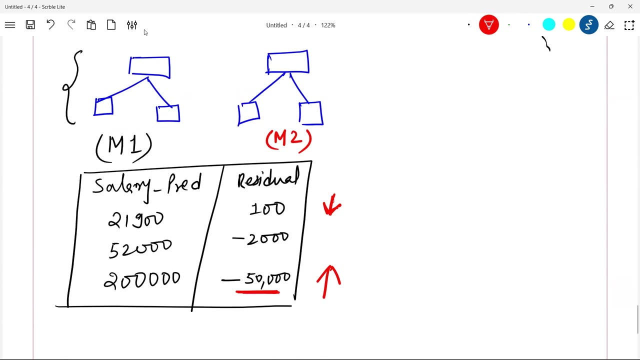 will not be same for all these three records. rather, weight will be increased for this because you are getting more errors here, and weight will be decreased for this because you are getting less error here. okay, and so on and so forth. m2 will come, compute, create the residual, then again weights will be adjusted. m3 will come. 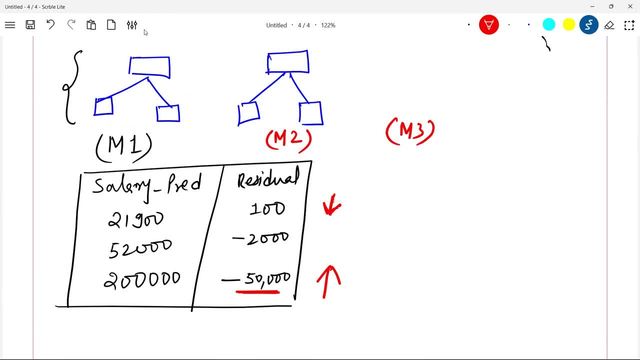 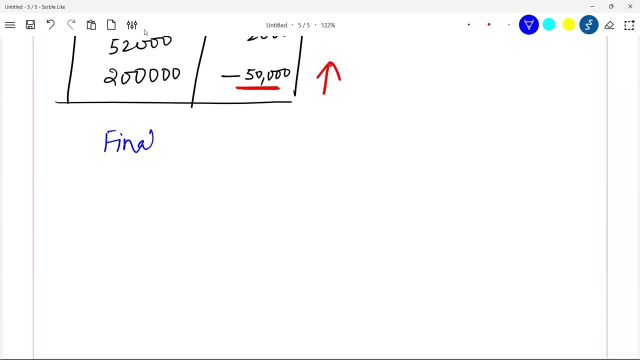 predict, residual will be calculated, weights will be adjusted and, finally, what you will get is a combination of what will be your final model. your final model will be a combination of base model- i'm calling it the first model, okay- plus m1, plus m2, plus m3, plus so on and so forth. remember this: this is not a mathematical equation. 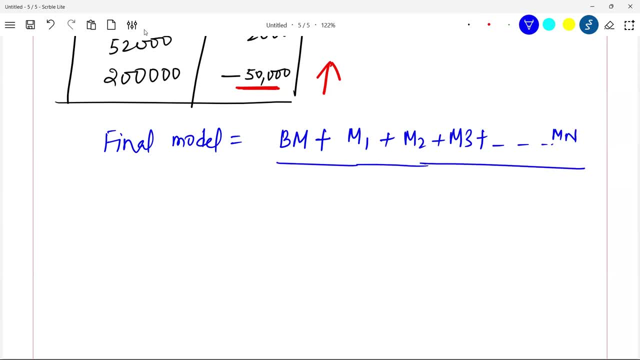 this is just an indicative equation i'm giving you. okay, if you want to understand more mathematics behind it, please go ahead and click on the link i'm giving you in the description. okay, and all these things will not have equal say in the final output. their say also will be different in the 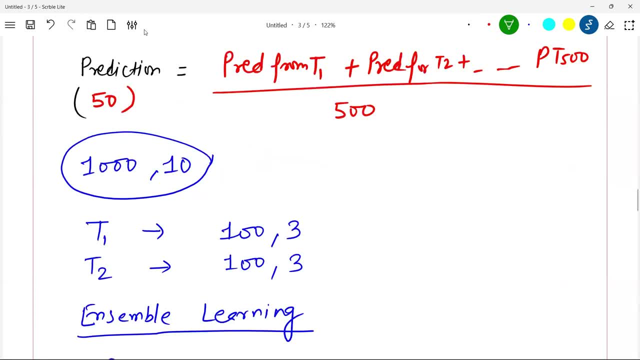 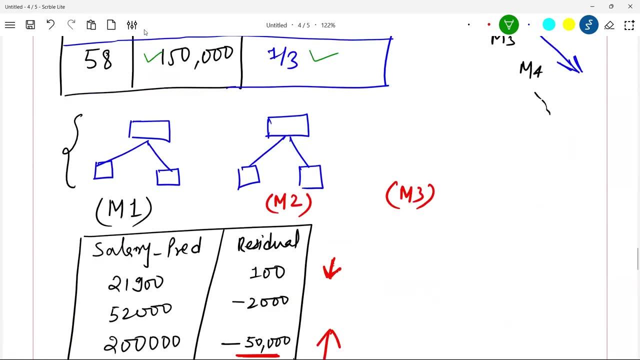 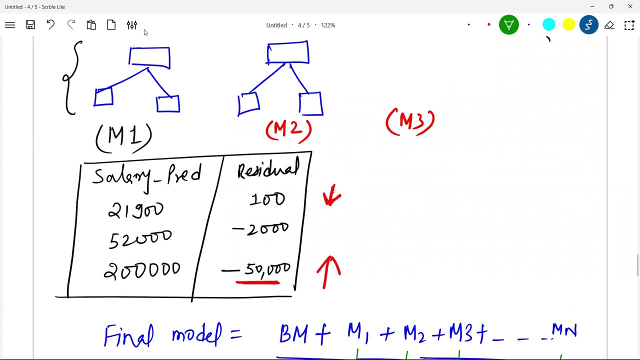 final output. for example, in random forest, you saw all the models have equal say in the final output. we are dividing by 500, okay, but here all these models will not have equal say, they will have unequal say. okay, let's move ahead to another. what is the pros and cons for this model? again this: 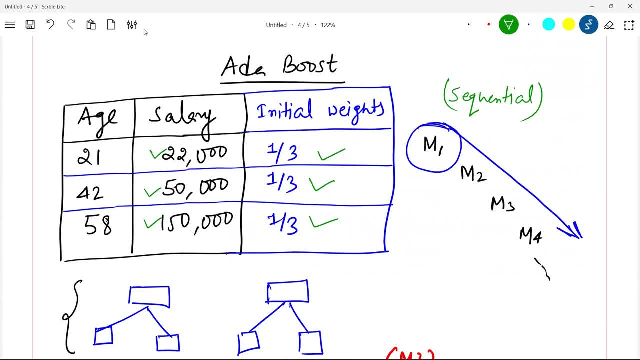 model will give you a may give you a better result than most of the models because it is adapting to the changes. but if you have a larger data side, it may it may need more resources to train and also it is a one kind of black box model. some kind of black box model means you don't have much. 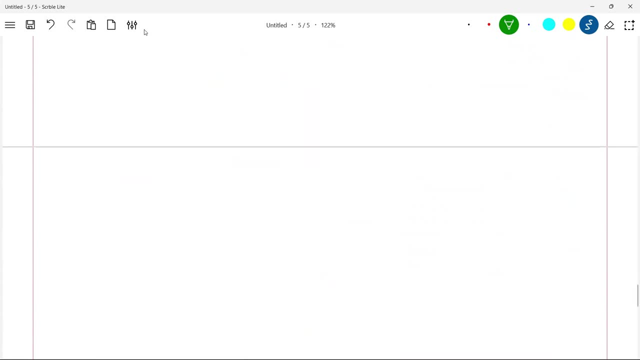 explainer. you don't have enough explainer. you don't have enough explainer. you don't have enough explainer of what is going on inside, apart from some hyper parameters. okay, let's move ahead to the last algorithm integration category, known as gradient boost. okay, what is the last algorithm integration? 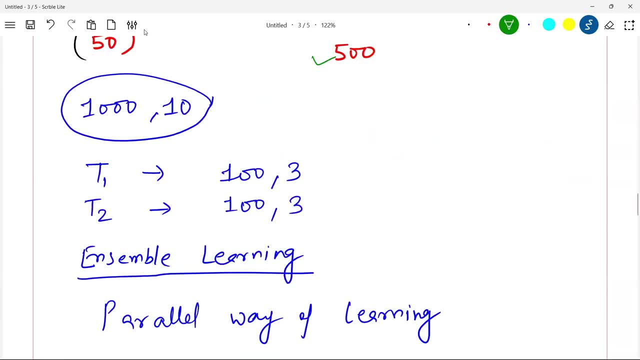 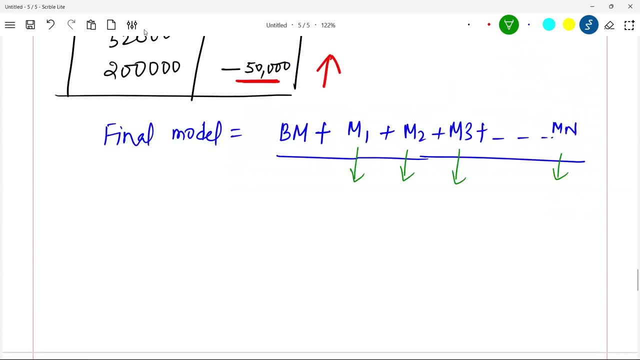 output we are dividing by 500. okay, but here all the levels in the final output are very similar to this. models will not have equal say. they will have an equal say. okay, let's move ahead to another. what is the pros and cons for this model? again, this model will give you a may, give you a better. 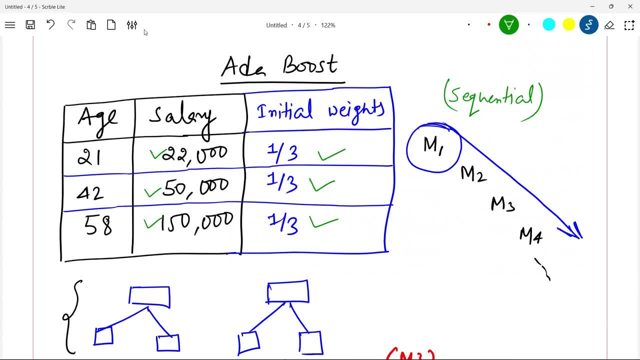 result than most of the models because it is adapting to the changes. but if you have a larger data side, it may it may need more resources to train and also it is a one kind of black box model. some kind of black box model means you don't have much explanation of what is going on inside. 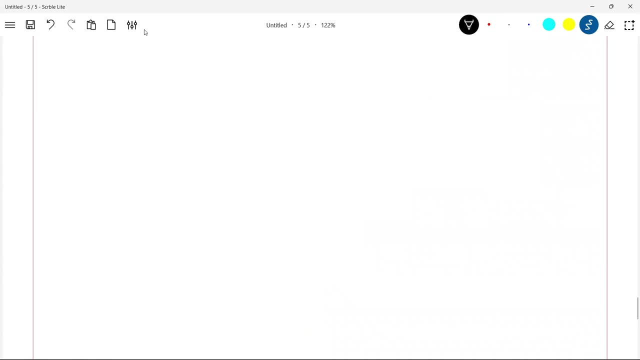 apart from some hyper parameters. okay, let's move ahead to the last algorithm integration category, known as gradient boost. okay, what is the last algorithm integration category? gradient boost. remember, guys, all these algorithms that i'm explaining you, i have not taken anything that is used less. all are used more, only okay. so i will take a simple data: age salary is 21 salary. 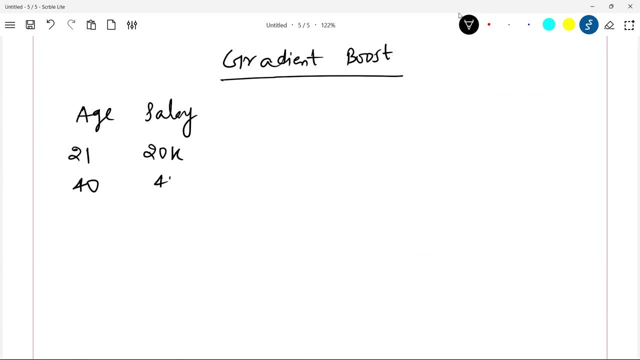 let's say 20k is 40 salaries. let's say 42k is 58 salaries. let's say 60k. this is your input data and you want to run a gradient boost on this. what will happen is: understand, guys, this is again a sequential learning, not a parallel learning. okay. 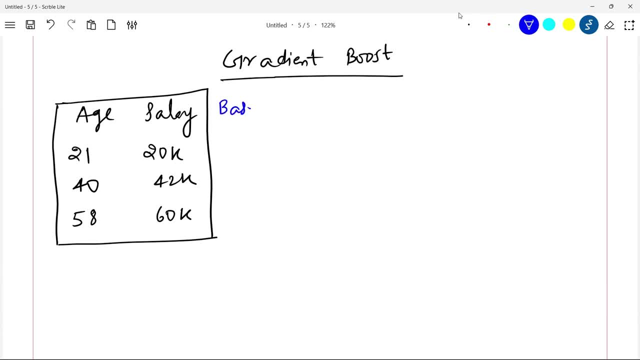 so there will be a base prediction for all these data. base prediction, okay, base prediction. what is the base prediction, guys? base prediction is nothing, but it's the kind of dumb model it will assume that for all these guys it will be an average of. you know all these three records. so what is the average of this? uh, 80 plus 42. 80 plus 42. 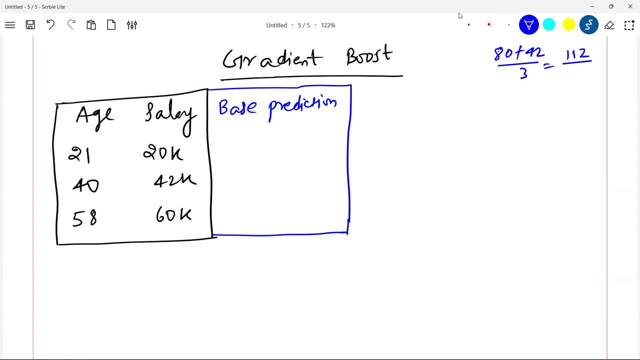 divided by three right, so two one. one, two right. let's assume, for simplicity, this is 36k, okay, so the base prediction will be put here: 36k, 36k, 36k. once the base prediction comes, then there will be a residual computed, okay, residual will be the difference between actual and 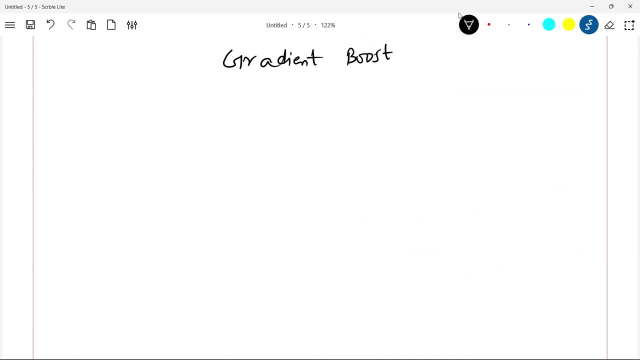 category: gradient boost. remember, guys, all these algorithms that i'm explaining you, i have not taken anything that is used less. all are used more, only okay. so i will take a simple data: age: salary is 21. salary, let's say 20k, is 40. salary is, let's say 42k. age 58: salary is, let's say, 60k. this is your input data and you want to. 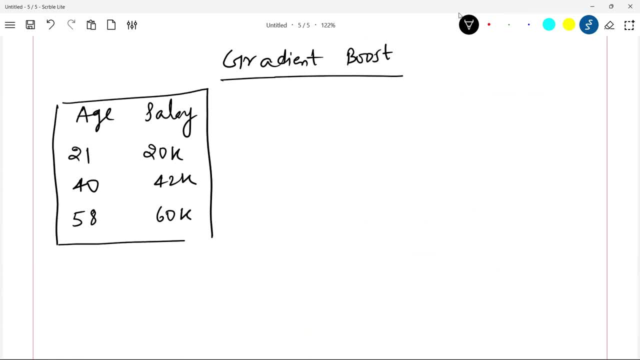 run a gradient boost on this. what will happen is: understand, guys, this is again a sequential learning, not a parallel learning. okay, so there will be a base prediction for all these data. base prediction, okay, base prediction. what is the base prediction, guys? base prediction is nothing, but it's the kind. 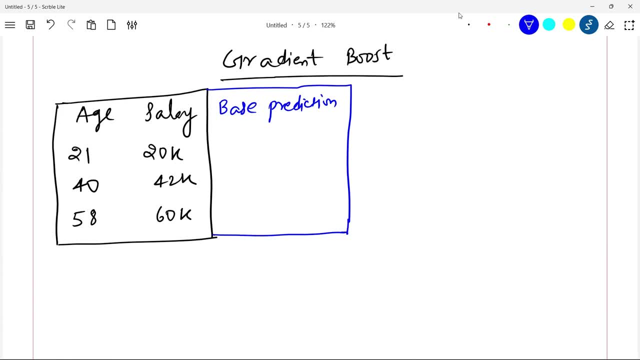 of dumb model. it will assume that for all these data, it will assume that it will assume that it will these guys. it will be a average of, you know, all these three records. so what is the average of this? 80 plus 42, 80 plus 42 divided by 3 right. so 2 1, 1, 2 right. let's assume, for simplicity, this is 36k. 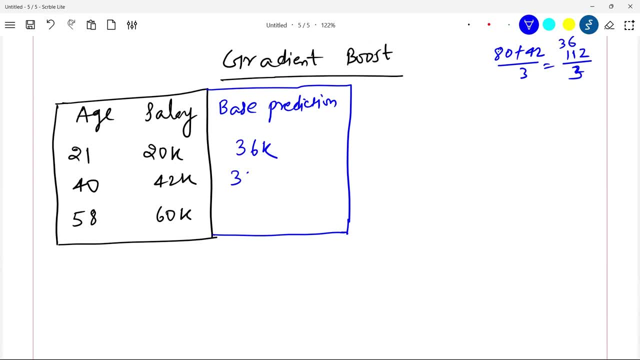 okay, so the base prediction will be put here: 36k, 36k, 36k. once the base prediction comes, then there will be a residual computed. okay, residual will be the difference between actual and predicted values. whatever these numbers are fine. now comes the interesting part: how gradient boost is different from ada boost or 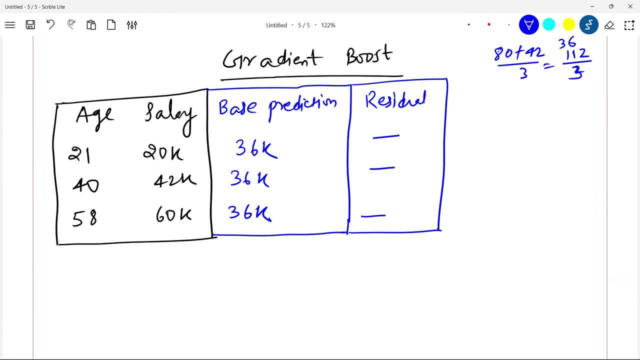 other algorithms. so what gradient boost will do is: it will try to fit a model on this residual, okay. it will try to fit a model on this residual and try to minimize these residuals. so that will be called as a base model, okay. and then there will be 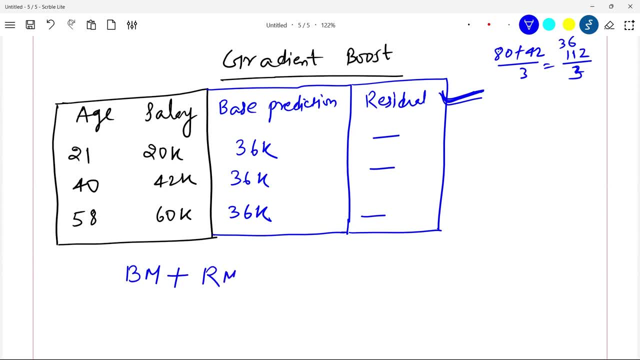 next model. you can call it residual model one, okay. and then there will be a next model- you can call it residual model two, and so on and so forth. okay, so what will happen is residuals will be computed and then, whatever the residual comes based on that base prediction will be updated. 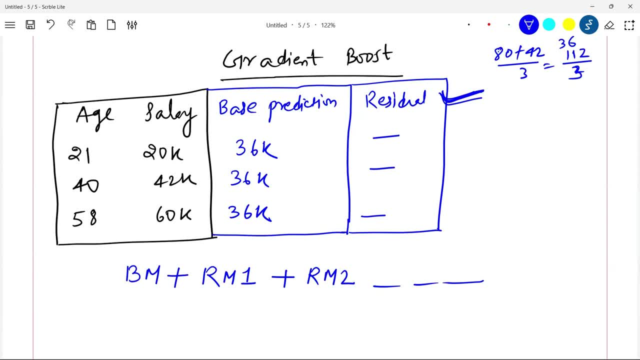 so, for example, let's say your residual here is how much- 20 minus 36 minus 16 is your residual right? so these will act as a independent callings column and this residual will act as a target column. and then let's say in the prediction: 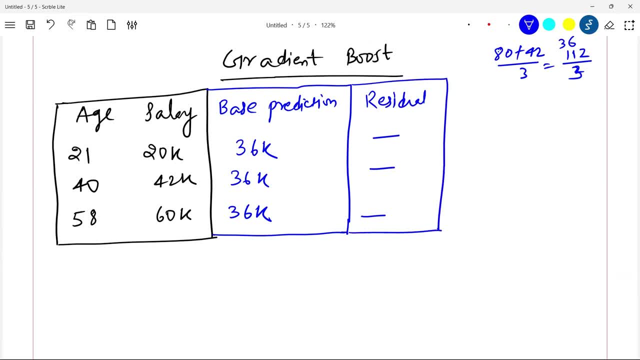 predicted values. whatever these numbers are fine. now comes the interesting part: how gradient boost is different from ada boost or other algorithms. so what gradient boost will do is: it will try to fit a model on this residual. okay, it will try to fit a model on this residual and try to minimize these. 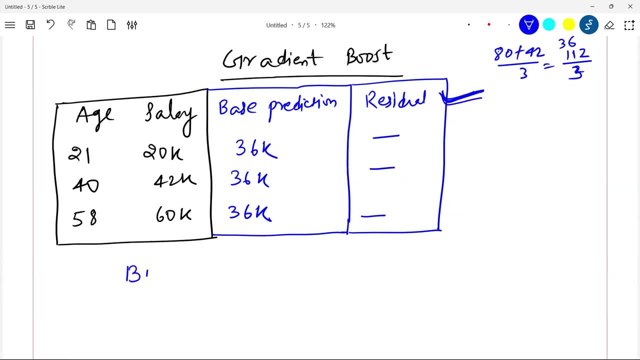 residuals. so that will be called as a base model, okay. and then there will be next model. you can call it residual model 1, okay. and then there will be a next model, you can call it residual model 2, and so on and so forth. okay, so what will happen is residuals will be computed. 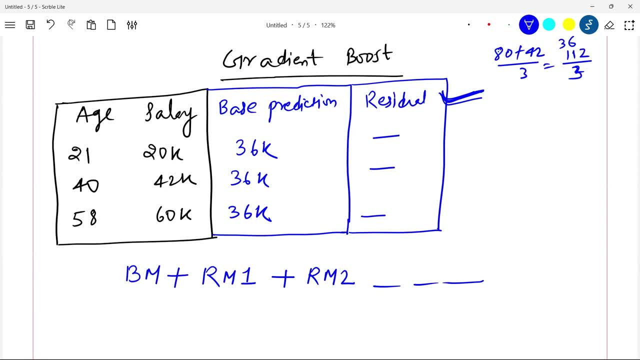 and then, whatever the residual comes, based on that base, prediction will be updated. so, for example, let's say your residual here is how much- 20 minus 36 minus 16 is your residual right? so these will act as an independent column and this residual will act as a target. 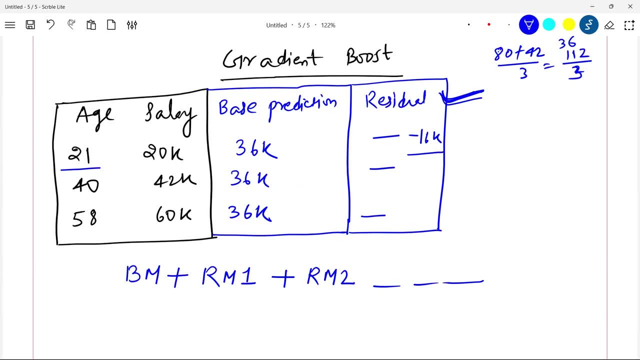 column and then let's say in the prediction, this minus 16 is, is comes as, let's say, minus 10. so what will happen is this base prediction will get updated by this. this base prediction will get updated again. it's a complicated model if you want to understand more details. 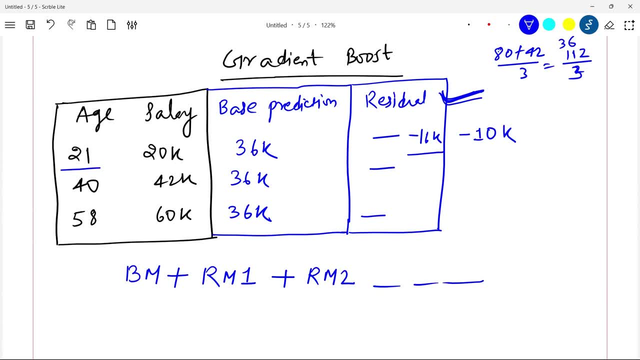 there are links in the description. please click on that. it will be very clear to you, okay? So what will happen? base model plus residual model 1 plus residual model 2, so on and so forth, and there will be some parameters which will assign weight to all these models. so 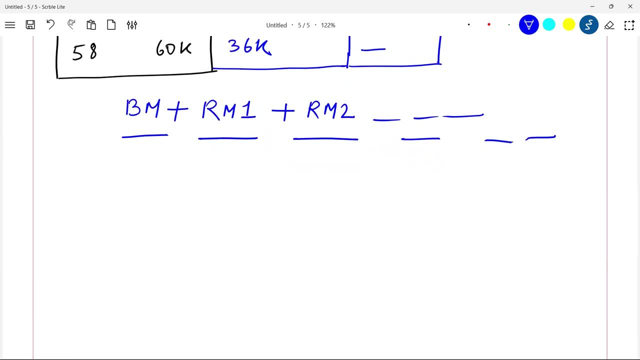 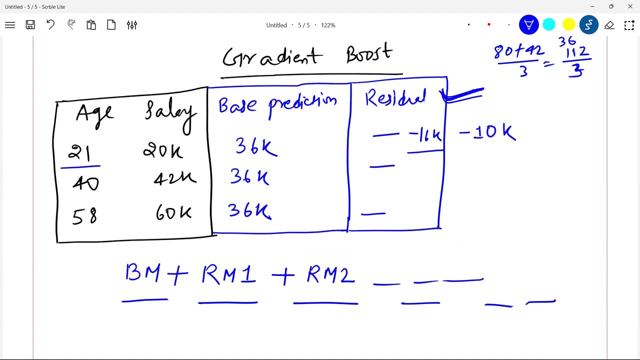 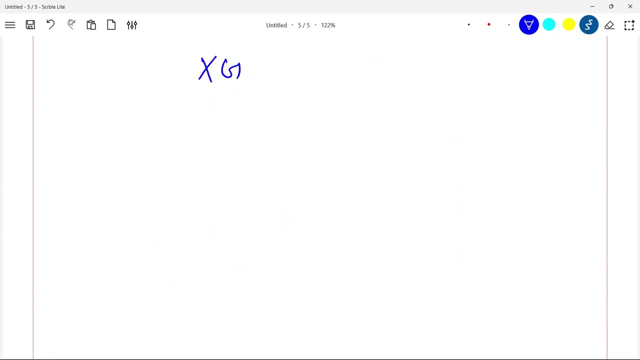 as I say, all these models will not have a equal vote in the final output. there will be a different votes in this. fine, so this is about gradient boost, one of the famous algorithm for winning Kaggle competitions and most of the things. so gradient boost. and there is another variant of gradient boost known as XGB- extreme gradient boost, please. 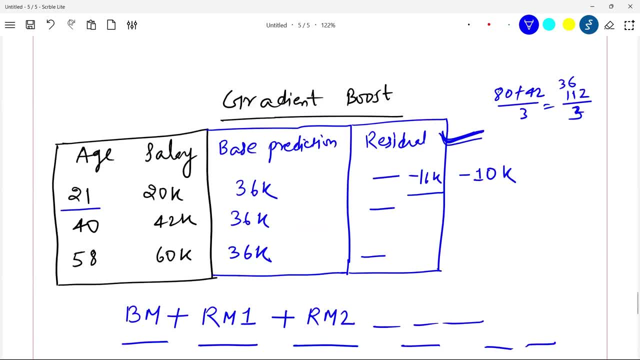 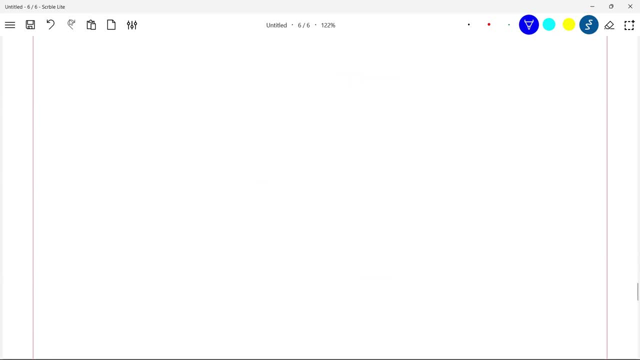 go ahead and read about this algorithm. Please go ahead and read about this algorithm, guys I'm not covering, because there is a slight difference between gradient boost and XGB. you can read about that as well. fine, let's move ahead to the second category of algorithms. 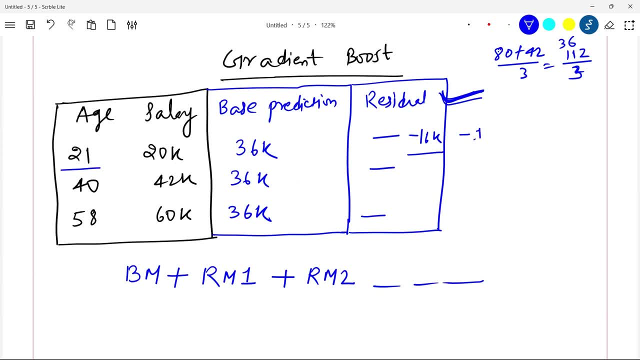 this minus 16 is, is comes as, let's say, minus 10. so what will happen is this base prediction will get updated by this. this base prediction will get updated again. it's a complicated model. if you want to understand more details, there are links in the description, please. 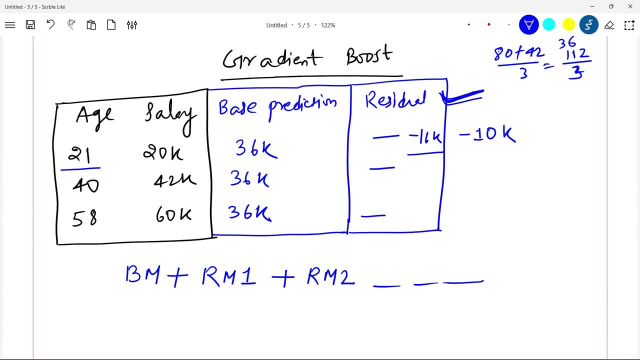 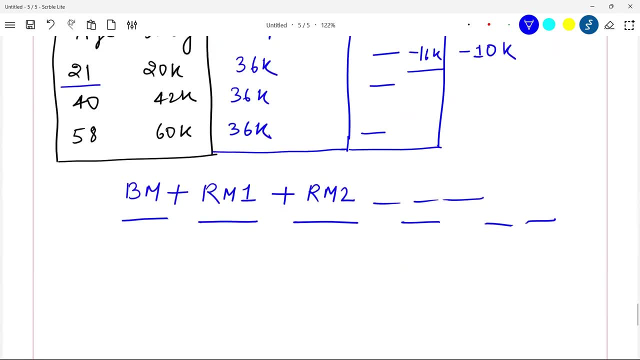 click on that, it will be very clear to you. okay, so what will happen? base model plus residual model 1 plus residual model 2, so on and so forth, and there will be some parameters which will assign weight to all these models. so, as I say, all these models will not have an 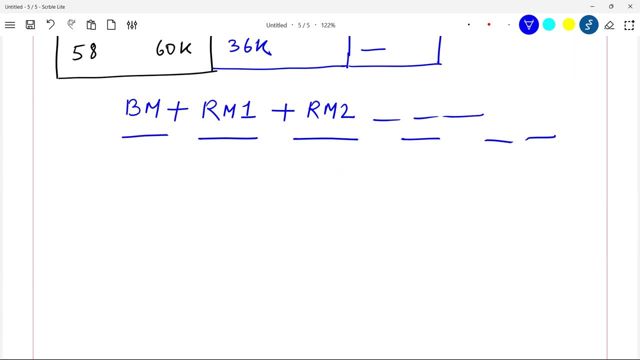 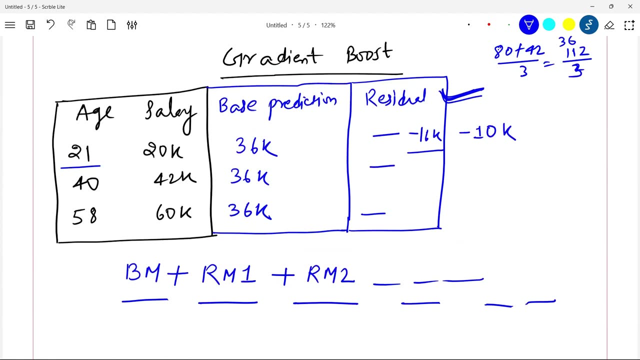 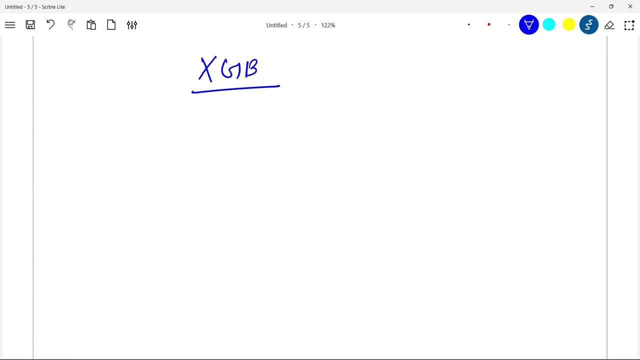 equal vote in the final output. there will be a different votes in this. fine. so this is about gradient boost, one of the famous algorithm for winning Kaggle competitions and most of the things. so gradient boost. and there is another variant of gradient boost known as xgb, extreme gradient boost. please go ahead and read about this algorithm, guys. 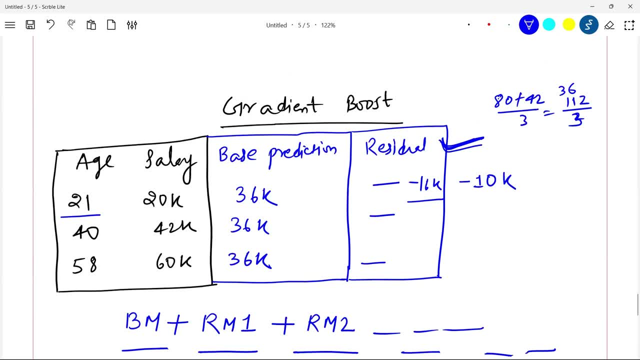 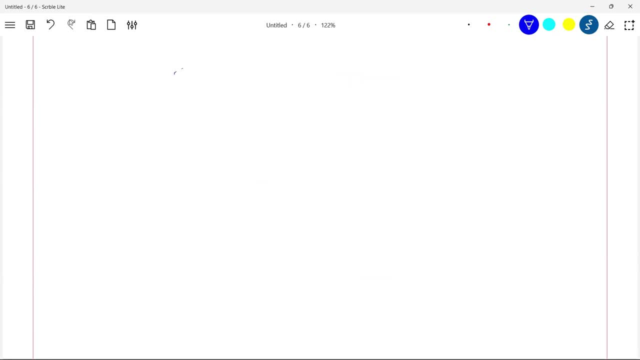 I'm not covering, because there is a slight difference between gradient boost and xgb. you can read about that as well. fine, let's move ahead to the second category of algorithms, known as classification algorithms. so in classification algorithms, the first algorithm that i'm going to cover is logistic regression. now very, very important guys, please pay attention. 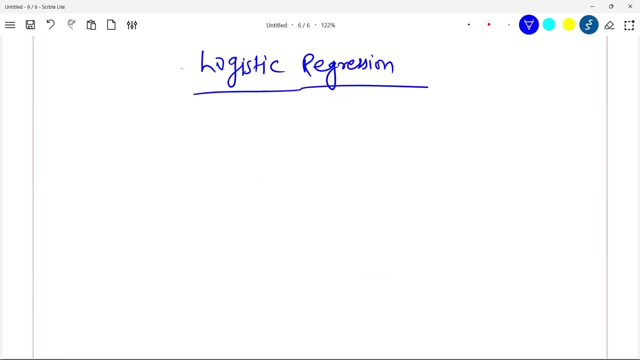 here and try to understand how logistic regression is going to work for any given scenario. it's a mathematical model, hence it is important for you to understand. okay, suppose this is an employee data and you have 21, 22k, whether the employee leaves the organization or does not leave the organization. 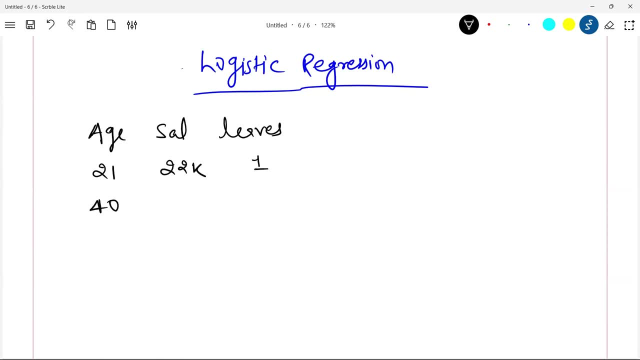 just i'm saying 1, 0, okay. and then 40 year guy makes, let's say 42k, leaves 0, no. 58 year guy makes, let's say 60k, just for example, leaves no 1. so this is a classification problem where we are trying to 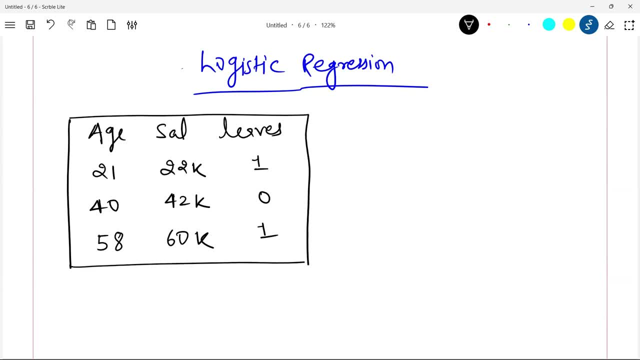 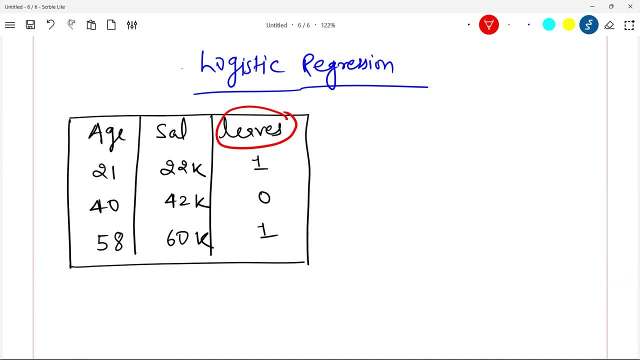 the last column that you see is your target column. this type of problem is called a classification problem, because what this? what the objective of this model is tomorrow? i give you age of the employee, for example 31. salary of the employee, for example, 34k, and i ask: 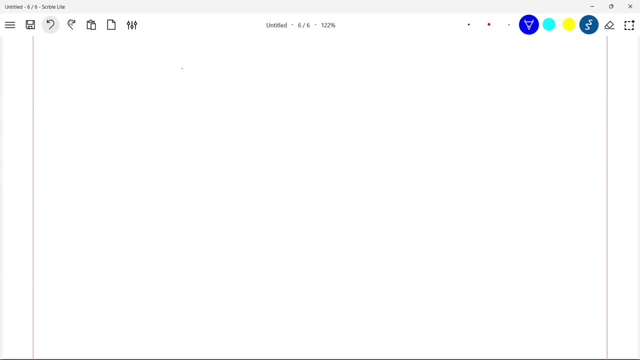 known as classification algorithms. so in classification algorithms, the first algorithm that I'm going to cover is logistic regression. now, very, very important guys, please pay attention here and try to understand how logistic regression is going to work for any given scenario. it's a mathematical model, hence it is important for you to understand. 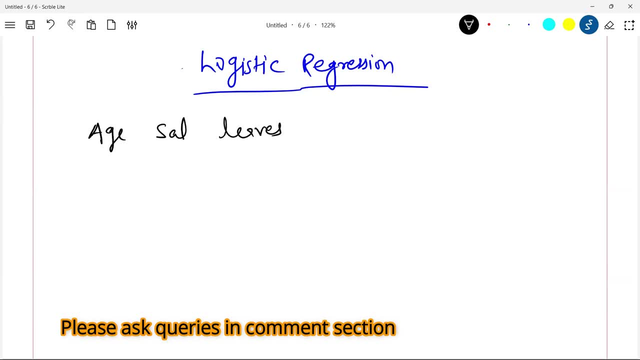 how logistic regression is going to work for any given scenario. it's a mathematical model, hence it is important for you to understand. okay, suppose this is an employee data and you have 21, 22 K, whether the employee leaves the organization or does not leave the organization. just I'm saying 1, 0, okay, and then 40 year. 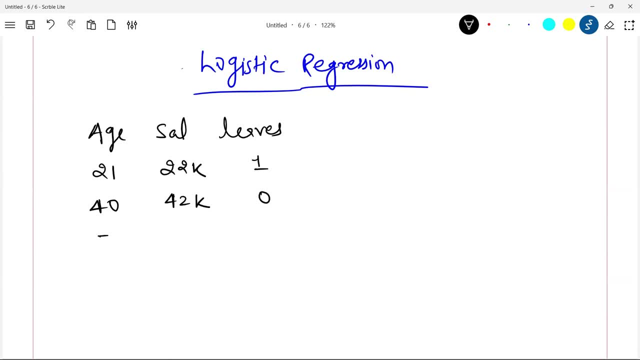 guy makes, let's say, 42 K, leaves 0. no 58 year guy makes, let's say, 60 K, just for example, leaves no one. so this is a classification problem, where we are trying to predict whether a employee will leave the organization or does not leave the organization. the last one. 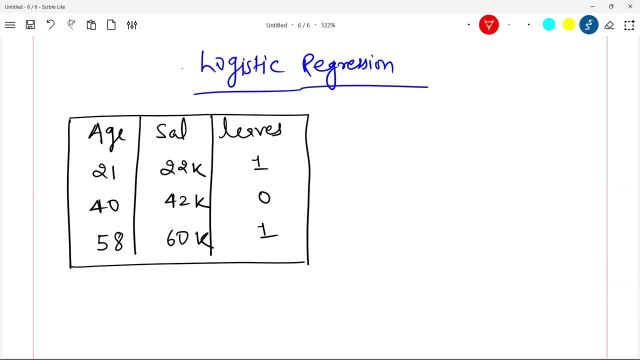 last column that you see is your target column. the last column that you see is your target column. this type of problem is called a classification problem, because what this, what the objective of this model is tomorrow? I give you age of the employee, for example 31. salary of the. 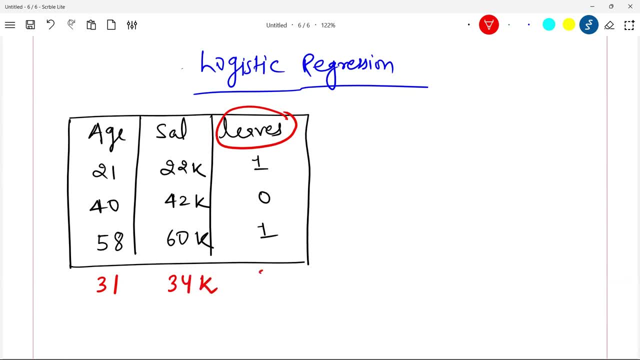 employee, for example, 34 K, and I asked to the model: hey, will the guy leave or not leave the organization? okay, so this is a classification problem, how logistic regression will take. this problem is we have we have to understand some mathematical concepts here. so if you see, here the target column is 1, 0 only. so that is either 1 or 0, 1 or 0. 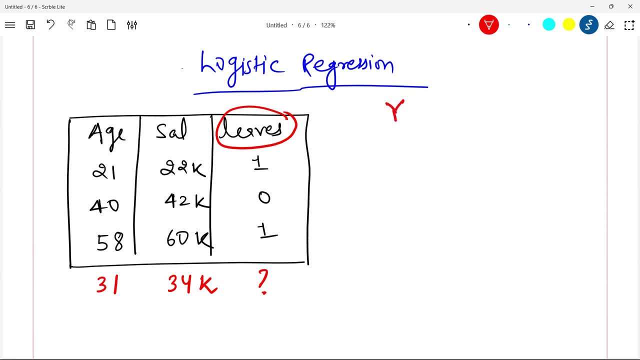 okay, so which means that Y, which is our target, can be understand. this is very important concept. guys, can be either 0 or 1. it cannot be anything else. your target cannot be anything else apart from 0 or 1, but your age and salary can take any real number. 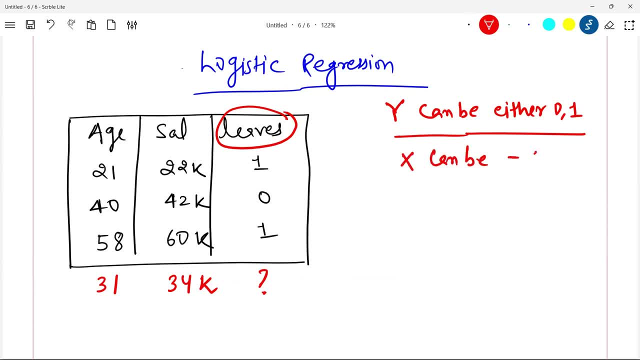 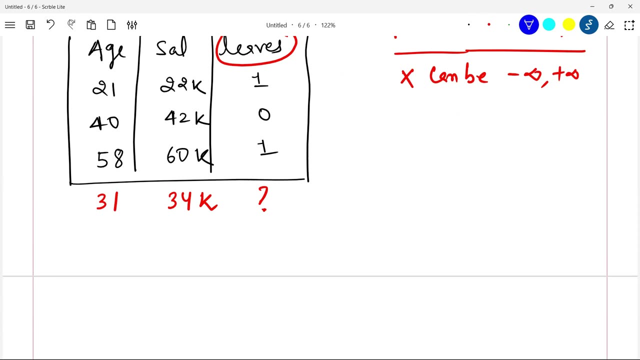 X can be Any value between minus infinity to plus infinity. right, so X can be any value between minus infinity to plus infinity. Y can be only 0 or 1. okay, so what we have to understand here is we have to somehow create a relation that will enable us to predict Y given X. okay, the 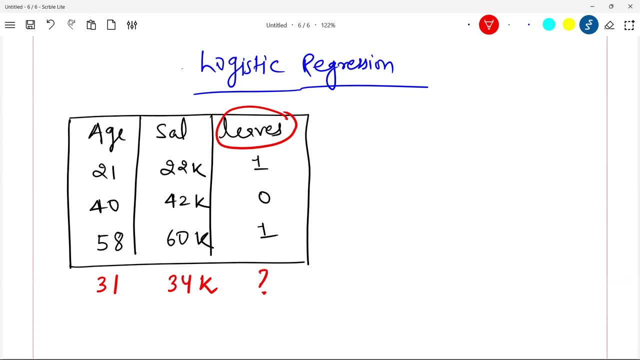 to the model: hey, will the guy leave or not leave the organization? okay, so this is a classification problem, how logistic regression will take. this problem is we. we have to understand some mathematical concepts here. so if you see, here the target column is one, zero only. so that is either one or zero. one or zero, okay. so which means that y, which is our. 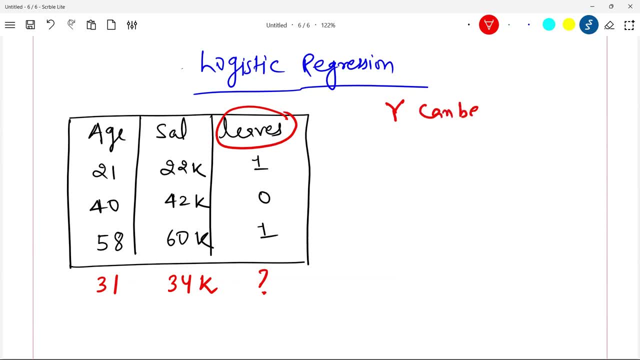 target can be understand. this is very important concept. guys can be either zero or one. it cannot be anything else. your target cannot be anything else apart from zero or one, but your age and salary can take any real number. x can be any value between minus infinity to plus infinity level. 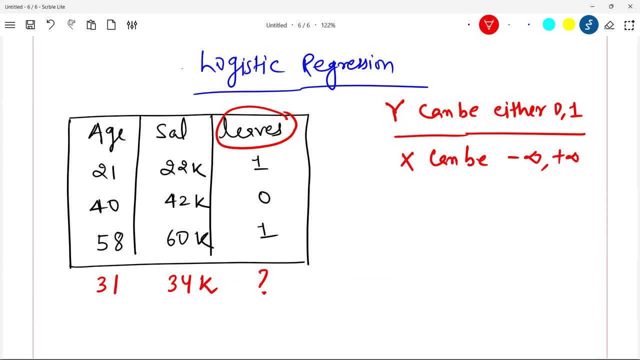 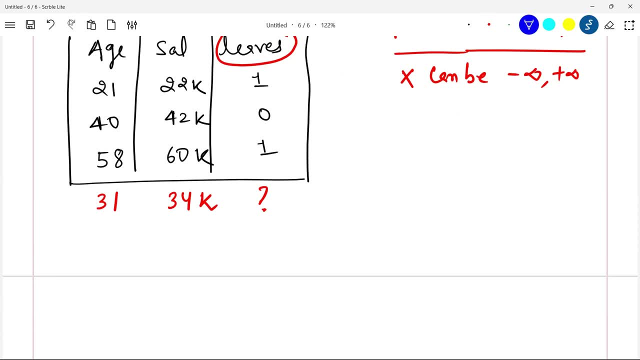 right, so x can be any value between minus infinity to plus infinity. y can be only zero or one. okay, so what we have to understand here is we have to somehow create a relation that will enable us to predict y given x. okay, the problem here is on the left hand side. we have minus infinity to plus. 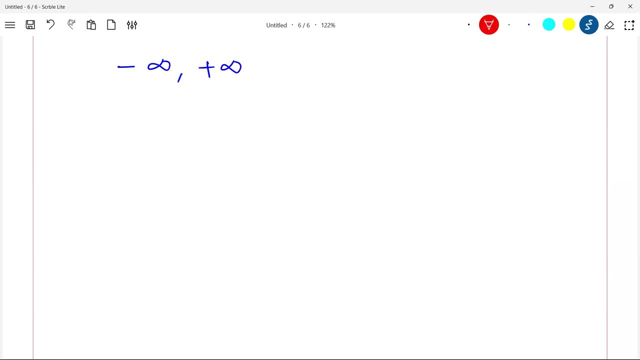 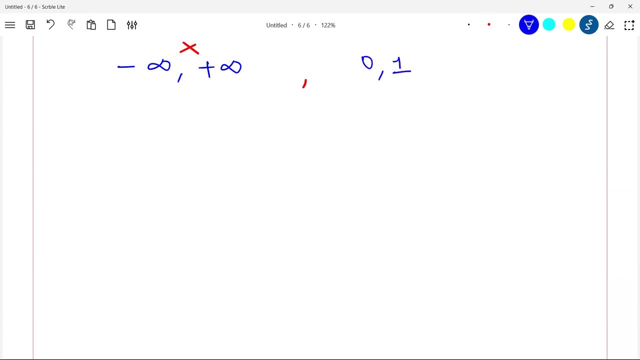 to generalize the data in order to write it, but i am not gonna write求, i am not. let you see, the values can be only 0 to 1, zero or 1, not 0 to 1. okay, so what we do is we do not directly predict y. 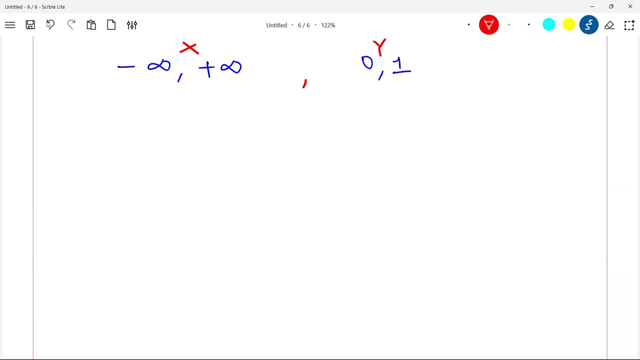 rather, we predict something else. what is that? something else that we predict? so, in place of predicting y, we predict probabilities. okay, probabilities of an observation falling in y, probabilities l i t i e s okay. so what we will do is we will predict probabilities, then the range. 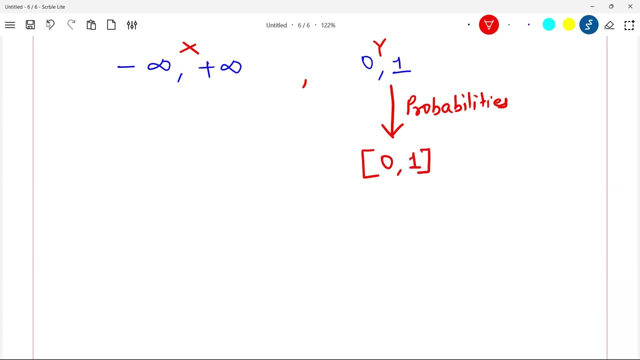 will be 0 to 1. as you know, probability can take the range between 0 to 1. okay, now, this range is also not what we are looking for: minus infinity to plus infinity. so what we will do is we will do one more transformation and we will make this as a odds. so what is the range of odds? 0 to 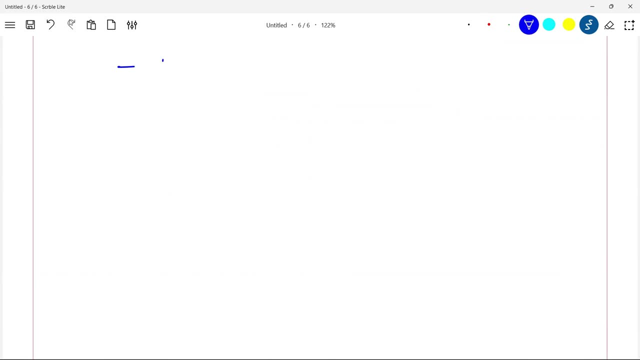 problem here is: on the left hand side we have minus infinity to plus infinity range, that is X range. okay, so I will write here X. X means independent features. on the right hand side, your values can be only 0 to 1, 0 or 1, not 0 to 1. okay, so what we do is we do not directly predict Y, rather we predict 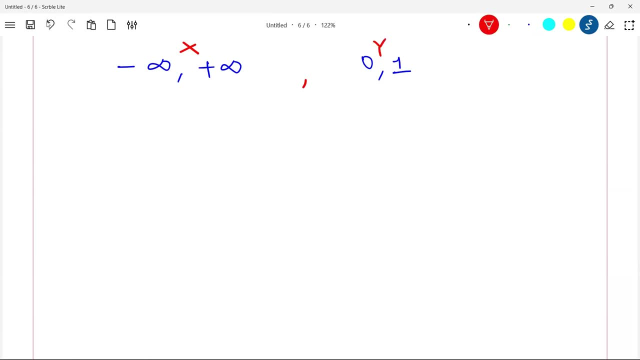 something else. what is that? something else that we predict. so, in place of predicting Y, we predict probabilities. okay, probabilities of an observation falling in Y, probabilities LITIS. okay, So what we will do is we will predict probabilities. then the range will be 0 to 1, as you know. probability. 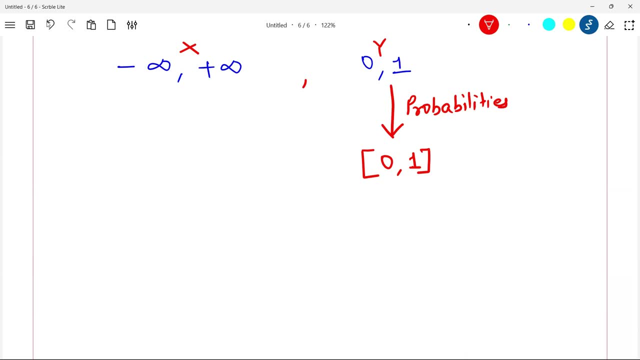 can take the range between 0 to 1. okay. now, this range is also not what we are looking for: minus infinity to plus infinity. so what we will do is we will do one more transformation and we will make this as a odds. so what is the range of odds? 0 to infinity, okay, but still. 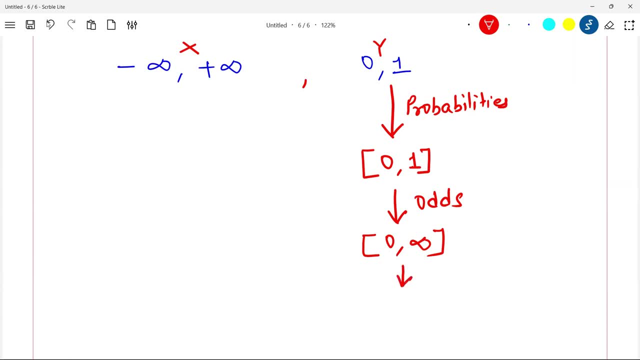 we are not minus infinity to plus infinity range. so what we will do is we will take log of odds, Log of odds, okay, and then the range will become minus infinity to plus infinity. how your equation will look like here is when you say: log of odds, right. so on the right hand side it will 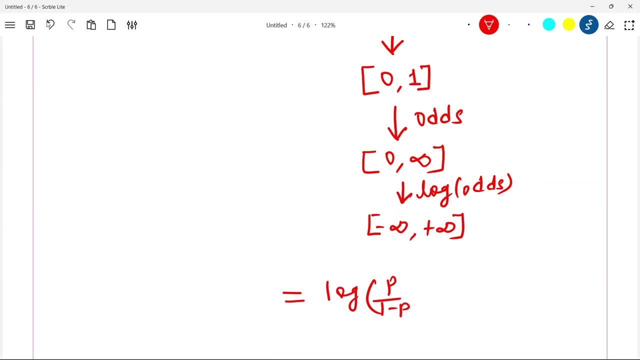 be log of P by 1 minus P. okay, on the left hand side you will have beta naught plus beta 1 X 1 plus so on and so forth. okay, this equation that you see in front of you now, it's called a base equation for the logistic regression. now one important concept to understand here. 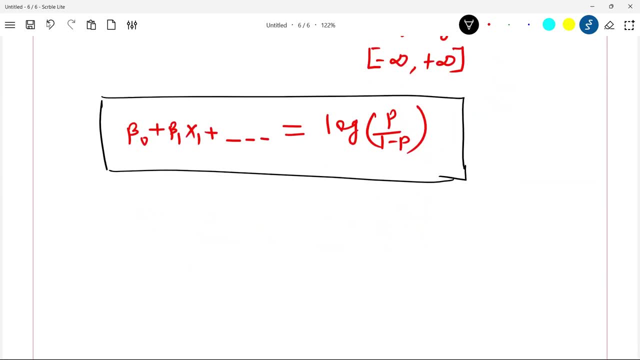 guys, this is a logit function. okay, and inverse of logit function. each sigmoid function: okay, support. suppose you take the inverse of this or sigmoid of this. so what will happen is if you apply sigmoid both sides. so if you don't know what is sigmoid function, then sigmoid. 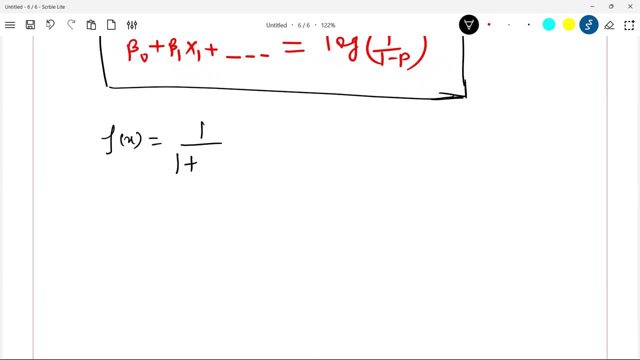 function fx looks like this: 1 by 1 plus e to the power minus X. this is your sigmoid function. So on xy plane how it will look like is this: suppose this is your 0, this is your 1 and this is your 0.5. okay, so sigmoid will look like this. so it will always be between 0 to 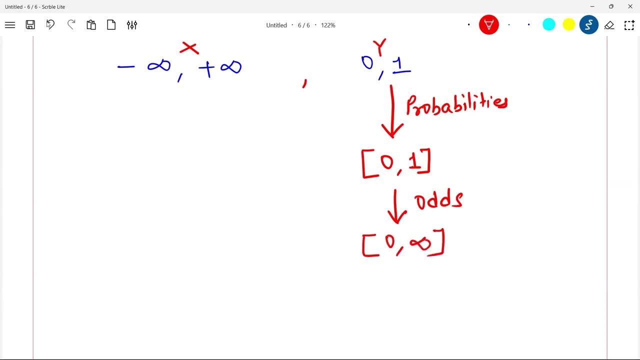 infinity okay, but still we are not minus infinity to plus infinity range. so what we will do is we will take log of odds okay, log of odds okay, and then the range will become minus infinity to plus infinity. how your equation will look like here is when you say: log of odds, right. 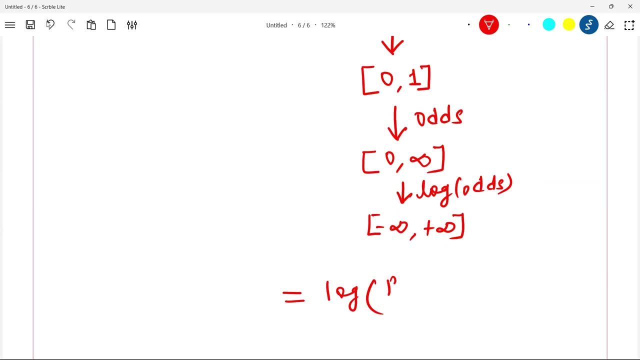 so on the right hand side, it will be log of p by 1 minus p. okay. on the left hand side, you will have beta naught plus plus beta 1 x1 plus so on and so forth. okay, this equation that you see in front of you now. 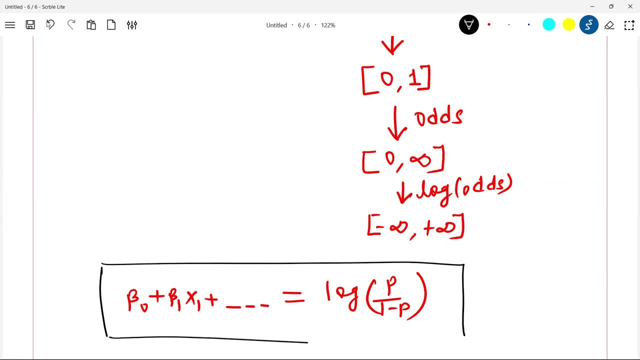 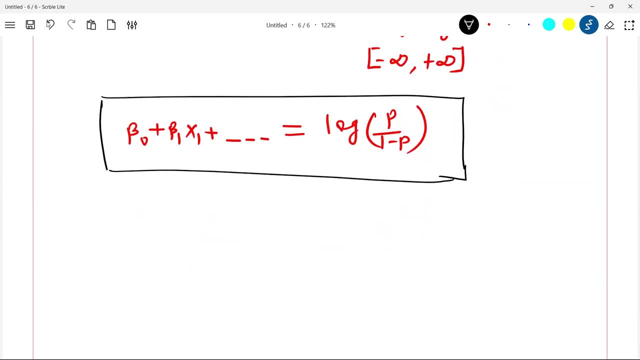 is called a base equation for the logistic regression. now one important concept to understand here, guys: this is a logit function- okay, and inverse of logit function is sigmoid function. okay, support, suppose you take the inverse of this or sigmoid of this. so what will happen is if you 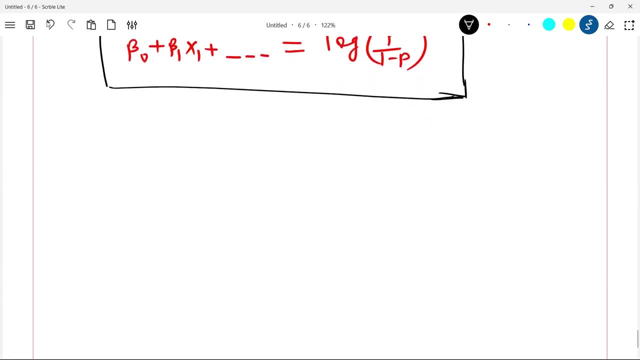 apply sigmoid both sides. so if you don't know what is sigmoid function, then sigmoid function fx looks like this: 1 by 1 plus e to the power minus x. this is your sigmoid function on xy plane. how it will look like is this: suppose this is your 0, this is your 1 and this is your 0.5. okay, 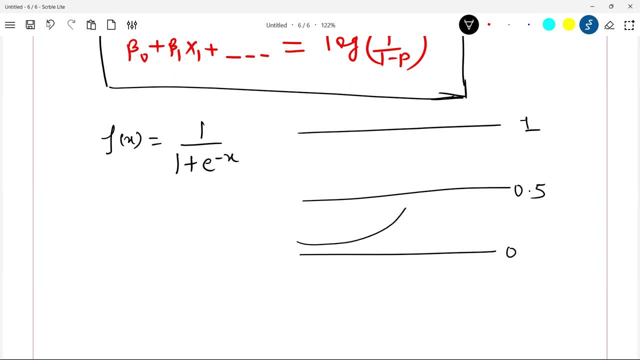 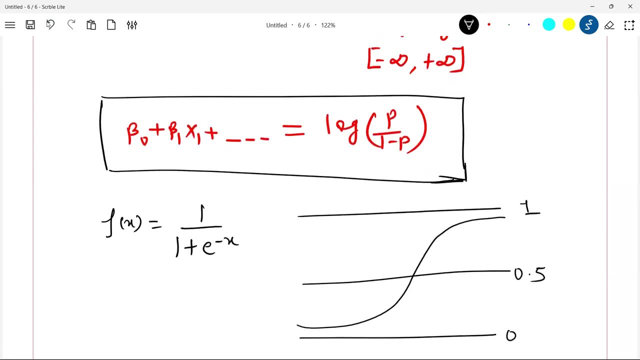 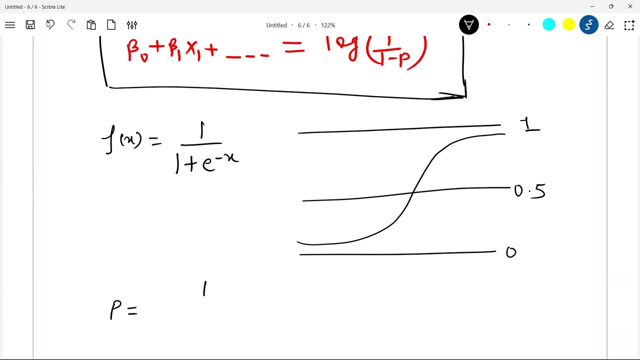 so sigmoid will look like this. so it will always be between 0 to 1. okay, so your logistic regression: this equation will be changed in the form of a logistic regression and this equation will be changed in the form of a logistic regression of sigmoid function. so your fx or p: okay, p will look like if you take, if you take, sigmoid on both. 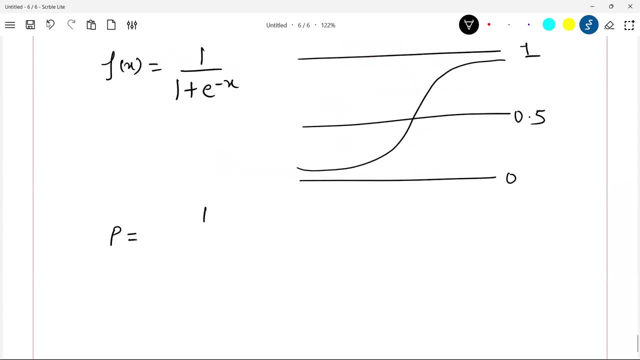 sides right then on the right hand side you will just have p and here you will have 1 by 1 plus e to the power, minus beta 0, plus beta 1 x1. okay, remember guys, this equation is equation 1 and this equation is equation 2. both the equations are same. the difference is: 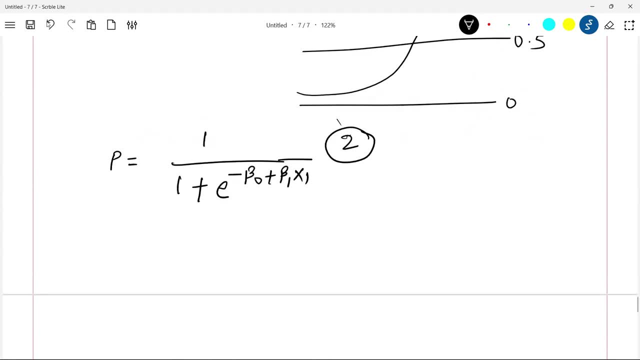 this is a logit equation and this is a sigmoid equation. okay, now take it. if you, if you take a inverse of logit, that is nothing but sigmoid. okay, understand this carefully. and now this equation, from our example, how it can be written, is: 1 by 1 plus e to the power, minus beta 0 plus beta 1. 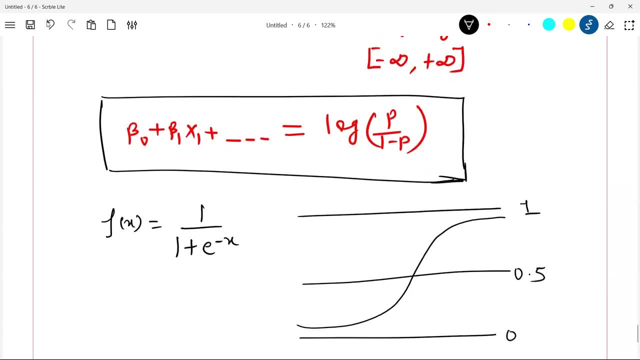 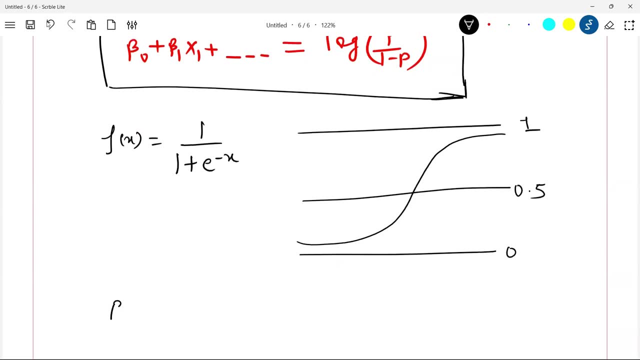 1. okay, so your logistic regression. this equation will be changed in the form of sigmoid function. so your fx or P, okay, P will look like if you take. if you take sigmoid on both sides right, then on the right hand side you will just have P. 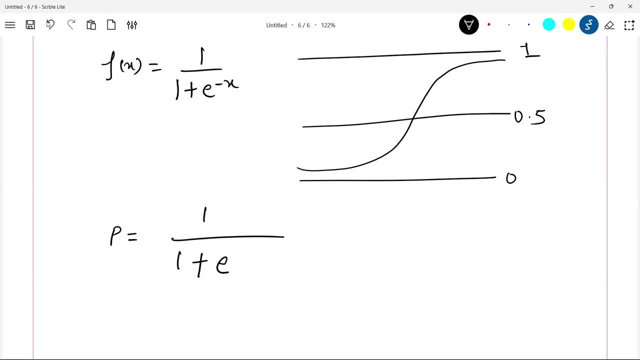 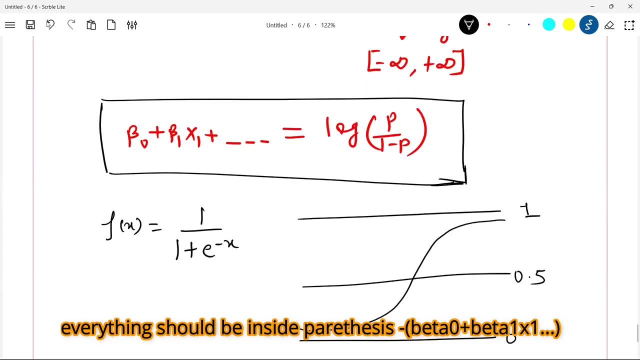 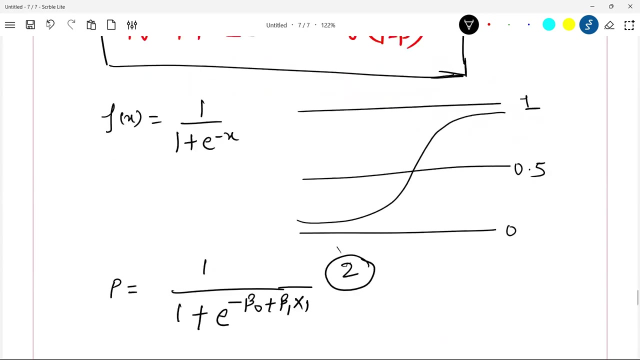 and here you will have 1 by 1 plus e to the power, minus beta 0, plus beta 1 X 1. okay, remember guys, this equation is equation 1 and this equation is equation 2. both the equations are same. the difference is this is a logit equation and this is a sigmoid equation. okay, 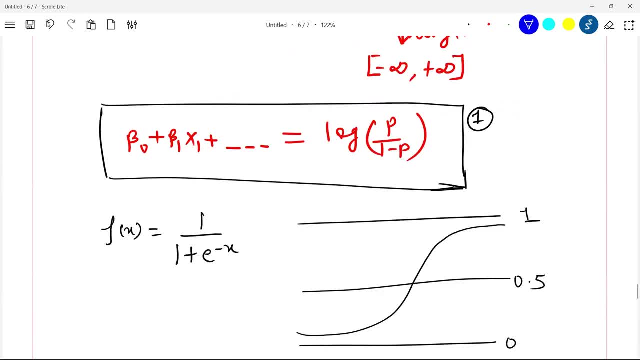 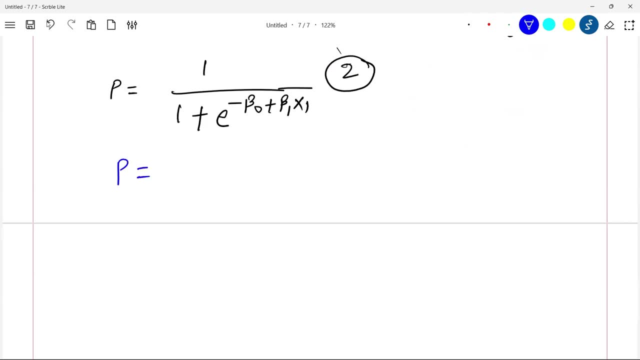 now take it. if you, if you take a inverse of logit, that is nothing but sigmoid. okay, understand this carefully. And now this equation from our example- how it can be written- is: 1 by 1 plus e to the power, minus beta 0, plus beta 1 into age, okay, plus beta 2 into salary. this is nothing but. 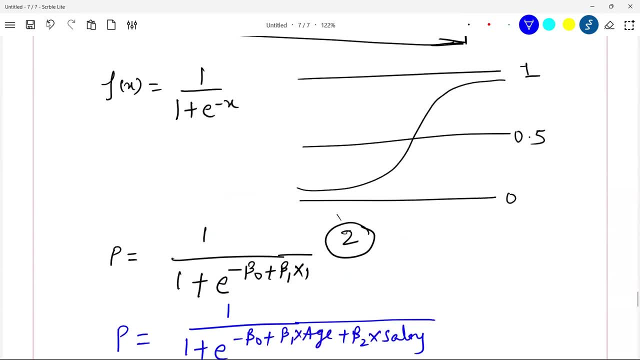 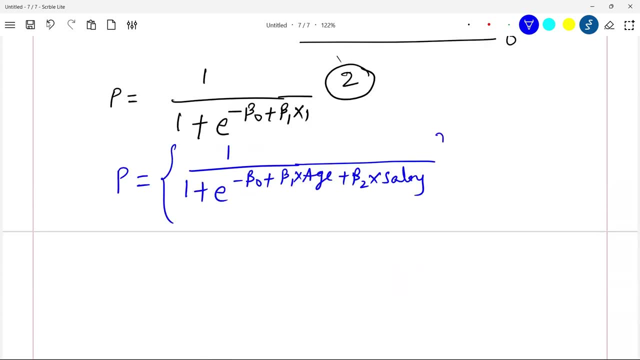 your logistic regression equation. okay, and, as you know, as I told you, this is a sigmoid function, so the output of what you see here, output of this, will always be between 0 to 1, which means you can get a probability and then you can say that, based on this probability, 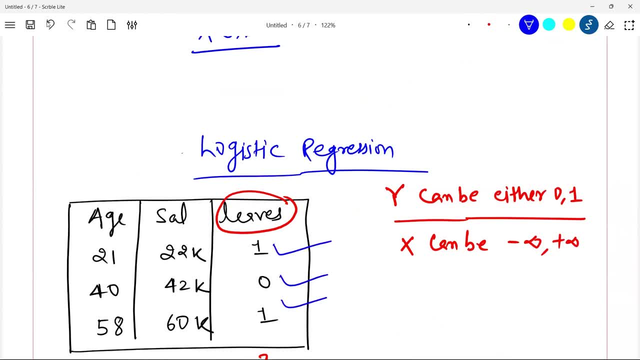 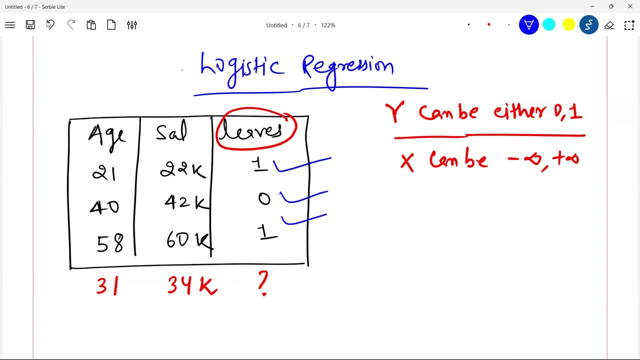 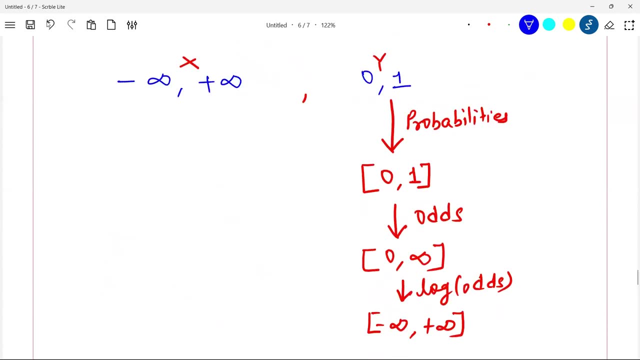 I can say whether the employee leaves or does not leave. okay, logistic regression is again a very important and not easy to understand concept. okay, so, as you can see, we are modeling a categorical variable against real numbers, hence we need to do certain transformations. these are the transformations that we need to do and how it relates to the probability. 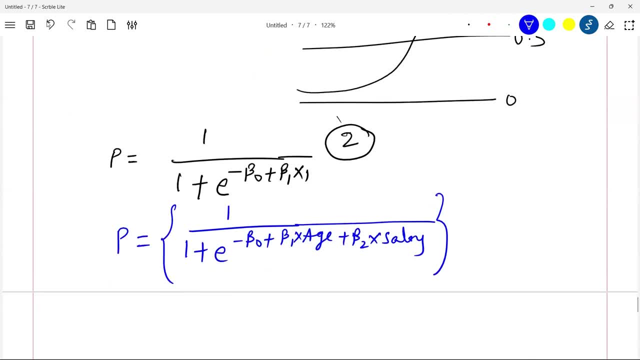 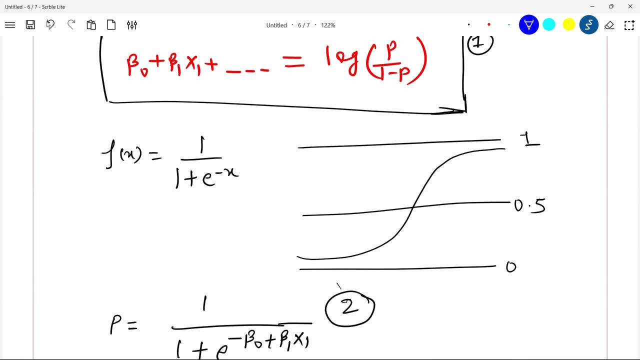 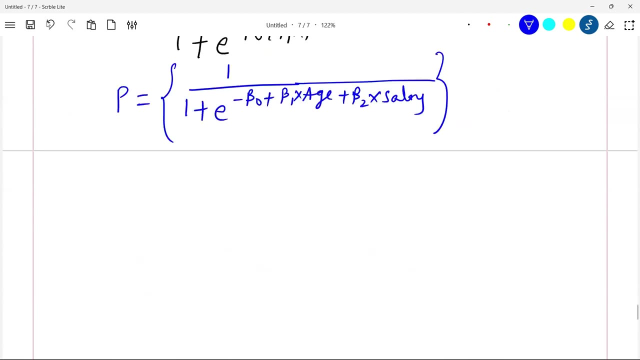 I just explained. you know okay Pros and Cons. Mathematical model, not very difficult to understand. cons: it again assumes a lot of things about the data which may or may not be correct. hence it may not give a great result all the time, okay, but very famous and very important algorithm to understand. next algorithm: 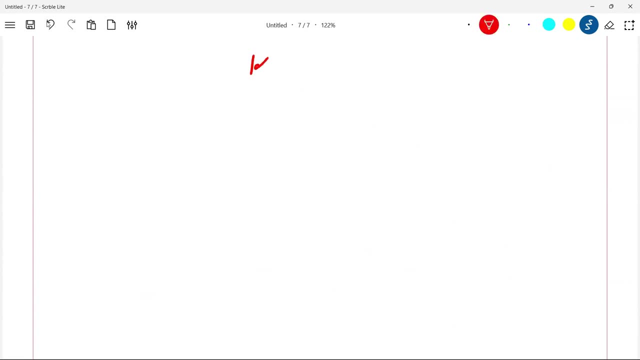 in the category, in the classification category, one simple one I want to cover here that is known as Kearney-Arrest-Neighbor. okay, it's a pretty simple algorithm. suppose in the same data, on this data, You want to build a cannon algorithm. okay, so, since I have data here, so I will explain. 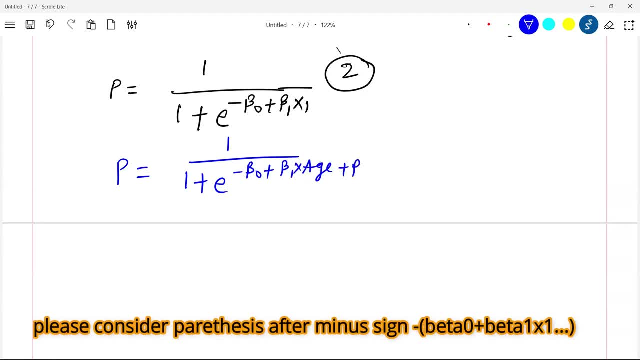 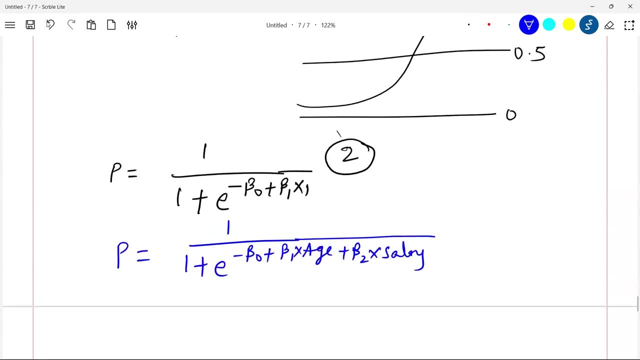 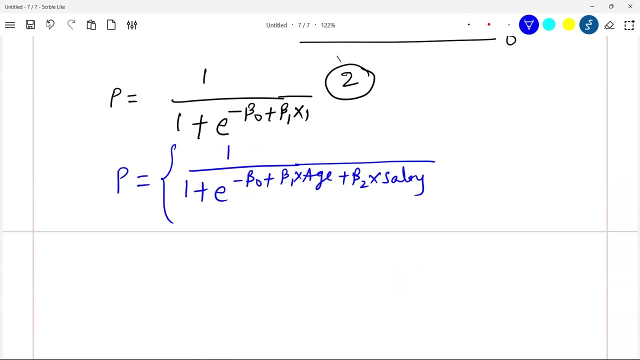 into age, okay, plus beta 2 into salary. this is nothing but your logit equation and this is a logistic regression equation. okay, and as you know, as i told you, this is a sigmoid function, so the output of what you see here, output of this, will always be between 0 to 1, which means you can. 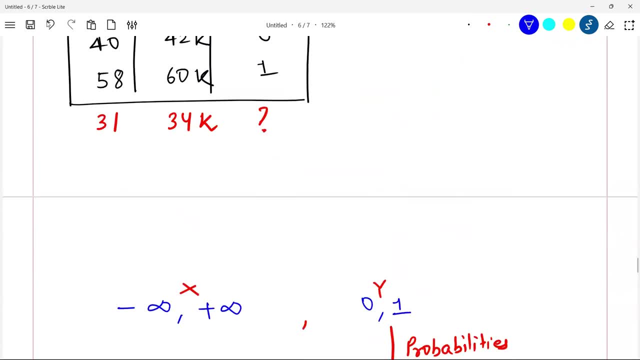 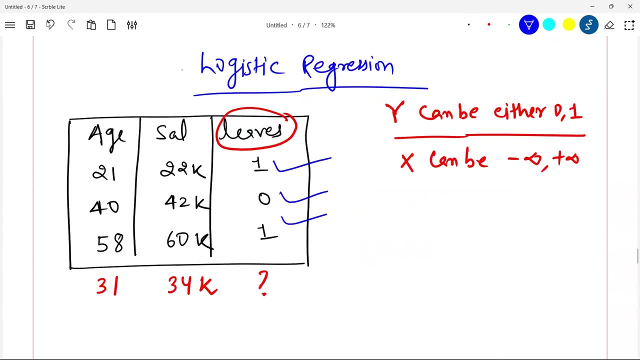 get a probability and then you can say that, based on this probability, i can say whether the employee leaves or does not leave. okay, logistic regression is again a very important and not easy to understand concept. okay, so, as you can see, we are modeling a categorical variable against. 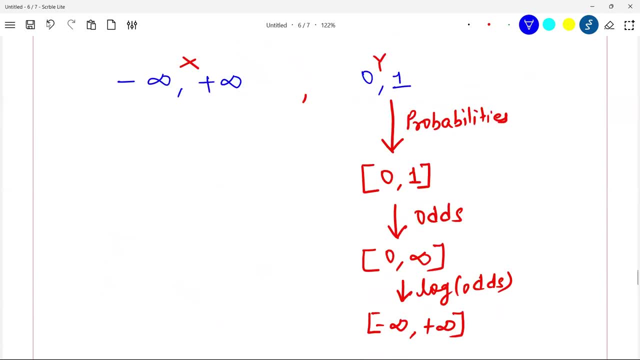 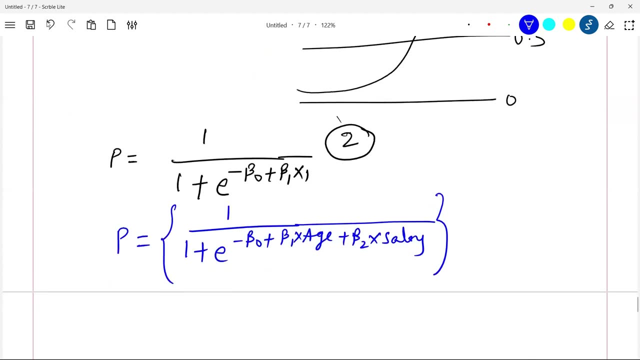 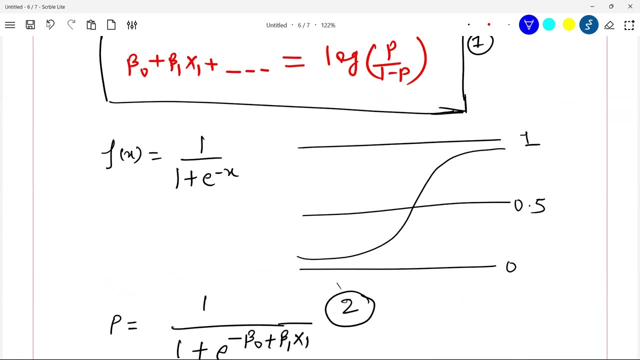 real numbers. hence we need to do certain transformations. these are the transformations that we need to do and how it relates to the probability i just explained you. now, okay, pros and cons: mathematical model, not very difficult to understand. cons: it again assumes a lot of things about the data, which may or may not be correct. hence it may not give a great result all the time. 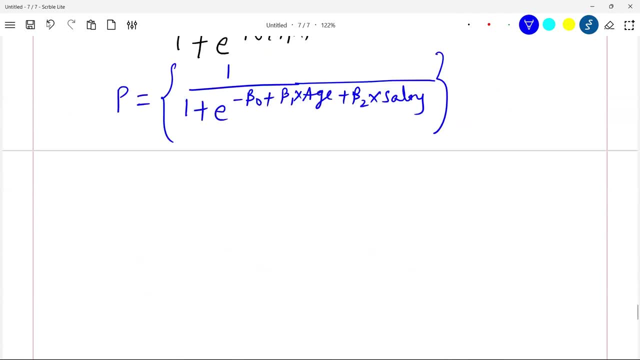 okay, but very famous and very important algorithm to understand. next algorithm in the category, in the classification category, one simple one i want to cover here. that is known as k nearest neighbor. okay, it's a pretty simple algorithm, suppose in the same data, on this data, you want to build a canon. 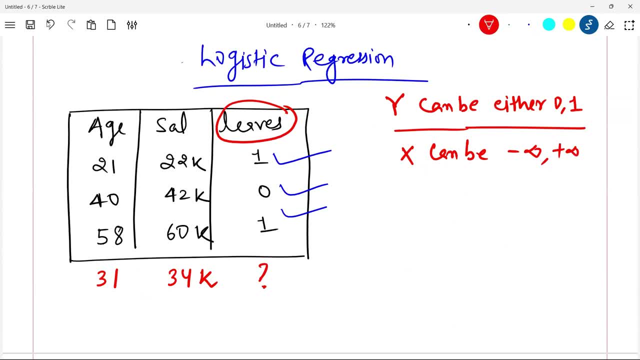 algorithm. okay. so since i have data here, so i will explain here only. so what can happen is it will plot a x-way plane like this: okay, and it's a three-dimensional data, so you can have one more axis for salary or you can have two axis only, because from two axis we can 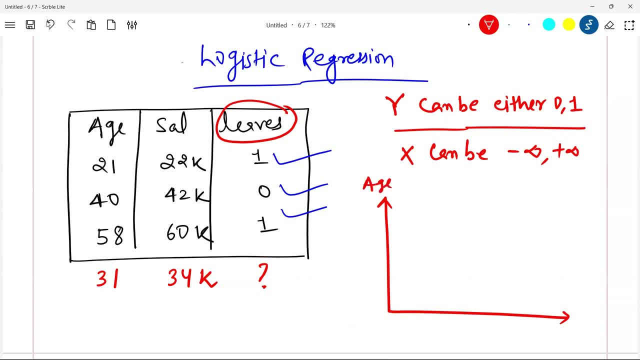 we can predict. okay. so let's come here here age and let's say here, salary. okay, out of these three employees, let's say one employees, 21, 22 employees falls here and second employee, 40 falls here and 58 falls somewhere here. okay, so what k nearest neighbor will do is it will try to allocate neighbors to all these. 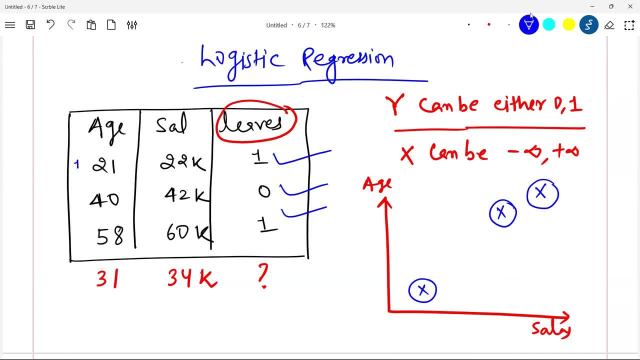 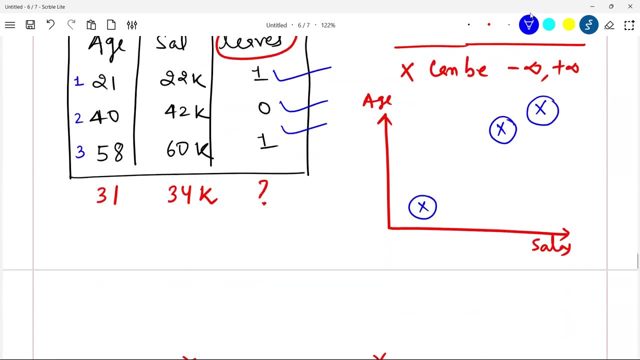 individual observations. for example, this is your observation one, this is your observation two and this is your observation three. okay, so one does not has any neighbors, but two is the neighbor of three and three is the neighbor of two. okay, so tomorrow some prediction comes for, let's say, age 50. again, i will take 50 example. 50 example so. 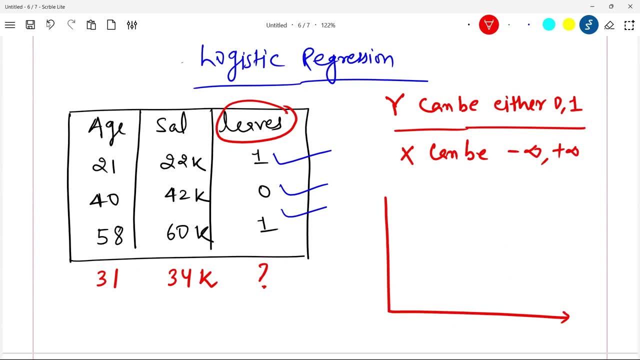 here only. so what can happen is it will plot an x-way plane like this: okay, and it's a three dimensional data, so you can have one more axis for salary, or you can have two axis only because from two axis we can, we can predict, okay. so let's come here, age, and let's say: 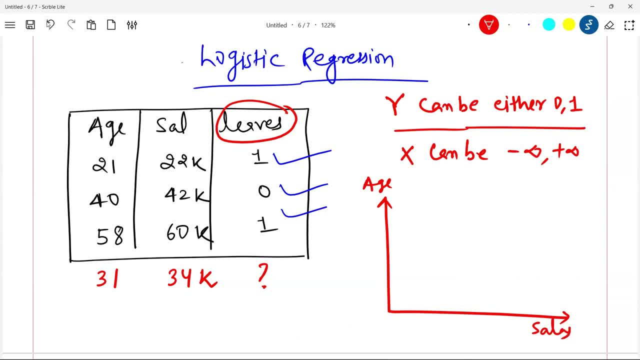 your salary, okay. out of these three employees- let's say one employees, 21, 22 employees falls here, Okay. Let's say, 40 falls here and 58 falls somewhere here, okay. so what Kearney-Arrest-Neighbor will do is it will try to allocate neighbors to all these individual observations. for example, 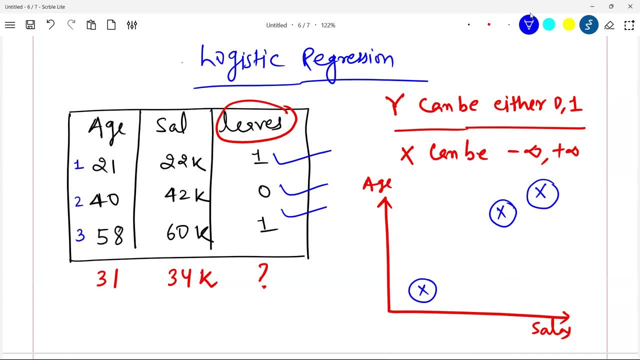 this is your observation one, this is your observation two and this is your observation three. okay, so one does not has any neighbors, but two is the neighbor of three and three is the neighbor of two. okay, so tomorrow some prediction comes for, let's say, age 50 again. 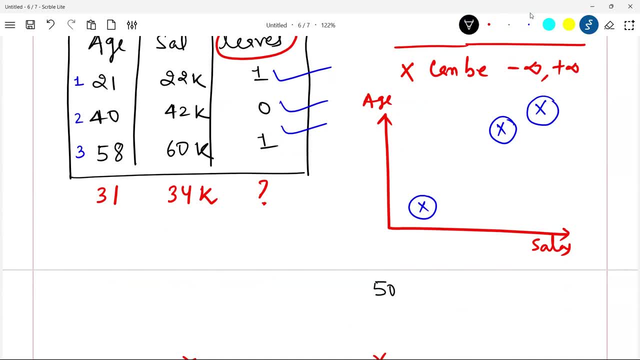 I will take 50 example. So what it will do is it will try to see. and I will take salary also, because in this case salary is also there. so salary is, let's say, 61 K. okay, so what it will do is it will try. 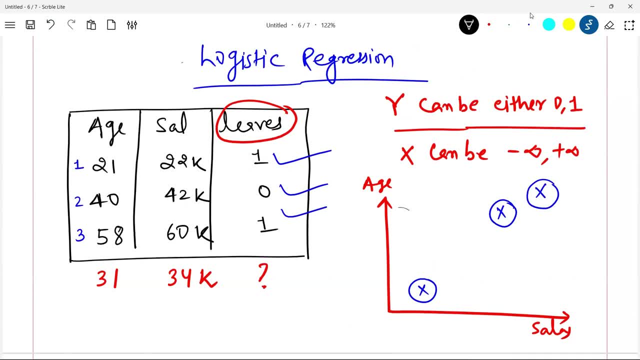 to see where can I fit this 50 age person and salary 61 K maybe who are the nearest neighbor to that guy? so the nearest neighbor to that guy may be this guy and this guy. suppose that new guy comes somewhere here, Okay, So what are the neighbors for this? this is the first neighbor. this is the second neighbor. 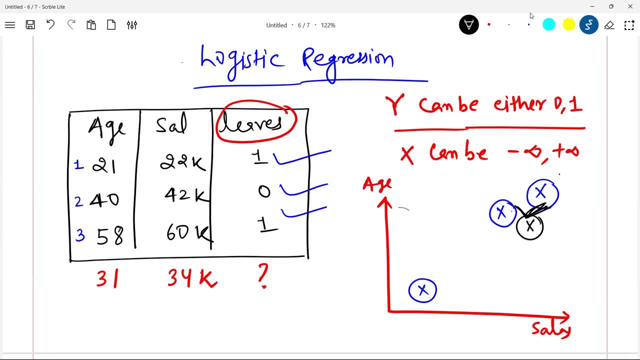 okay, so it will simply go ahead and take the, you know, mode of results. for example, these, these two guys are the. are the second neighbors, right, I mean two neighbors of that? so it will take 0 and 1, which is maximum. so in this case there is no mode of the data, but obviously, 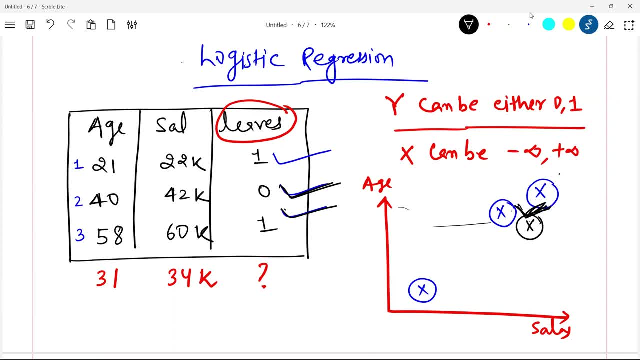 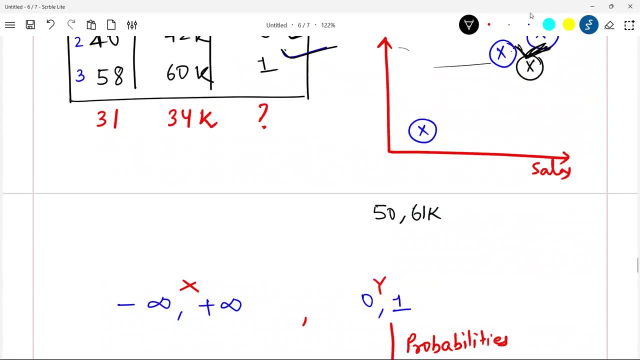 if you take a larger data, there will be modes of the data. okay, so whichever mode- for example, suppose there are 30 record sort of that- 20 is 1 and 10 is 0. so the prediction for this guy will be whatever is maximum or whatever is mode. so if the mode is 1 or 0, whatever. 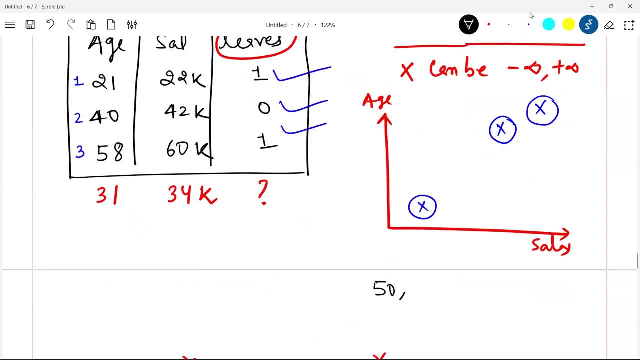 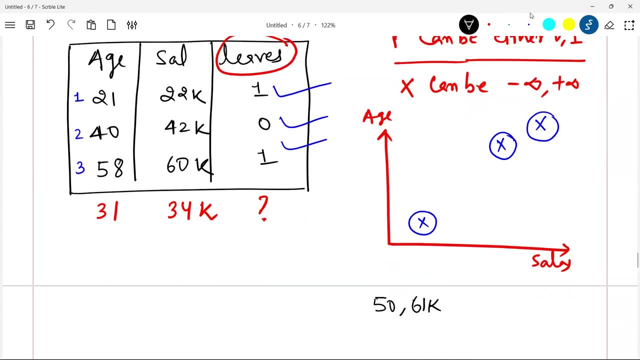 what it will do is it will try to see- and i will take salary also, because in this case salary is also there- so salary is, let's say, 61k, okay. so what it will do is it will try to see. where can i fit this 50 age person and salary 61k? maybe who are the neighbors? 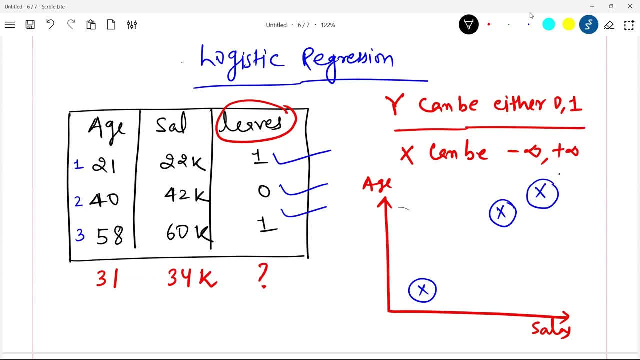 the nearest neighbor to that guy. so the nearest neighbor to that guy may be this guy and this guy- suppose that new guy comes somewhere here? okay, so who are the neighbors for this? this is the first neighbor. this is the second neighbor. okay, so it will simply go ahead and take the. 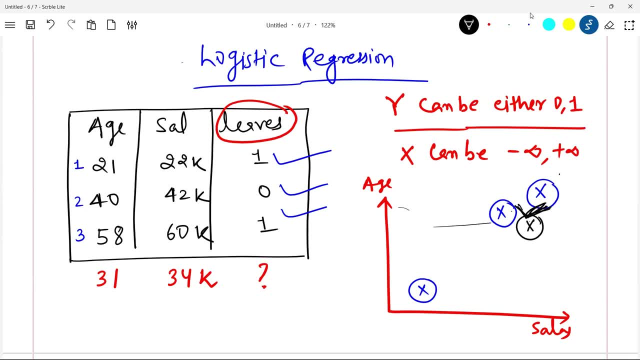 you know, mode of results. for example, these, these two guys are the, are the second neighbors, right, i mean two neighbors of that. so it will take zero and one, which is maximum. so in this case there is no mode of the data, but obviously if you take a level of the data, you can see that there is no data. but obviously if you take a level, 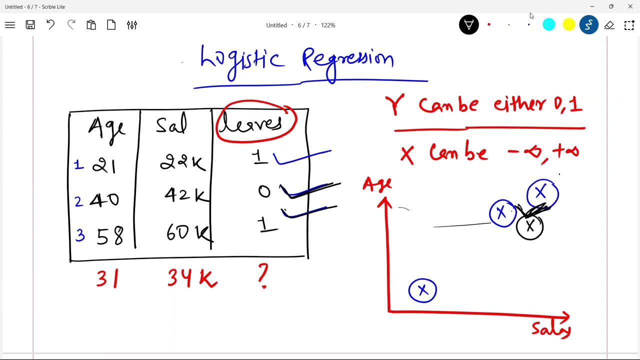 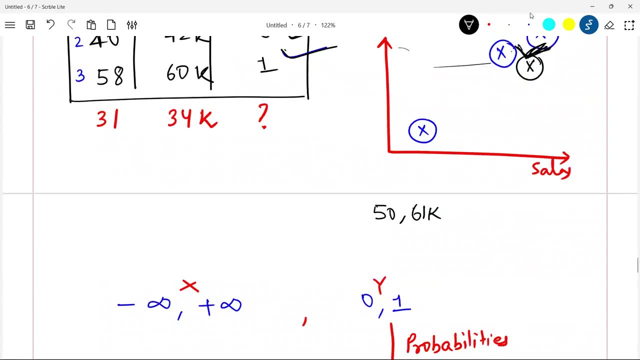 of the data, you can see that there is no data. but obviously if you take a larger data, there will be modes of the data. okay, so whichever mode- for example, suppose there are 30 records out of that, 20 is 1 and 10 is 0. so the prediction for this guy will be: whatever is maximum, or 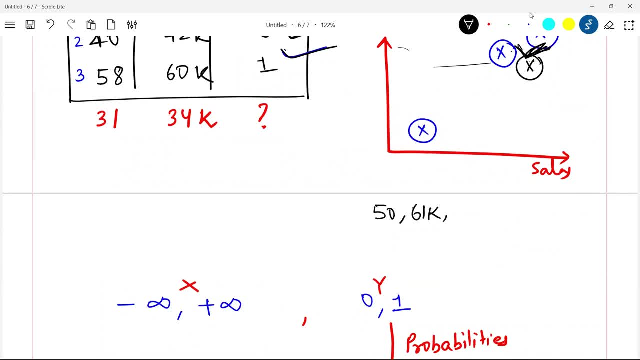 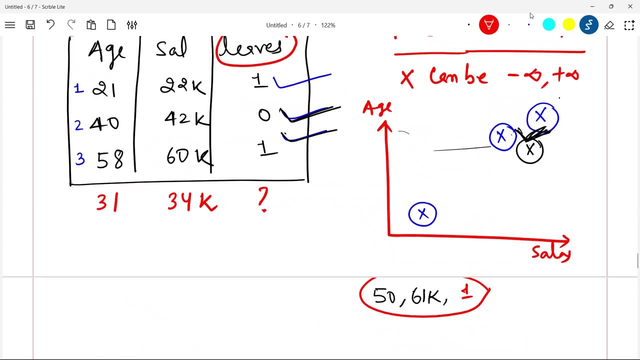 whatever is mode. so if the mode is 1 or 0, whatever it is, that will be the prediction for knn. okay, so, as i told you, canon is a pretty simple algorithm. it will just plot your data, try to find the nearest neighbors and then, when a new observation comes, you give how. 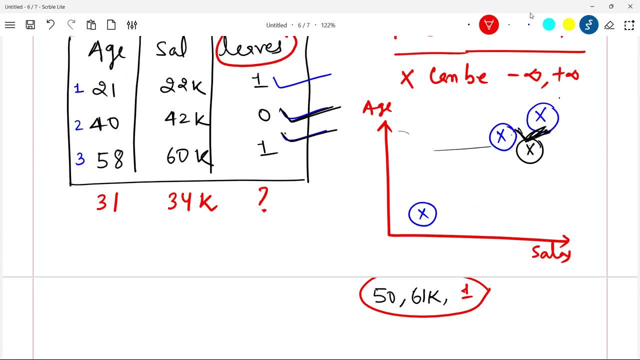 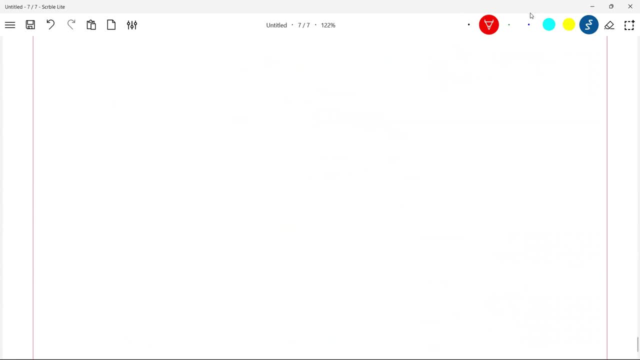 many, how many observation, how many neighbors you want for that record, and it will create on based on that. okay, so canon is a simple to understand algorithm, nothing complex in that, so i covered quickly in that that slide itself. okay, now let's try to understand another classification technique known as support. 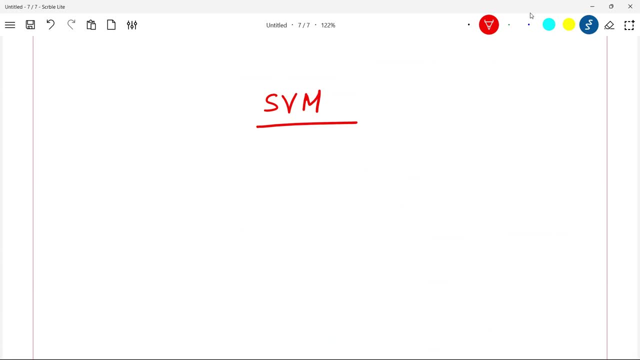 vector machines, or svms. so what svms will do is it will plot your data in whatever axis you have. suppose age is one axis and salary is one axis. okay, and your data points. i will take little more data points. okay, your data points look like this: so these are some data points and this is. these are. 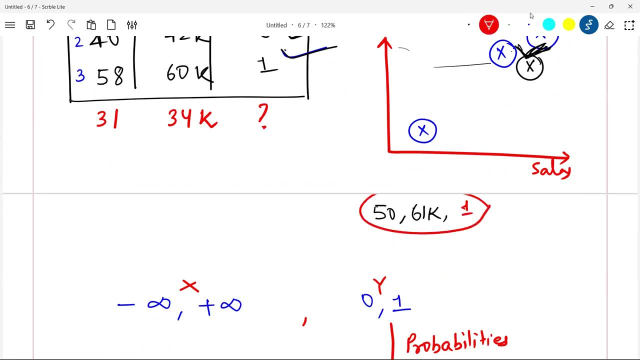 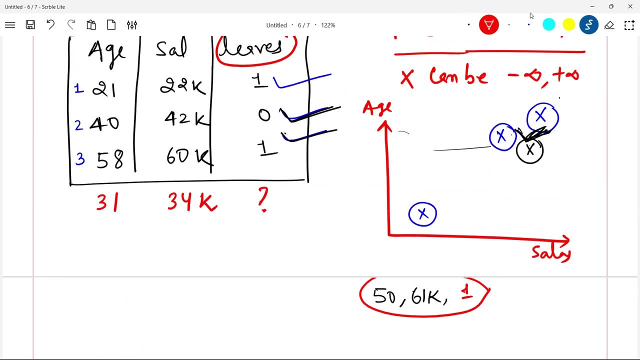 it is. that will be the prediction for KNN. okay, so, as I told you, KNN is a pretty simple algorithm. it will just plot your data, try to find the nearest neighbors and then, when a new observation comes, you give how many, how many of the, how many neighbors you want. 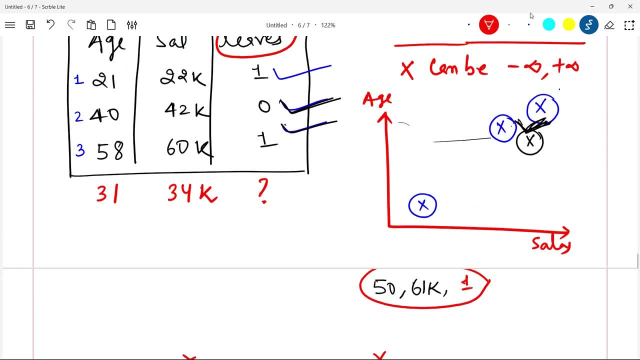 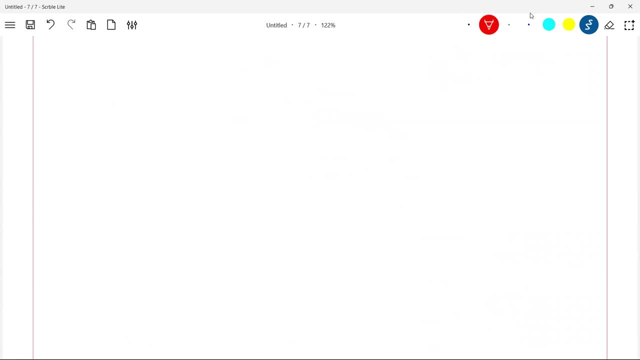 for that record and it will create on based on that. okay, so KNN is a simple to understand algorithm. nothing complex in that, so I covered quickly in that. that slide itself. okay, now let's try to understand another classification technique, known as support vector machines or SVMs. so what SVMs will do is it will plot your data in whatever axis. 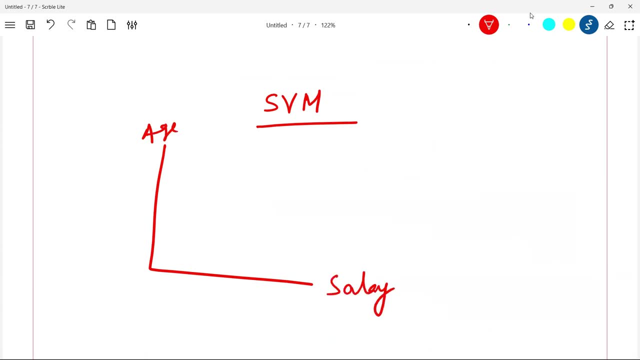 you have. suppose age is one axis and salary is one axis. okay, and your data points? I will take little more data points. okay, your data points look like this: so these are some data points and this is these are some more data points. okay, so what SVM will do is it will try to create something known as a decision boundary. okay, 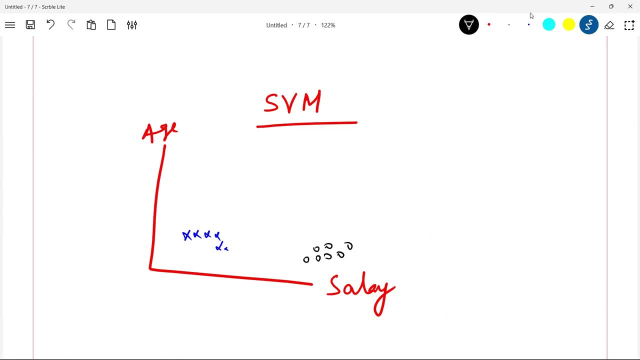 how this decision boundary is different from linear regression. decision boundary is in linear regression. there is a pure mathematical equation involved here. there is a concept of something known as a hyper plane. okay, for example, if I draw a line between this: right, so all these guys- black guys, you can think, leaves or target column is one. all these guys. 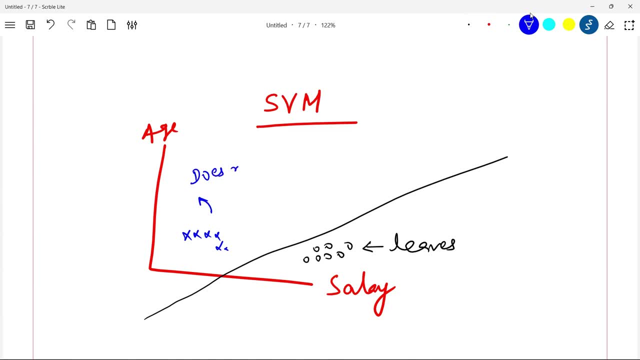 you can think, does not leave, or target column is zero, does not leave. Okay, suppose your data is like this. so what will happen is your SVM will plot. this is called in the language of sbm, this is called decision boundary. okay, decision boundary. so in this case your data looks pretty simple, pretty separated, hence the decision boundary. 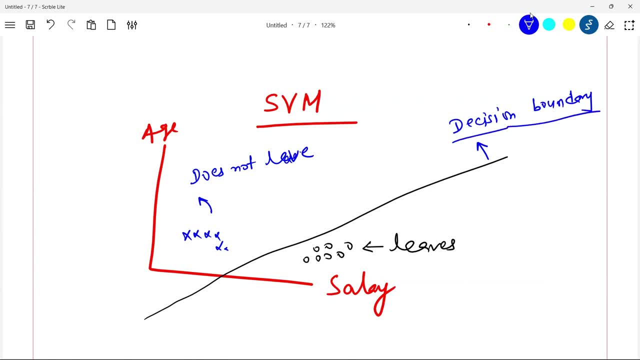 can be as simple as a line- okay, but in most of the scenarios, real world scenarios, decision boundary cannot be as simple as this. okay, So there will be some black dots here, there will be some black circles here, okay, and there can be some- this cross, blue cross, this side, right. so in this case, decision boundary is: 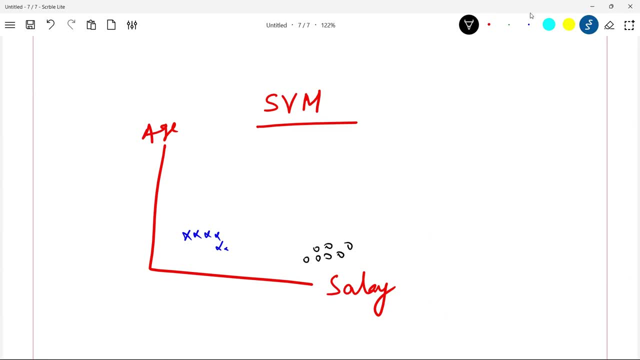 some more data points. okay, so what svm will do is it will try to create something known as a decision boundary. okay, how this decision boundary is different from linear regression. decision boundary is in linear regression. there is a pure mathematical equation involved here. there is a concept of something known as a hyper plane. okay, for example, if i draw 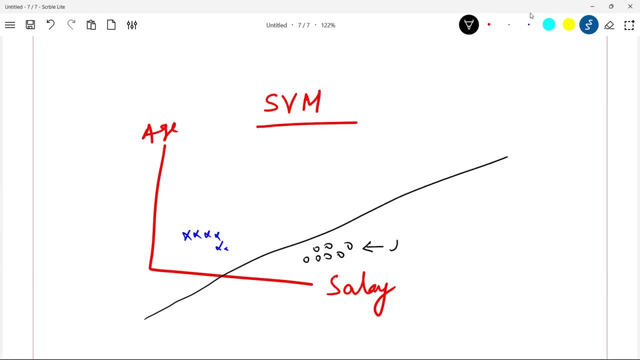 a line between this. right? so all these guys- black guys you can think leaves or target column is one. all these guys you can think does not leave or target column is 0, does not leave. okay, suppose your data is like this. so what will happen is your svm will plot. this is called in the language of svm this: 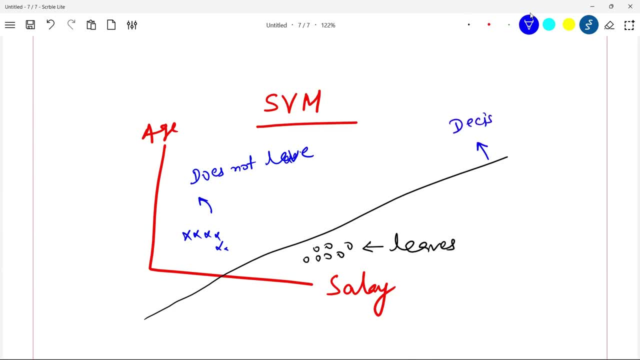 is called a decision boundary. okay, decision boundary. so in this case, your data looks pretty simple, pretty separated, hence the decision boundary can be as simple as such and that's a line. okay. but in most of the scenarios, real world scenarios, decision boundary cannot be as simple as this. okay, so there will be some black dots here, there will be some black circles. 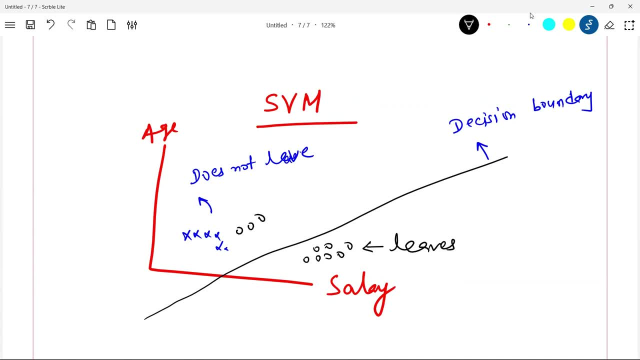 here, okay, and there can be some: this cross, blue cross, this side, right. so in this case, decision boundary is not doing justice. so decision boundary need to change and that is where the concept of hyper planes and kernels, two very important concept in SVM. guys, if you want to explore more on SVM, hyper planes, okay, and kernels so, when your data become, 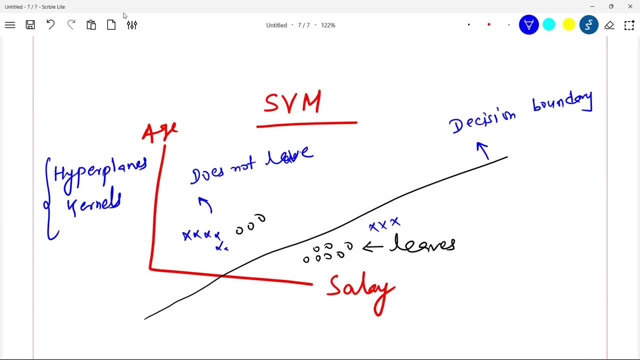 complex, then simple decision boundaries cannot predict it well. okay, so you need to have a have a complex decision boundary, and that is where hyper plane and kernels concepts come. but just to give you an idea of how SVM works, it will create a decision boundary, okay, and tomorrow any prediction, any new result come. for example, somebody asks: what is the? you know. 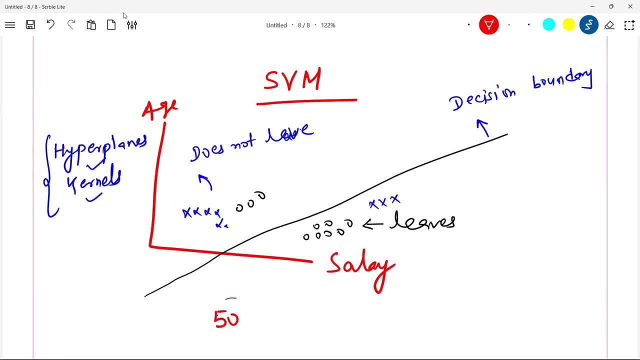 for a person with. for a person with age 50 and salary 60k, whether the person will leave or not leave. so this svm model will see on which side of decision boundary this guy is falling. if this guy falls on this side of decision boundary, it says: do not leave. if this guy falls on this side of 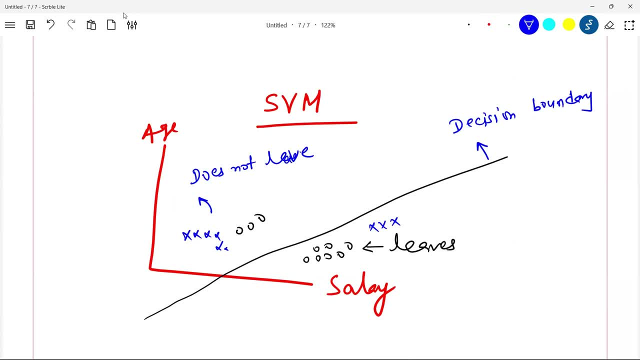 not doing justice. so decision boundary need to change and that is where the concept of hyper planes and kernels- two very important concept in SVM- guys, if you want to explore more on SVM, hyper planes, okay, and kernels. so when your data become complex, then simple decision boundaries cannot predict it well, okay, so you need to have a have a complex. 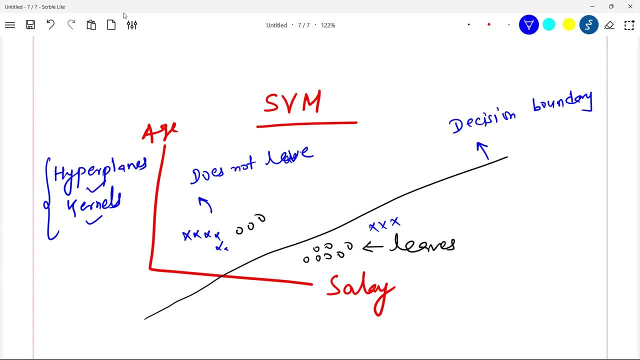 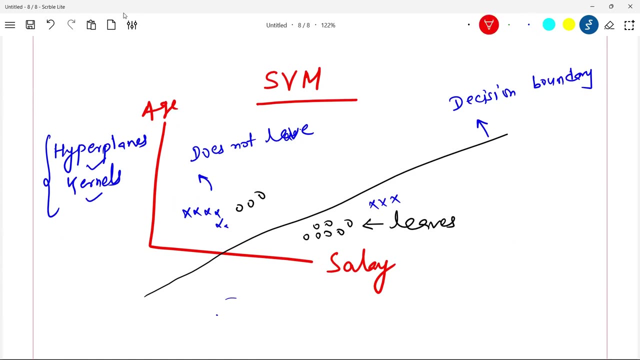 decision boundary and that is where hyper plane and kernels concept come. but just to give you an idea of how SVM works, it will create a decision boundary and tomorrow any prediction, any new result come. for example, somebody asks: what is the you know for a per person with, for a person with age 50 and salary 60k, whether the person will leave or 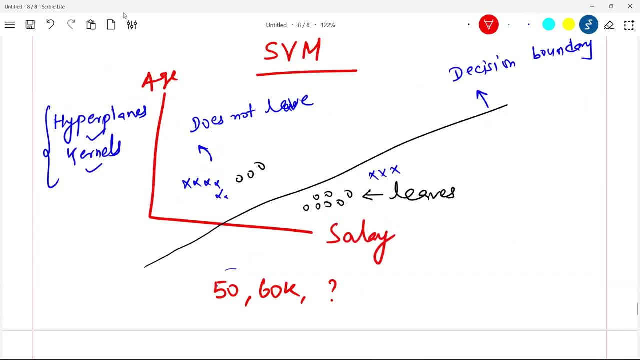 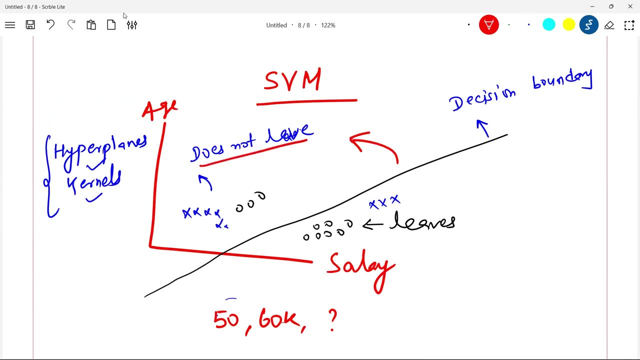 not leave. so this SVM model will see on which side of decision boundary this guy is falling. if this guy falls on this side of decision boundary, it says: do not leave. if this guy falls on this side of decision boundary, it says: leaves. okay. so in SVM, remember concept. 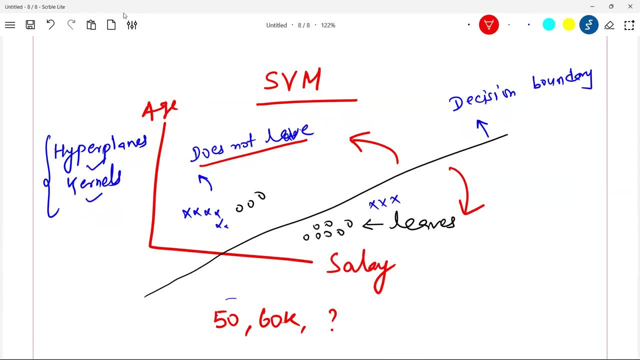 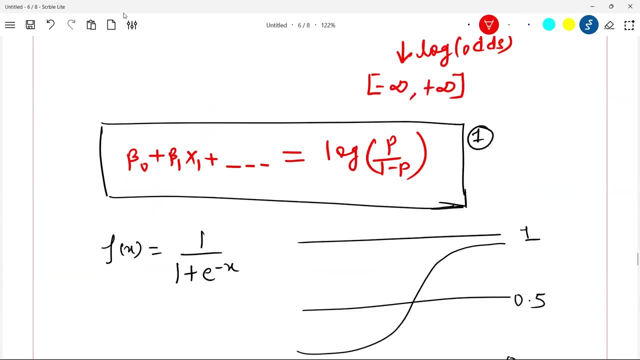 of decision boundaries, hyper planes, kernels and kernel tricks. okay, so we have covered three things from the Classification Scenarios and five things from the regression scenarios. let's go ahead and try to see some unsupervised learning problems. okay, so what is the meaning of unsupervised learning till? 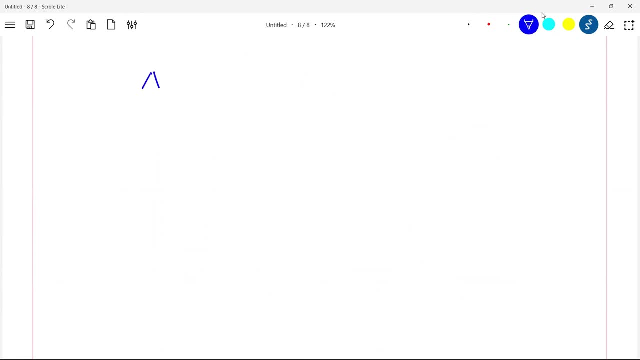 now we are having a target column, but in unsupervised learning we may not have a target column. okay, suppose for the same employee data we have age and salary. but somebody comes to you and tells you that, hey, can you tell me if there are different buckets of employees existing? 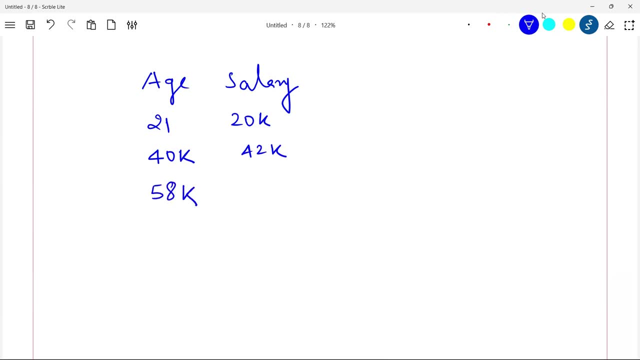 in my organization. Different buckets means some people with less age and more salary, some people with more is and less salary. so are there different buckets? somebody can can come and ask you. okay, so how you will solve that problem is by using something: knowledge clustering or segmentation. okay, so suppose the task in hand is here. there are three records only, but there. 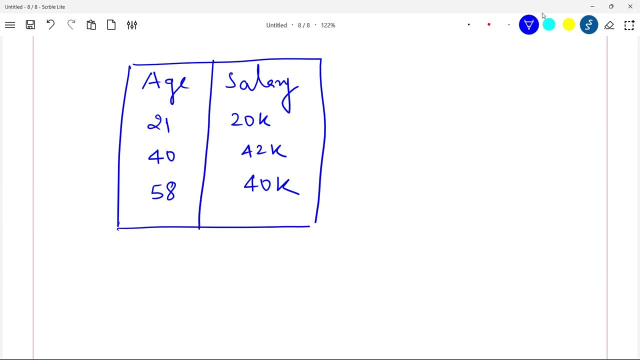 can be more records right in the real world scenario. what I'm interested in knowing is if there are natural clusters in my organization. so this is my organization data on one axis I have is on other axis I have salary okay and I have multiple data points here. three: 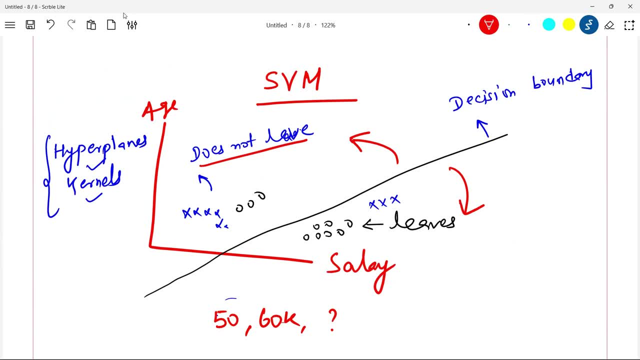 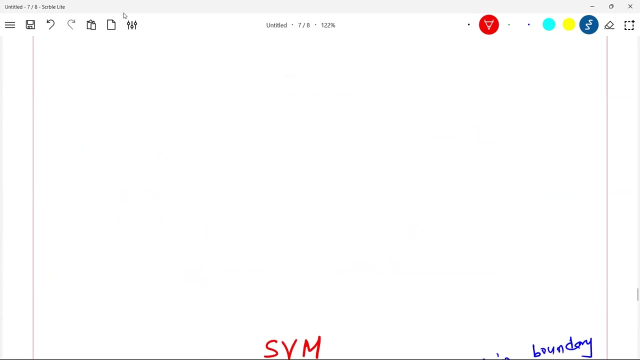 decision boundary, it says leaves. okay. so in svm, remember concept of decision boundaries, hyperplanes, kernels and kernel tricks. okay, so we have covered three things from the classification scenarios and five things from the regression scenarios. let's go ahead and try to see some unsupervised learning problems. okay, so what is the meaning of unsupervised learning? till now, we are having a. 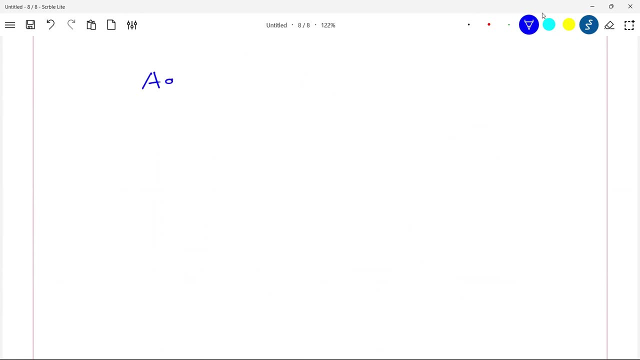 target column. but in unsupervised learning we may not have a target column. okay, suppose for the same employee data we have age and salary. but suppose for the same employee data we have age and salary, but suppose for the same employee data. somebody comes to you and tells you that, hey, can you tell me if there are different buckets of? 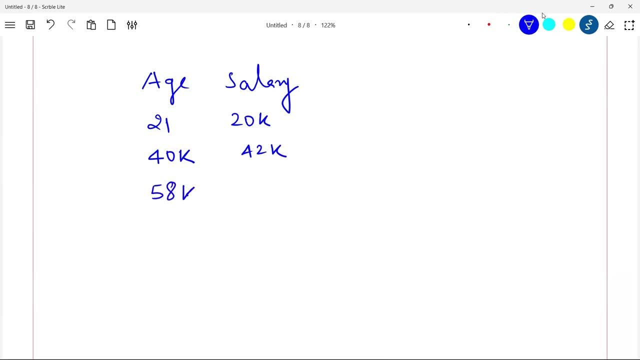 employees existing in my organization. different buckets means some people with less age and more salary, some people with more is and less salary. so are there different buckets? somebody can can come and ask you. okay, so how you really solve that problem is by using something known as clustering or segmentation. okay, so suppose the task in hand is here. there are three records. 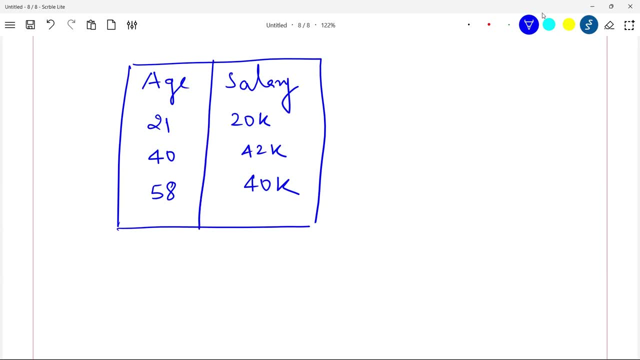 only, but there can be more records right in the real world scenario. what i am interested in knowing is if there are natural clusters in my organization. so this is my organization data on one axis. i have is on other axis. i have salary- okay, and i have multiple data points here. three data points only. 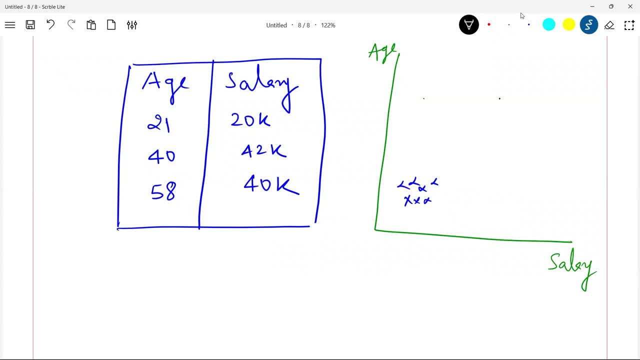 but i am plotting more data points just for demonstration. okay, so there is nothing to predict, but employer is interested in knowing if there are. buckets means if few employees are closer to each other in terms of their characteristics. so, for example, these employees are closer, you can call bucket one, these employees are closer, you can call bucket two. or 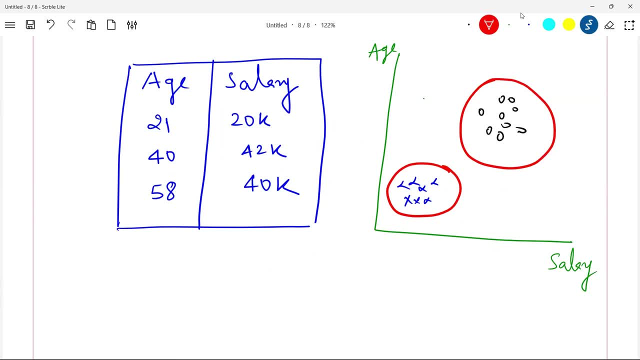 segment two. okay, but how this will be implemented is in: k means clustering. so one technique for implementing bucketing is k means clustering. okay, there can be other techniques also for segmentation or bucketing. one technique is k means clustering. in this technique, what will happen is the distance between the various employees will be. 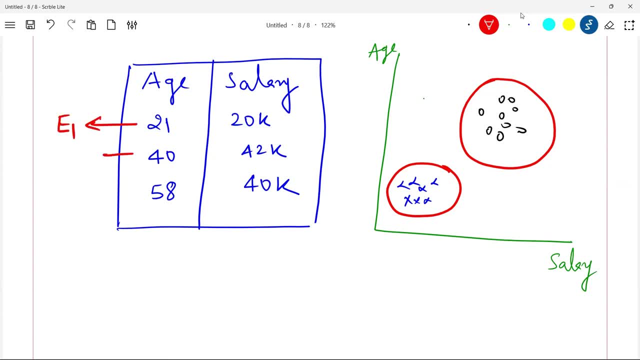 computed. for example, this is your employee one and this is your employee two. okay, suppose i ask you how similar is employee one from employee two? so there can be different similarity metric that you can compute, for example euclidean distance or manhattan distance or cosine similarity etc. 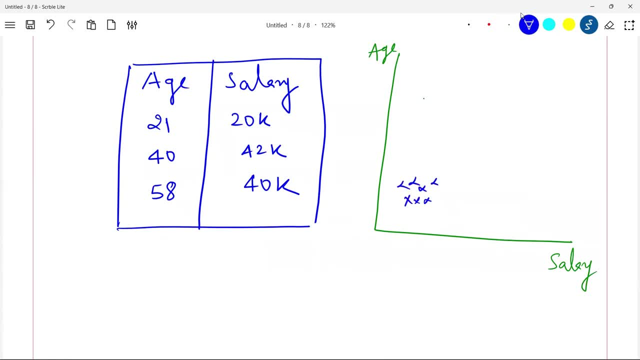 data points only, but I am plotting more data points just for demonstration. okay, so there is nothing to predict, but employer is interested in knowing if there are. buckets means if few employees are closer to each other in terms of their characteristics. so, for example, these employees are closer, you can call buckets. 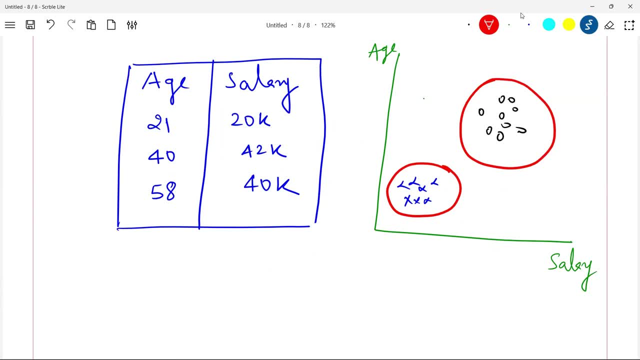 One. these employees are closer. you can call bucket two or segment two, okay, but how this will be implemented is in k-means clustering. so one technique for implementing bucketing is k-means clustering. okay, there can be other techniques also for segmentation or bucketing. one technique is k-means clustering. in this technique, what will happen is the distance. 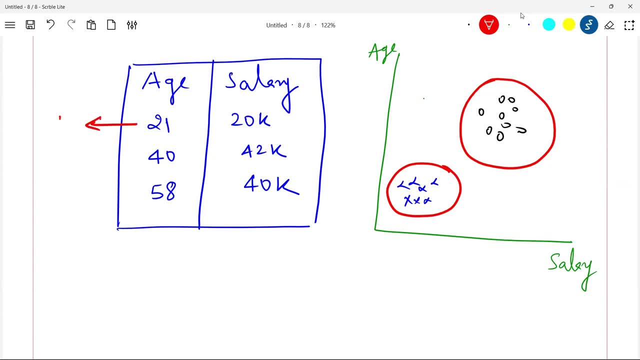 between the various employees will be computed. for example, this is your employee one and this is your employee two. okay, Suppose I ask you how similar is employee one from employee two? so there can be different similarity metric that you can compute, for example Euclidean distance or Manhattan distance. 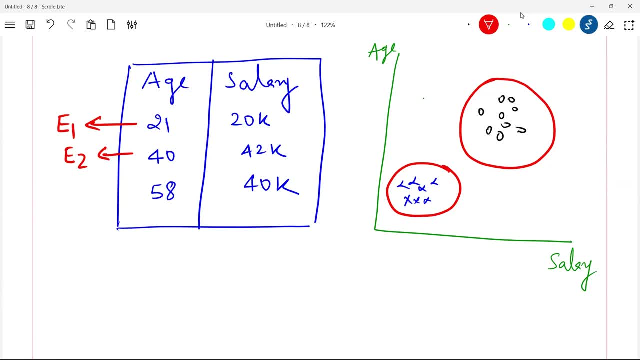 or cosine similarity, etc. I have detailed video on these things as well. I will link it in the description. but suppose I tell you a simple. you know how the distance, how the similar sim, how these two employees are similar or different. so you will say twenty one minus forty whole square plus twenty one. 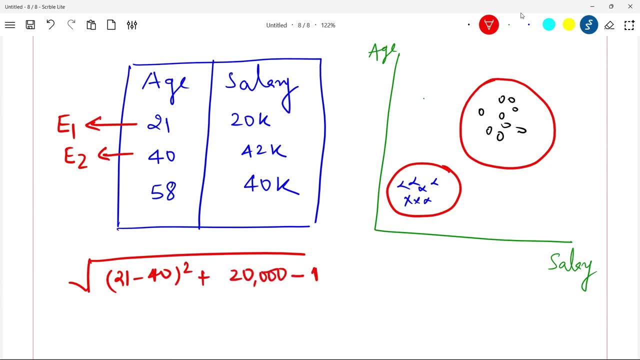 twenty k, twenty k minus forty two k, whole square. so on all the dimensions, you are taking the distance between them, squaring it and under routing it. this is called Euclidean distance between E1 and E2, whatever number you get it, okay. so suppose E1 and E2 Euclidean. 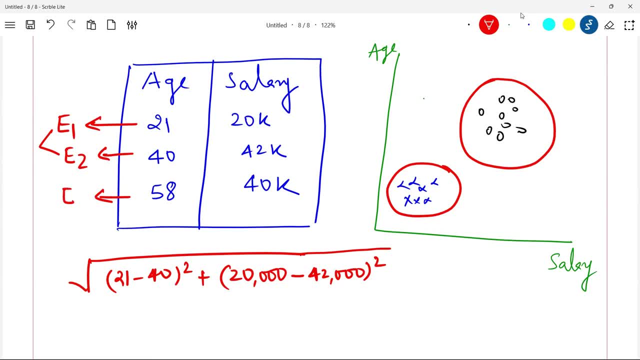 distance is less and E1 and E3 Euclidean distance is more. so in that case you say E1 and E2 are closer to each other. okay, and in the similar way you start finding the employees which are closer to each other And then you call this as one bucket. similarly, this call you call is at an another bucket. 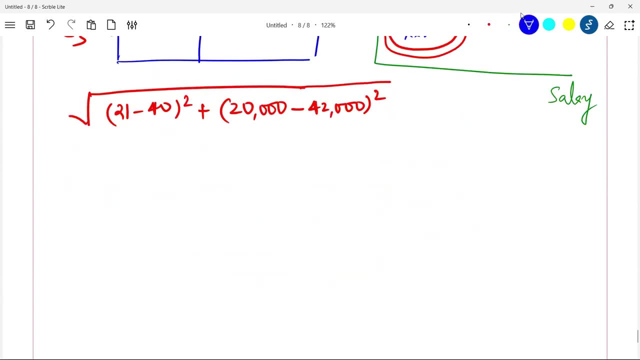 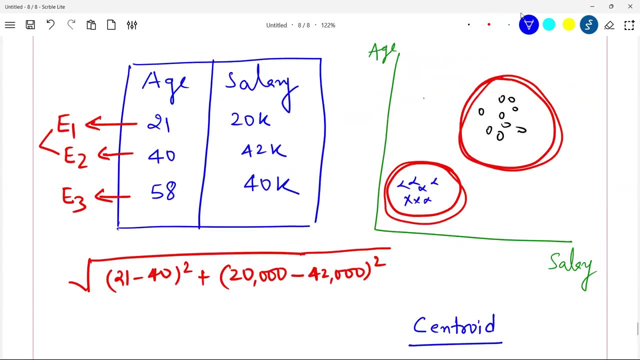 okay, remember, I have explained you in simple terms, but there is a very important concept in k-means, known as centroid concept. okay, so please go ahead and watch unfold data science detailed video on k-means clustering. you will understand all the details of how centroid is defined and how this algorithm works at a mathematical level. okay, I will link that. 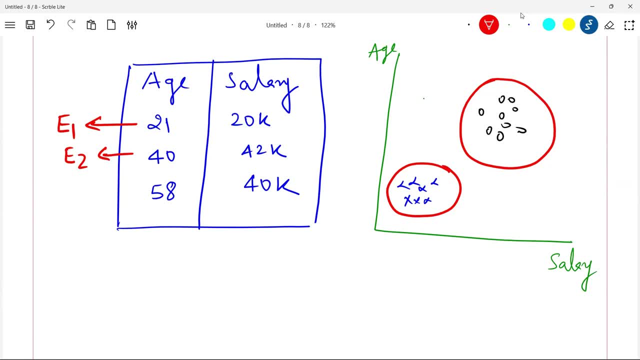 i have detailed video on these things as well. i will link it in the description. but suppose i tell you a simple: uh, you know how the distance, how the similar sim, how these two are different. so you will say 21 minus 40 whole square plus 20 k, 20 k minus 42 k whole square, so on. 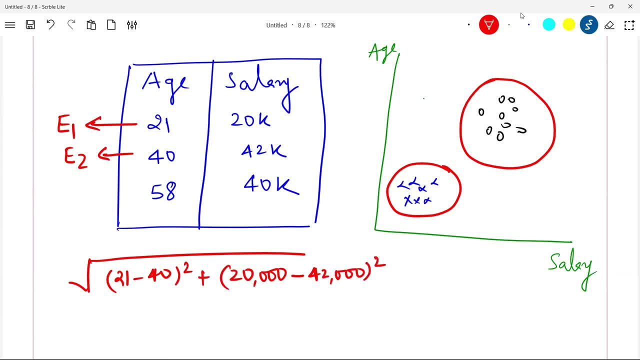 all the dimensions. you are taking the distance between them, squaring it and under rooting it. this is called euclidean distance between e1 and u2, whatever number you get it okay. so suppose e1 and e2 euclidean distance is less and e1 and e3 euclidean distance is more, so in that case you say: 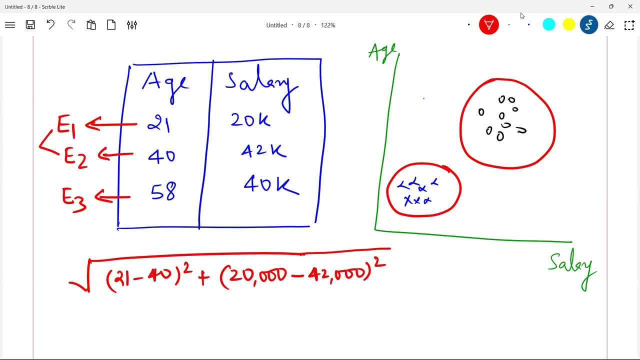 you are taking the distance between them, and you are taking the distance between them. okay. and in the similar way, you start finding the employees which are closer to each other and then you call this as one bucket. similarly, this call you call is at an another bucket- okay. 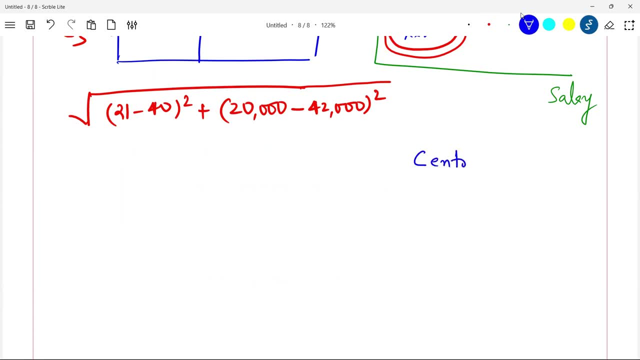 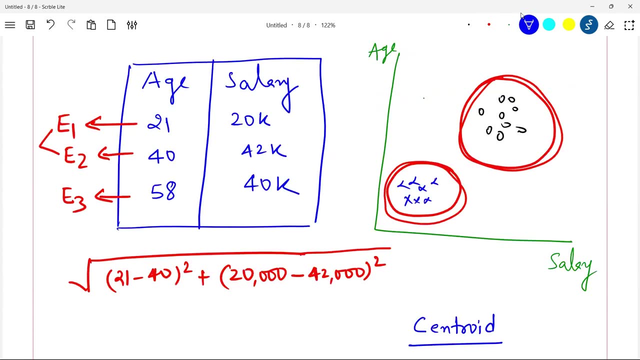 remember i have explained you in simple terms, but there is a very important concept in k-means, known as centroid concept. okay, so please go ahead and watch unfold data science detailed video on k means clustering. you will understand all the details of how centroid is defined and how this. 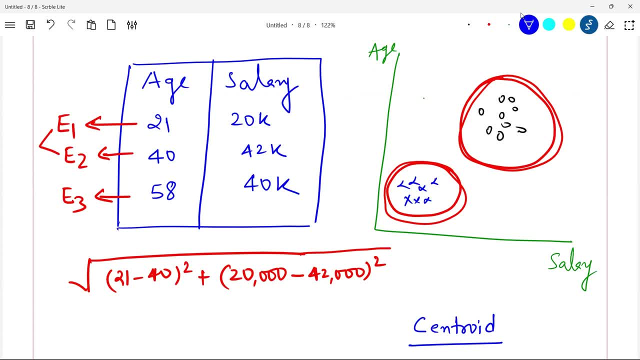 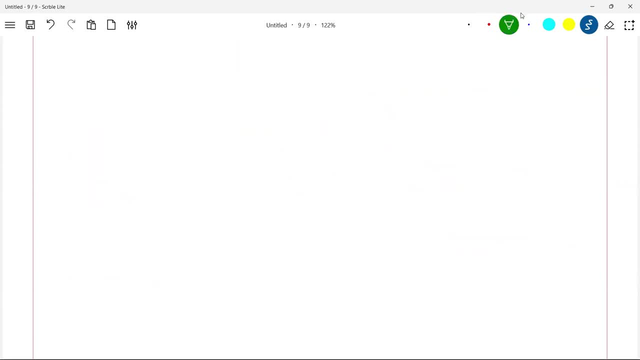 works at a mathematical level. okay, i will link that video. please ensure you watch that. so this is about k-means clustering. now, last but not the least, guys, you might have seen in amazon and flip card that there are different, different uh products. that is recommended to you, for example: 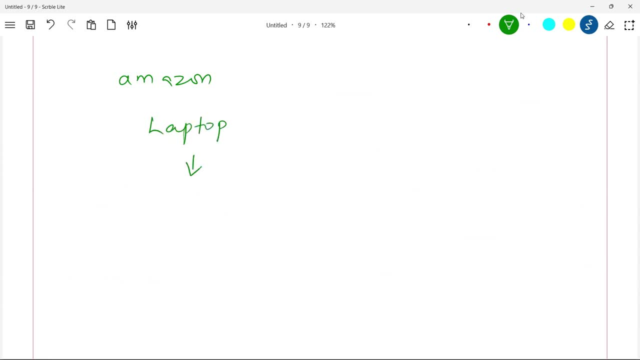 if you buy a laptop, then it will tell you, hey, go ahead and buy this laptop bag as well. so this is nothing but a recommendation. okay, in the netflix, if you watch, let's say, one movie, one actual movie. let's say, if you watch mission impossible, then it will go and recommend you jack ryan series. 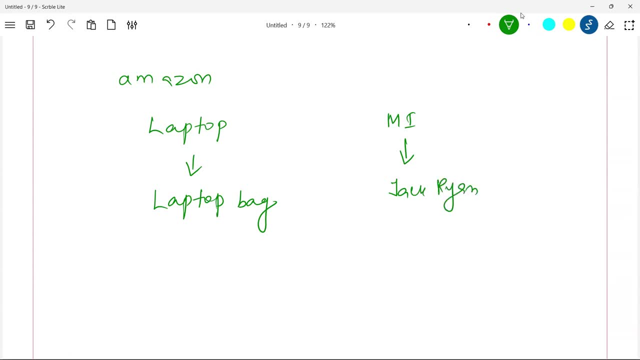 maybe. okay, so this is called a recommendation system that is running in background. okay, so how this system works? one simple, uh, yet powerful technique for recommender system is known as collaborative filtering. collaborative filtering- okay, so what collaborative filtering does is it will take users- okay, users- and it will take items. try to understand this simple concept, guys. it's pretty. 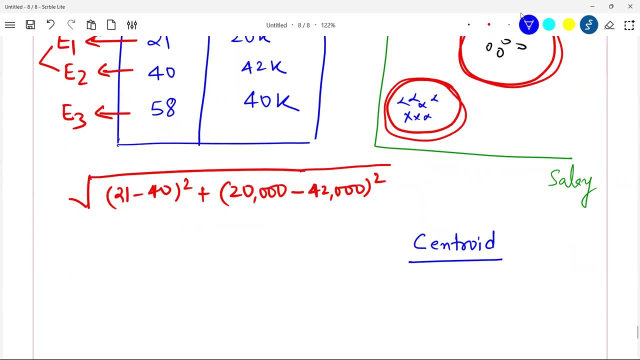 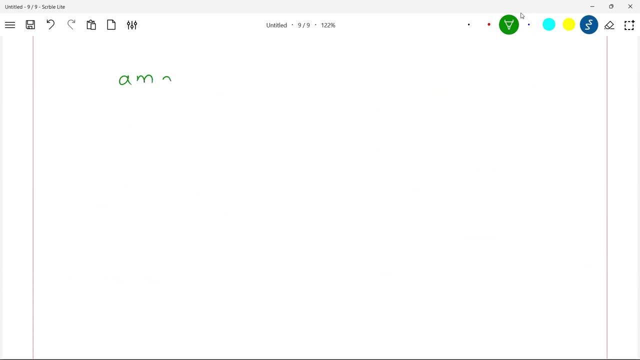 video. please ensure you watch that. So this is about k-means clustering. now, last but not the least, guys, you might have seen in Amazon and flipkart that there are different, different products that is recommended to you. for example, if you buy a laptop, then it will tell you: hey, go ahead and buy this laptop. 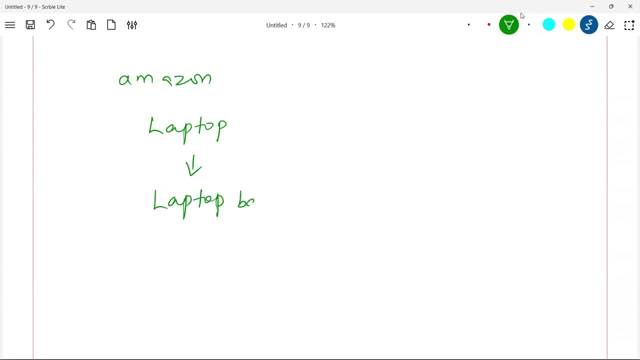 bag as well. so this is nothing but a recommendation. okay, in the Netflix, if you watch, let's say, one movie, one action movie, let's say, if you watch Mission Impossible, then it will go and recommend you Jack Ryan series, maybe. okay, so this is called a recommendation system that is running in. 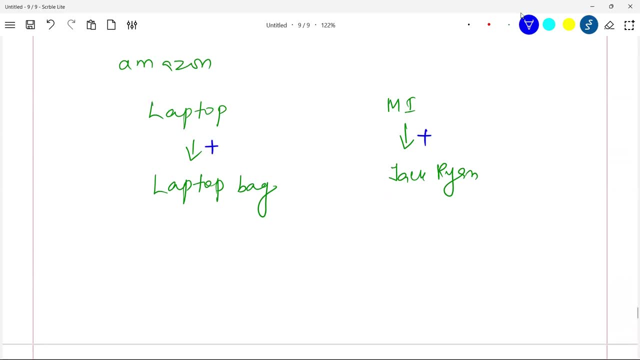 background: okay, so how this system works. one simple yet powerful technique for recommender system is known as collaborative filtering. collaborative filtering- okay. so what collaborative filtering does is it will take users- okay, users- and it will take items. Try to understand this simple concept, guys. it's pretty simple to understand. so users: 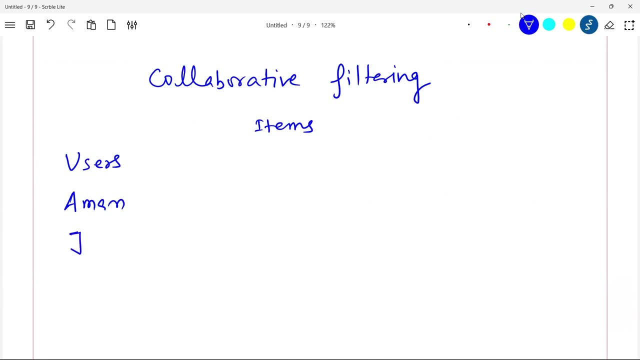 can be Aman and users can be John and users can be Doe, okay. and in the items we can have, let's say, Mission Impossible, in the items we can have Jack Ryan. in the items we can have another any movie of James Bond series. in the items we can have Spiderman, okay in. 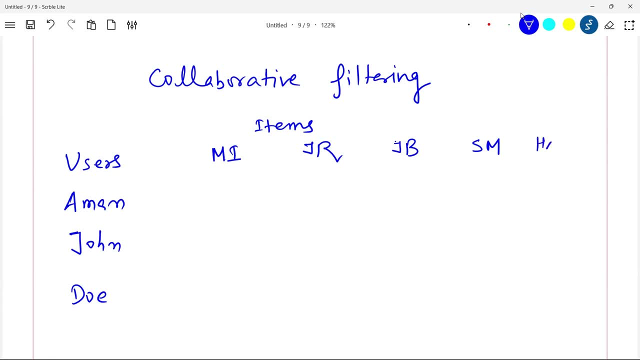 the items. we can have. any comedy movies, for example Home Alone. You can say, Okay, so Aman, which movie Aman watches? or which movie Aman has watched, for example, Mission Impossible. Aman has watched Jack Ryan, he has watched, but he has not watched. let's say this. 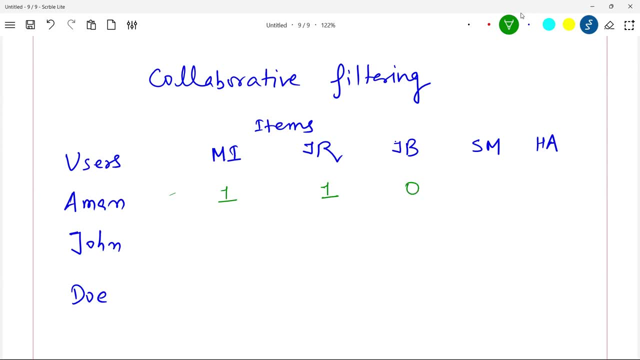 movie. zero. I will say: okay, James Bond movie, and this movie he has not not watched. okay, Spiderman movie. there is another guy, John, who has watched Mission Impossible, Jack Ryan, James Bond movie and Spiderman movie as well. There is another guy, Doe, who has not watched any of these movies but has watched Home Alone. 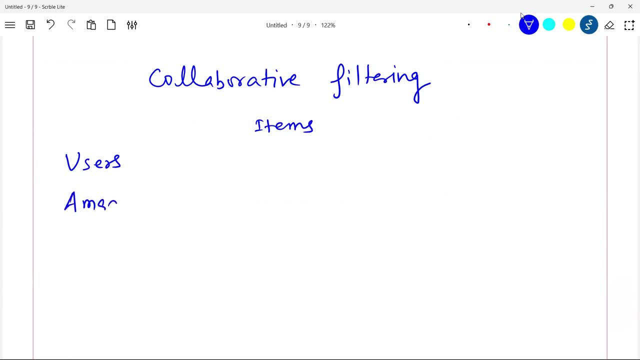 simple to understand. so users can be aman and users can be john and users can be do okay. and in the items we can have, let's say, mission impossible. in the items we can have jack ryan. in the items we can have another, any movie of james bond series. in the items we can have 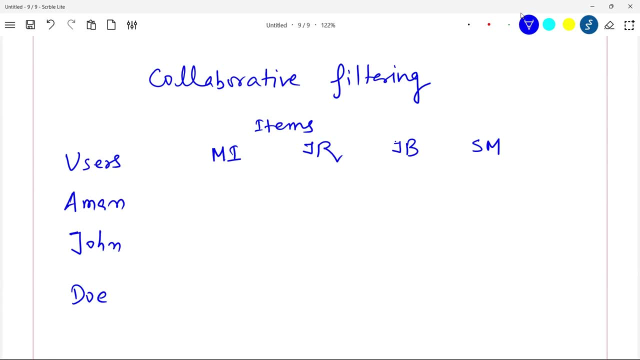 spiderman. okay, in the items we can have any comedy movies, for example home alone. you can say: okay, so aman, which movie aman watches? or which movie aman has watched, for example, mission impossible. aman has washed jack ryan. he has washed, but he has not washed. let's say this movie zero. i. 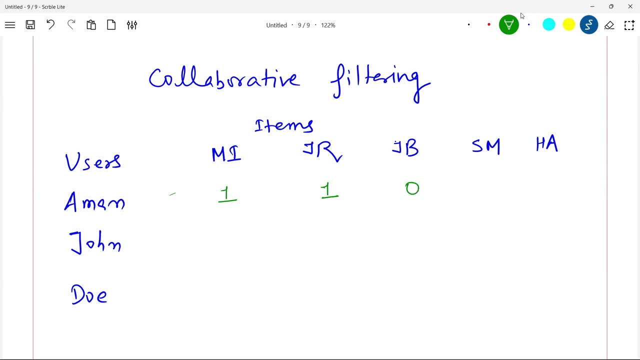 will say, okay, james bond movie and this movie he has not not uh watched. okay, spiderman movie. there is another guy, john, who has watched mission impossible, jack ryan, james bond movie and spiderman movie as well. there is another guy, doe, who has not watched any of these movies but has watched uh, home alone the comedy movie. okay, 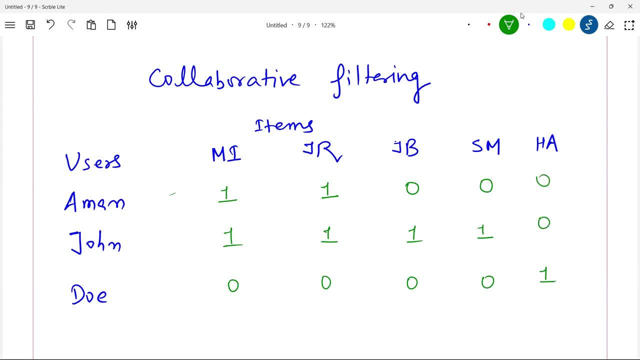 so the which users are similar to which user will be computed based on one of the user similarity metric. so what are the user similarity metric? i told you cosine similarity- it can be different kind of distance metric, so- and the other to which users are meetings, long distance matrix as well as rangezil distance metering. so that's a similar thing. so now let's put so. 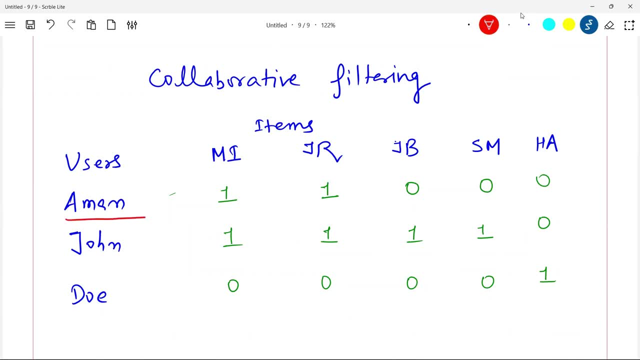 you can think from the common sense also here. Aman watches action movies, if you can see here, and John also watches action movies more. okay, Aman has watched Mission Impossible and Jack Ryan, but Aman has not watched James Wan movie and Aman has not watched Spider-Man movie. 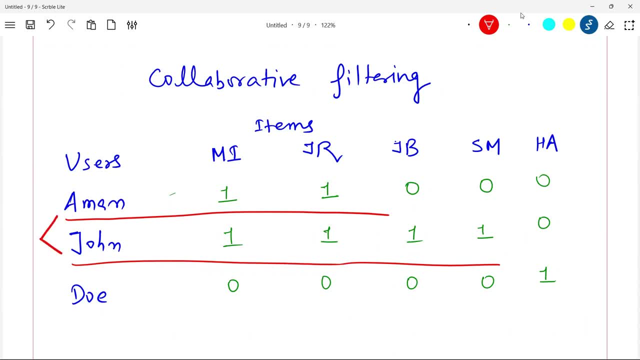 so what will happen is, since Aman and John are similar to each other, so go ahead and watch the movies that John has watched, but Aman has not watched, because Aman and John both tastes are similar- so go ahead and recommend what John has watched, but Aman has not watched. so what will be? 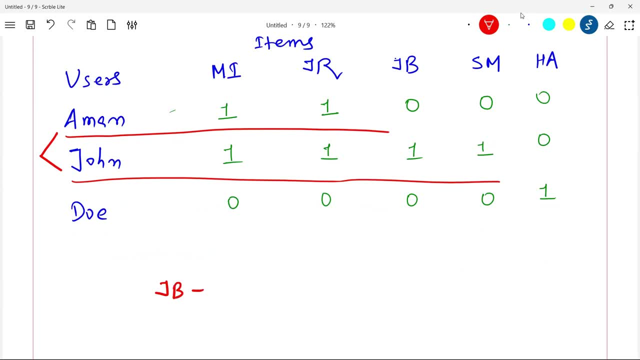 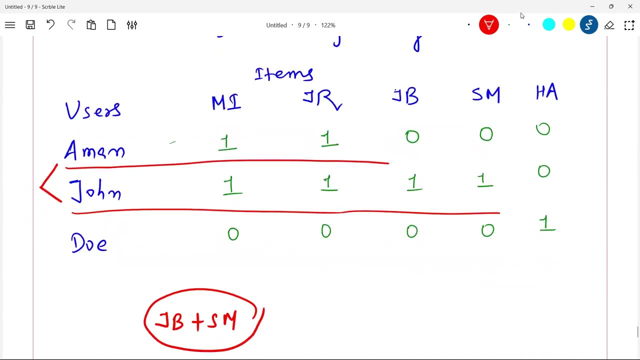 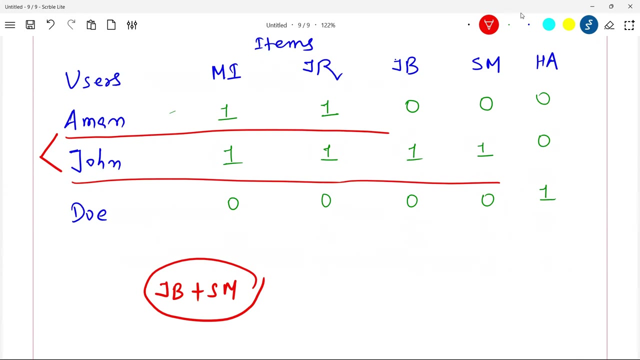 the recommendation going to Aman James Wan movie and Spider-Man movie. okay, now imagine this is a large metric of large users and large items, so it will be seen which users tastes are similar to each other. okay, and then the other user which has not watched that movie will be recommended. the movies or series based on: 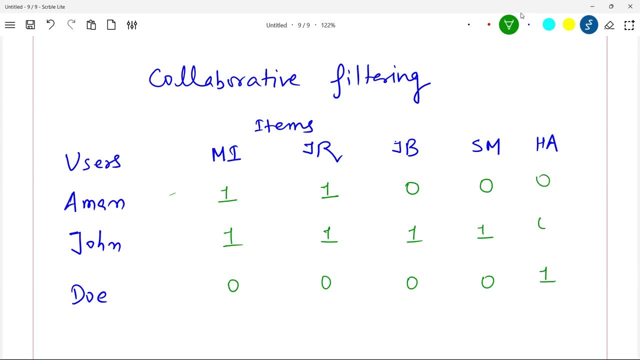 the comedy movie. okay, so the which users are similar to which user will be computed based on one of the user similarity metric. So what are the user similarity metric? I told you cosine similarity, it can be different kind of distance metric. so, as you can think from the common sense, also here, Aman watches. 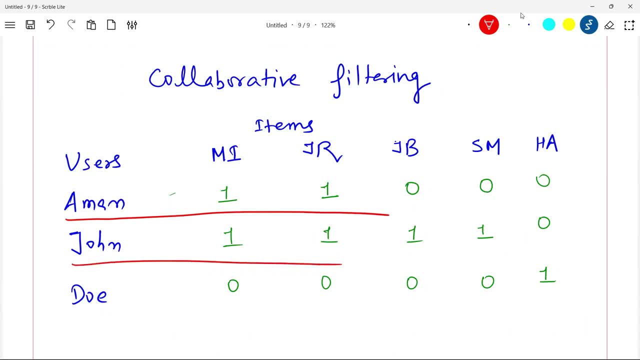 action movies You can see here, and John also watches action movies more. okay, Aman has watched Mission Impossible and Jack Ryan, but Aman has not watched James Bond movie and Aman has not watched Spiderman movie. So what will happen is, since Aman and John are similar to each other, so go ahead and 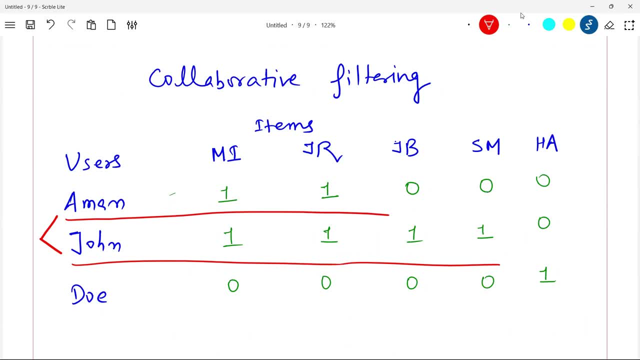 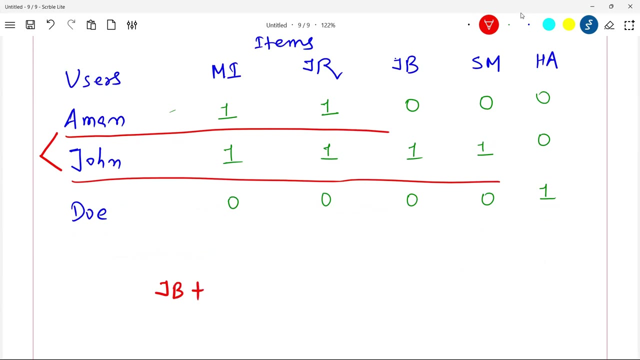 watch the movies that John has watched but Aman has not watched. because Aman and John both tastes are similar. So go ahead and recommend What John has watched but Aman has not watched. So what will be the recommendation going to Aman? James Bond movie and Spiderman movie. 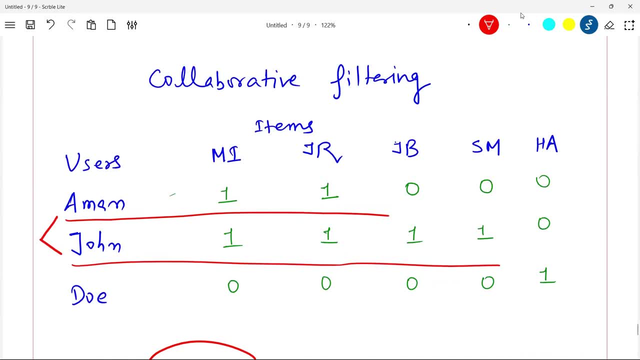 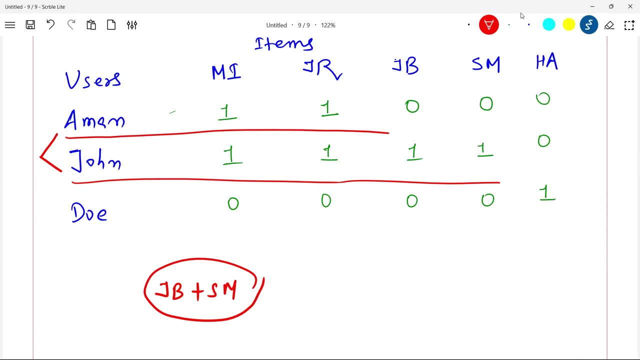 okay, now imagine this is a large metric of large users and large items, So it will be seen which users tastes are similar to each other. okay, and then the other user which has not watched that movie will be recommended: the movies or series based on the similar users watching history. 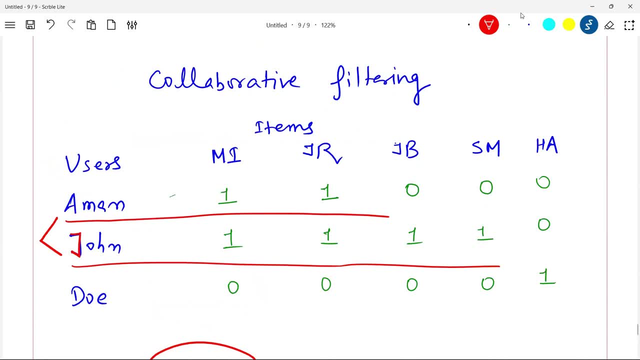 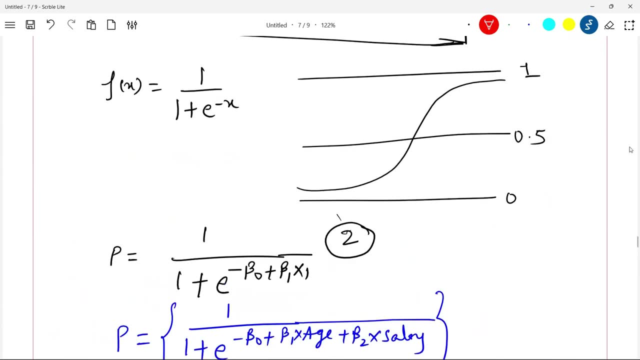 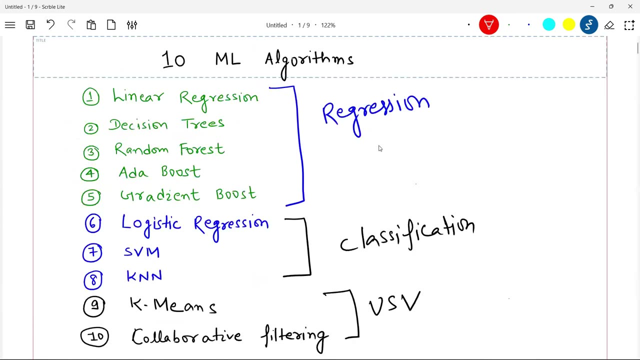 Okay, This is pretty simple but powerful technique known as collaborative filtering. So let's revise once, guys, what all we discussed. long discussion, but very, very fruitful for you to revise. few fundamental concepts: linear regression, decision tree, random for a strata boost, gradient boost for regression. we discussed classification. I explained you logistic regression. 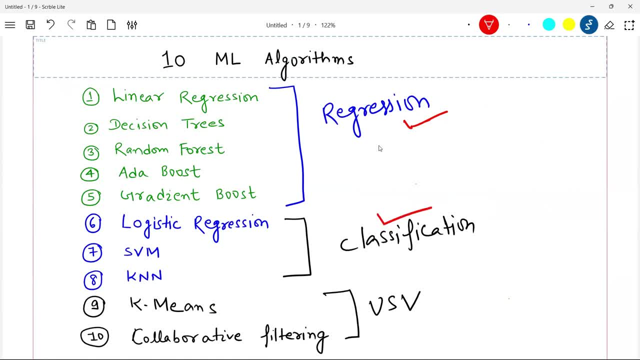 how SVM works and how Canon works, and I explained you to unsupervised technique, K-means and collaborative filtering. Now not in too much detail. I went because it's not possible to go in all the details of 10 algorithms in short time. but treat this as a refresher and please go ahead and click all the links of whichever. 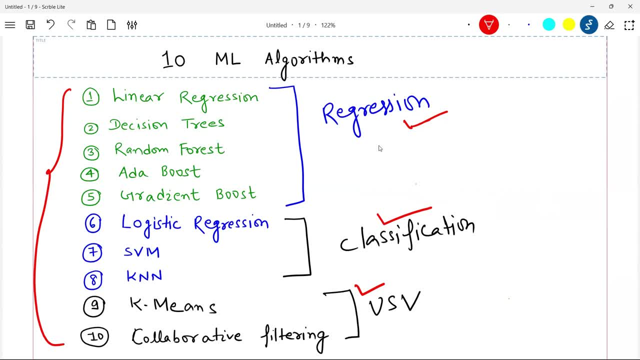 algorithm. you are more interested in learning. all the videos are there on all for data science. Okay, I request you guys, please press the like button if you like this video and please press the subscribe button and the bell icon if you want me to create more videos like this. see. 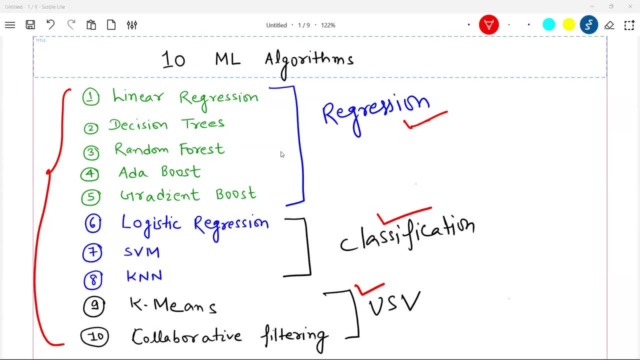 you all in the next video. guys, wherever you are, stay safe and take care. Bye, bye.